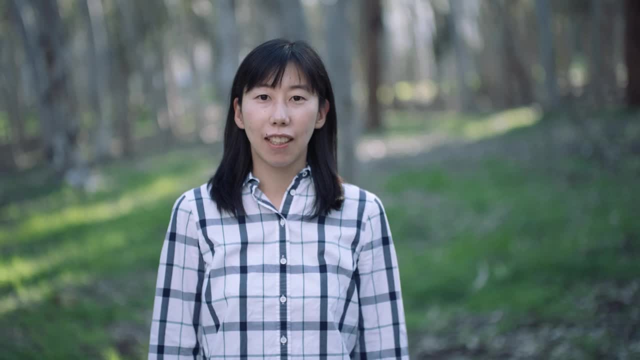 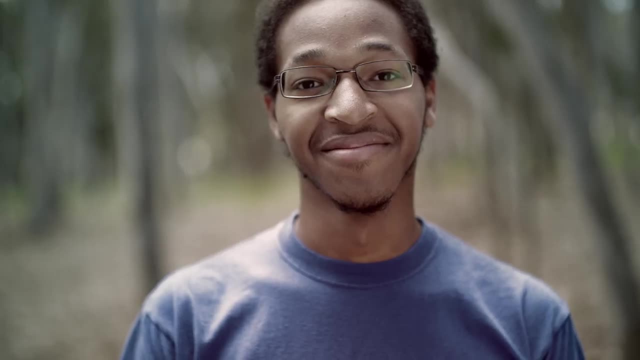 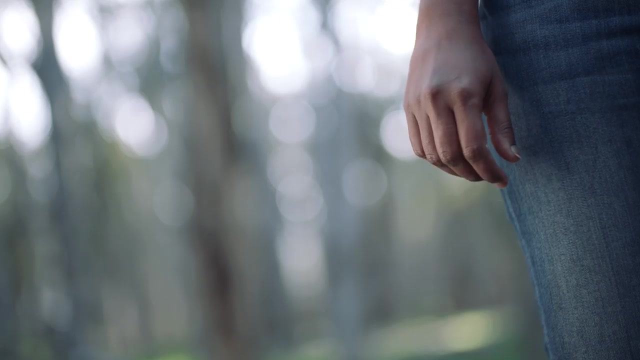 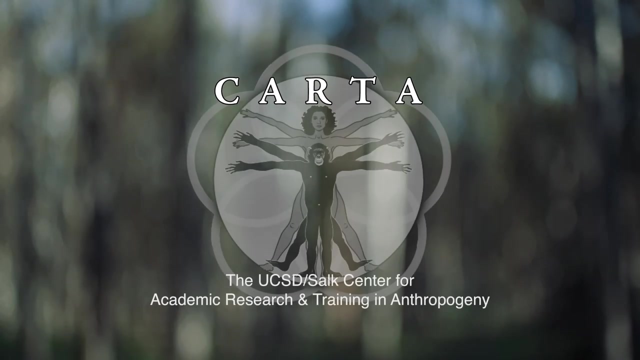 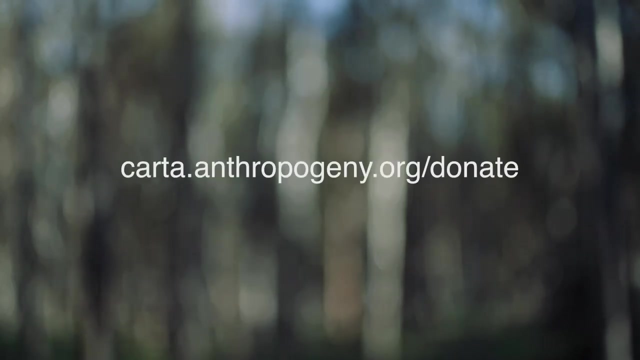 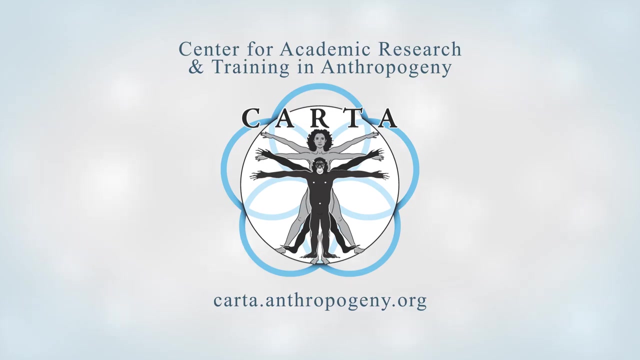 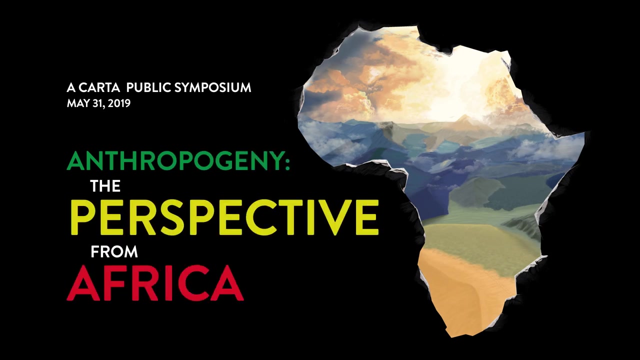 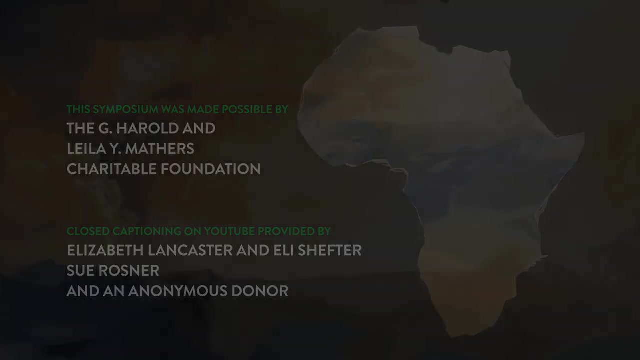 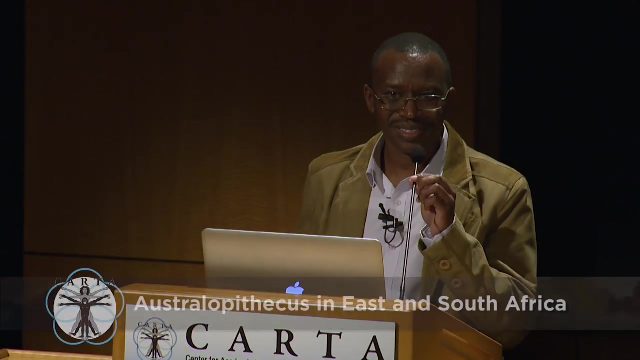 We shape the future from our shared understanding of the past. CARTA brings together experts from diverse disciplines to exchange insights on who we are and how we got here, An exploration made possible by the generosity of humans like you. Good afternoon. I would like to start with acknowledgments, just in case I run out of 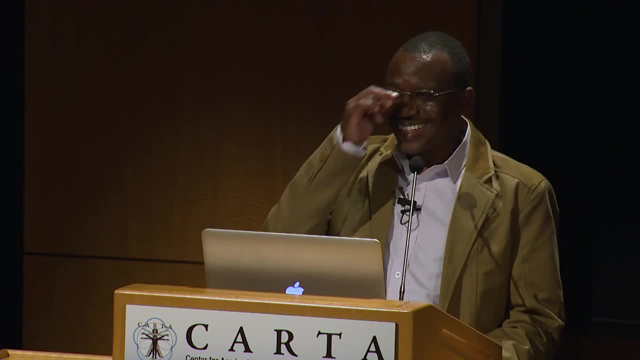 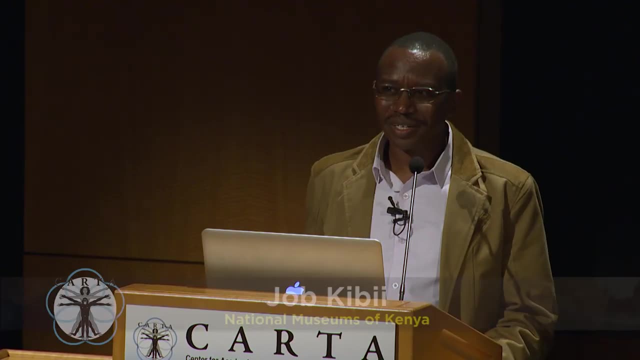 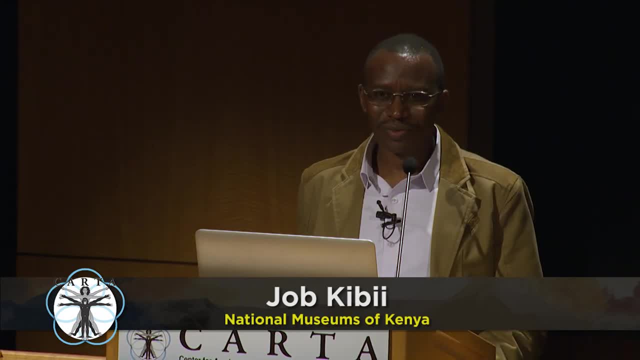 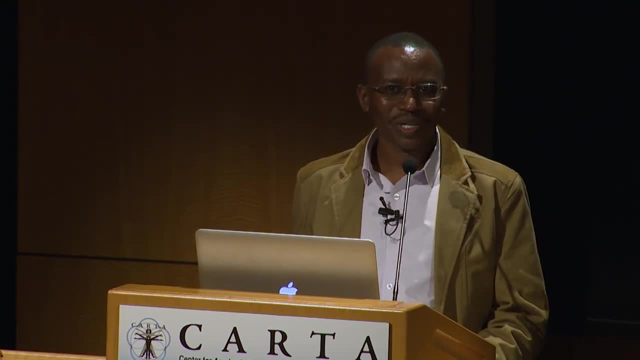 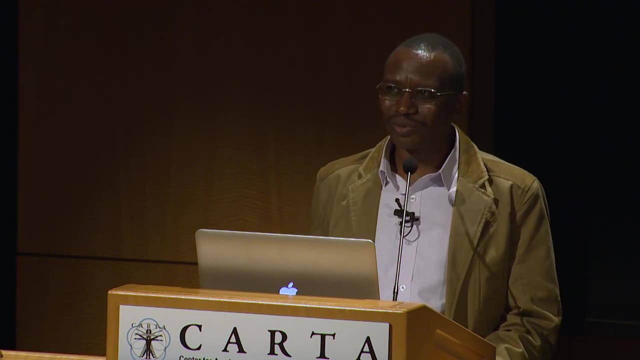 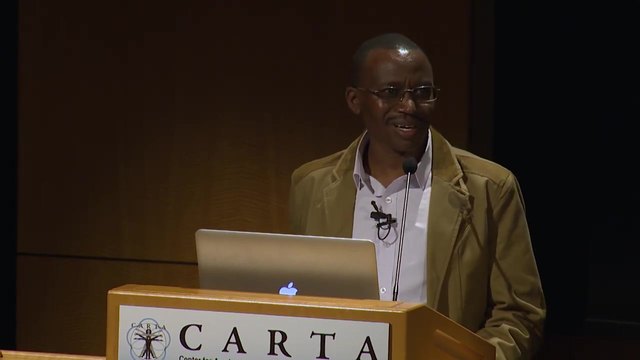 And thank you to the organizers, Bahani, Asfa and Lynn Woodley, and also to Linda- I think we have been communicating a lot with Linda- and also to the general staff of CARTA for making this trip and this symposium a success. I'm saying a success because I think it will be a success. 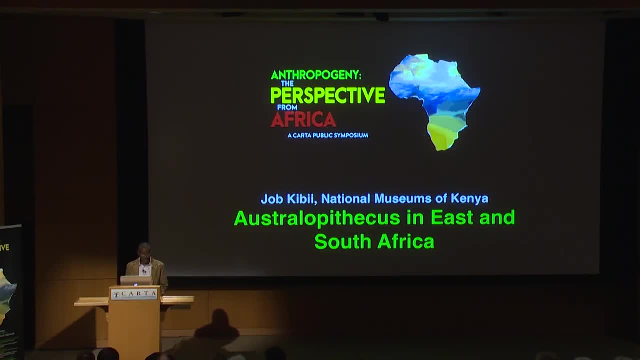 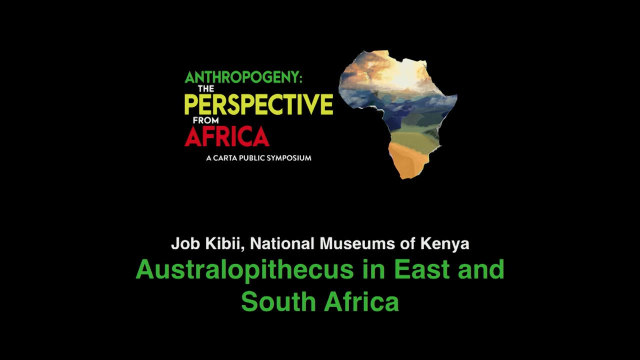 until the end. Yeah, so I've been invited to give a talk to the people of CARTA. I'm going to talk on Australopithecus in East and South Africa. It's quite an enormous task and I think I'll try. 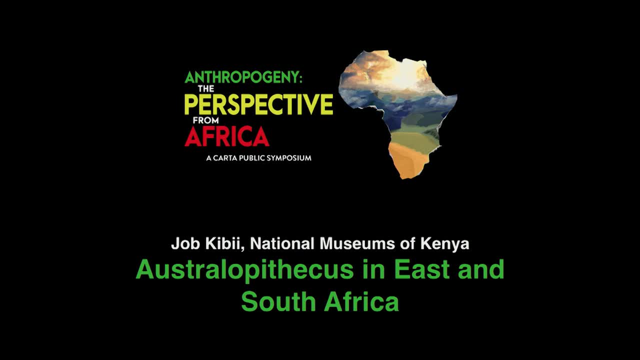 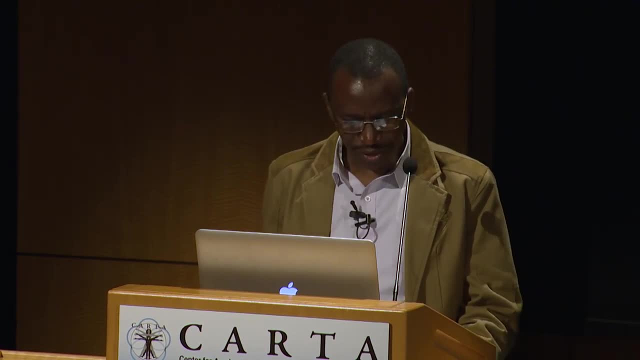 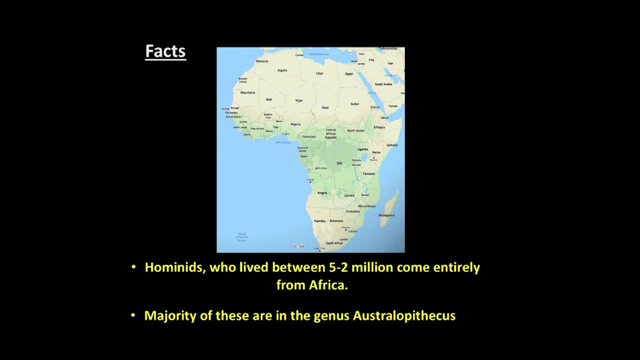 to do justice, because it's an enormous field of research that has gone on to make this research come to fruition. So let's get the facts for the first five million years of our evolution, since our common ancestors, With the closest cousins, the chimpanzees, At seven million years, those first five million years. 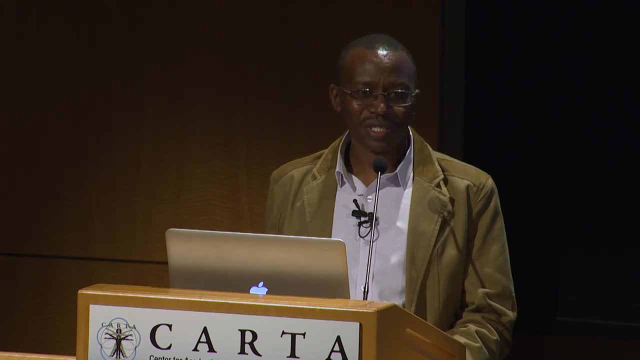 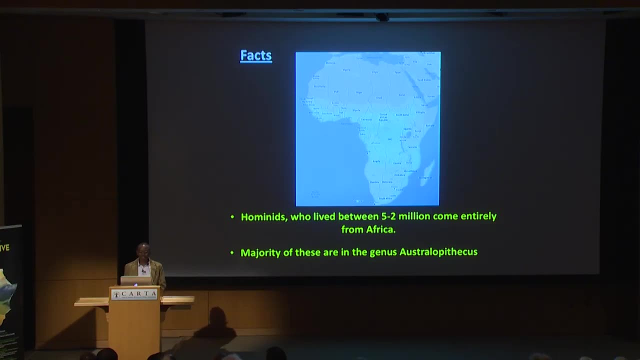 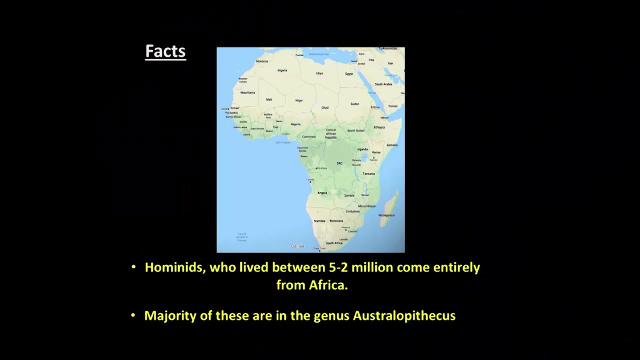 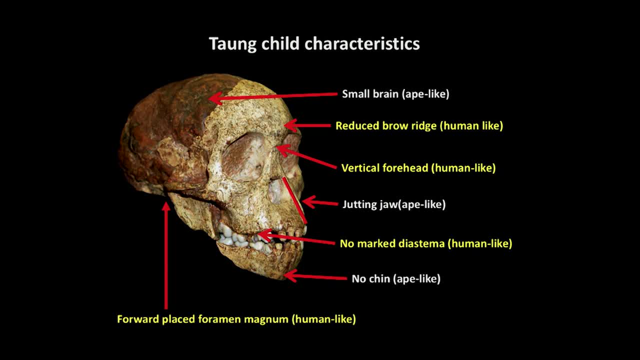 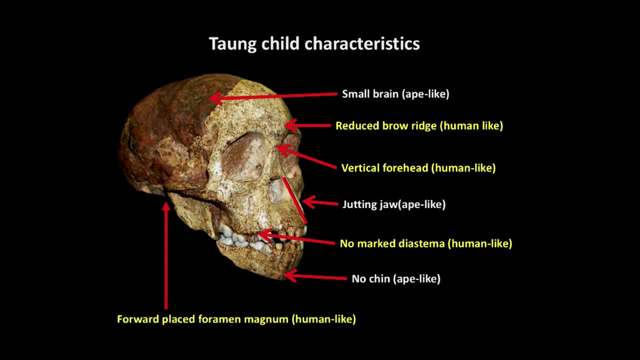 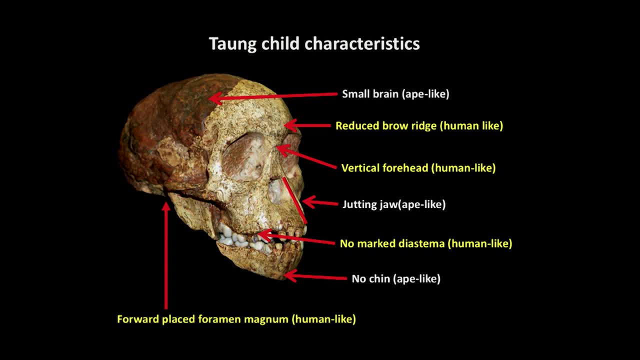 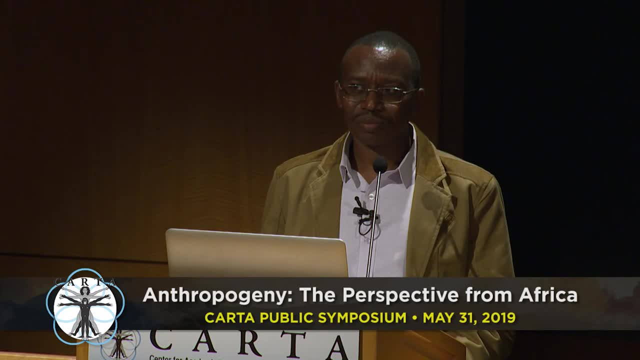 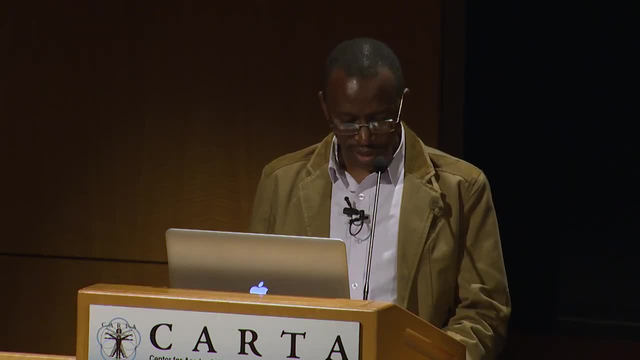 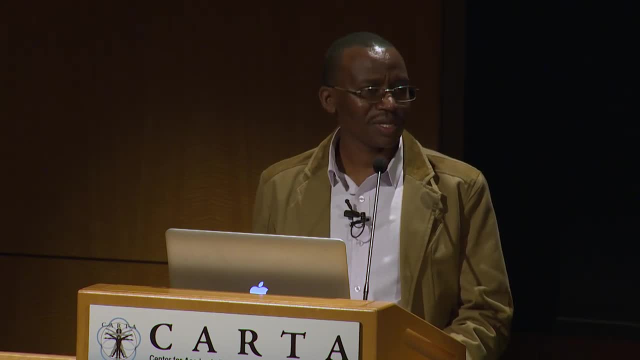 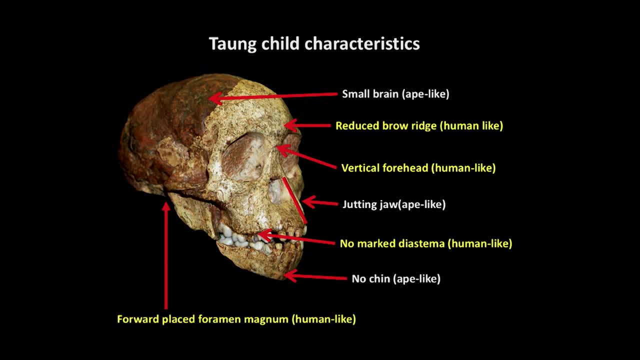 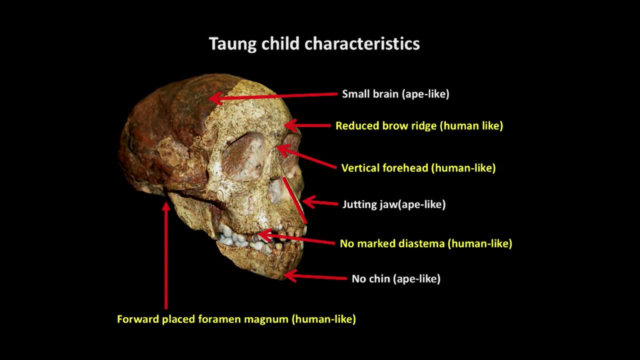 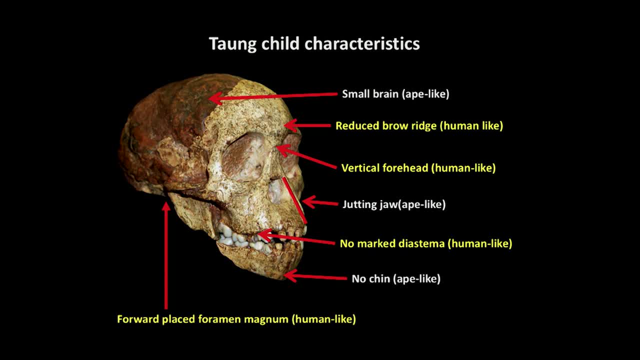 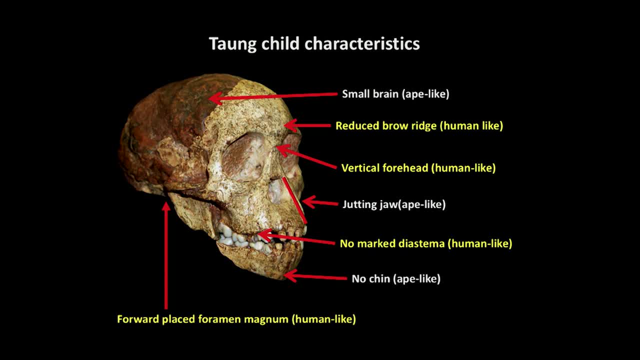 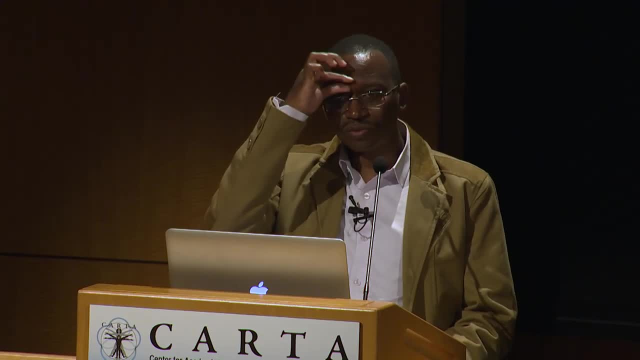 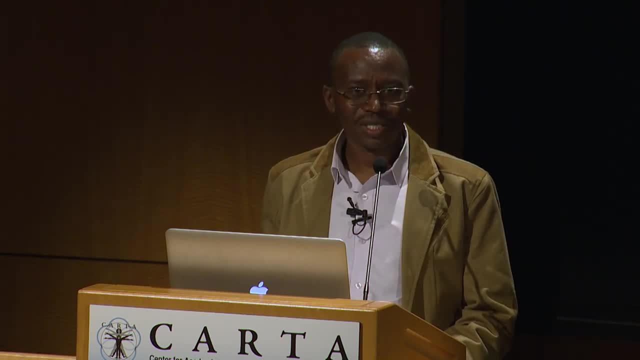 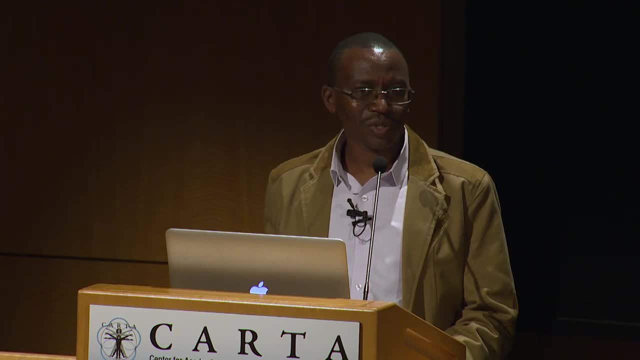 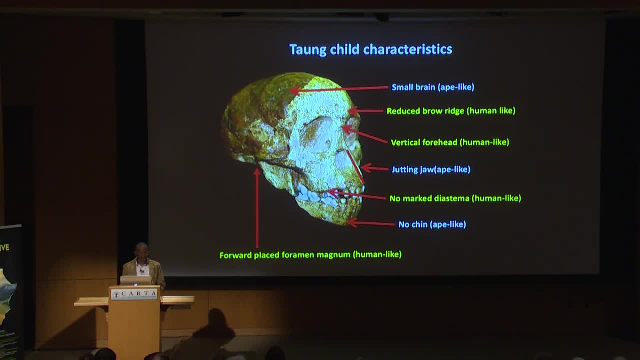 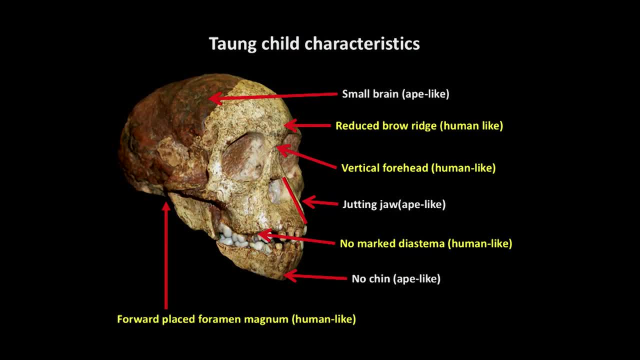 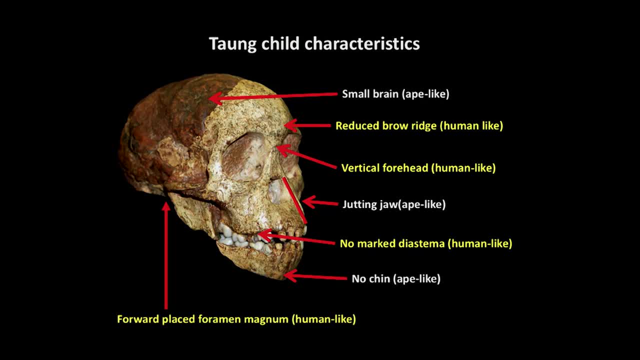 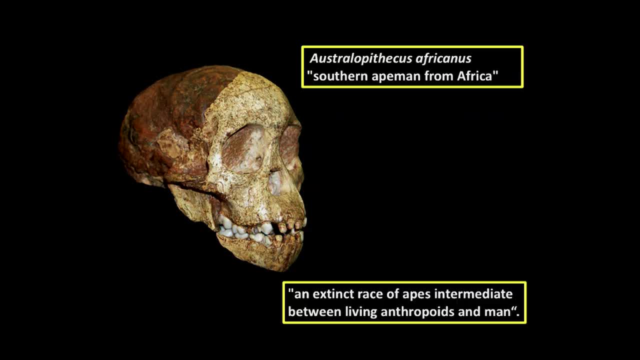 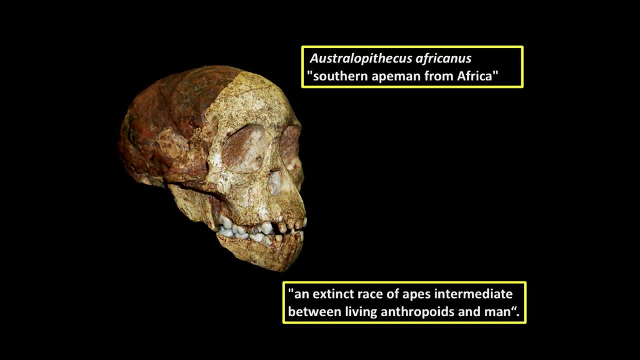 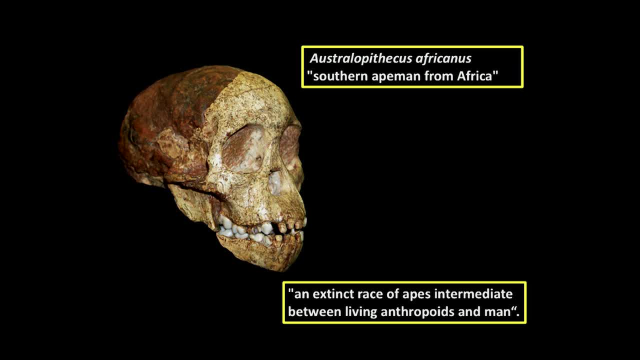 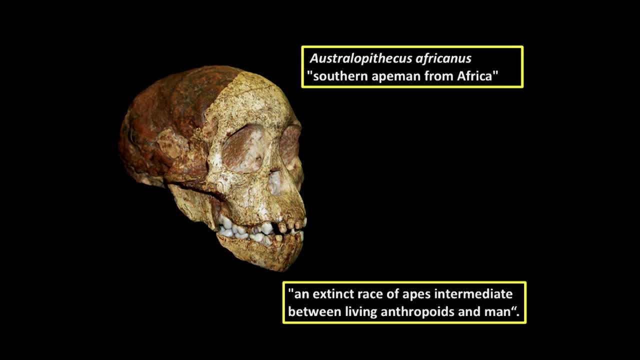 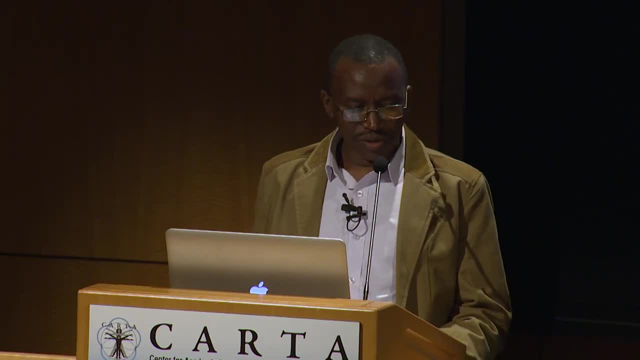 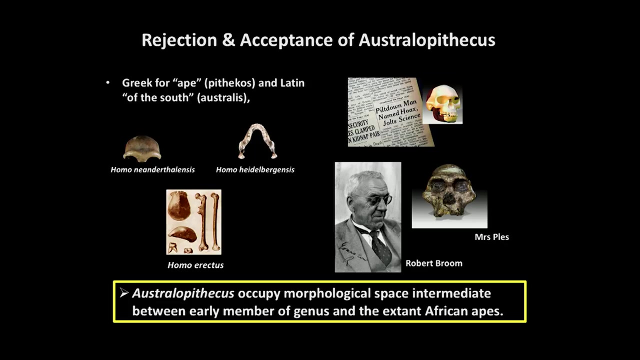 in man. However, this didn't go down well within the scientific community. He was criticized first for mixing Greek and Latin in coming up with the naming of the species. Also, at the same time we had the Piodan hawks. 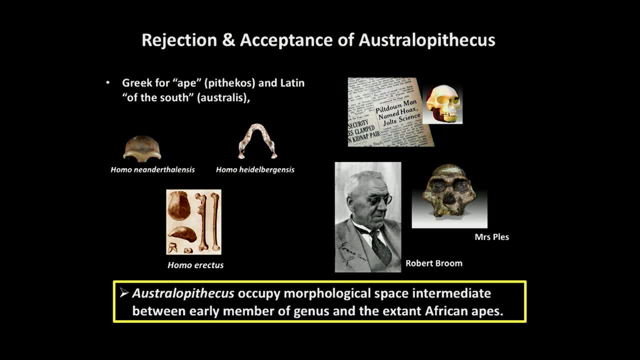 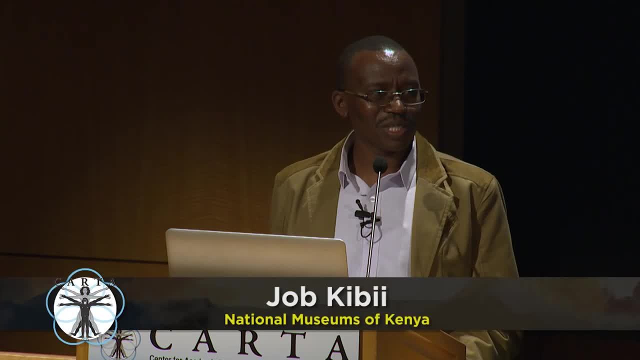 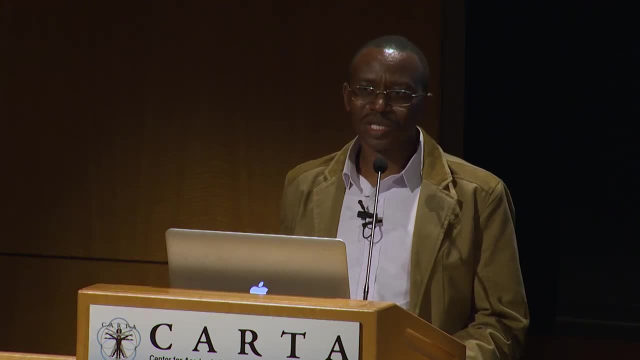 which had been engineered since 1912, and it indicated that the humans, or the ancestors of humans, we should be expecting a big brain and an ape-like jaw, and the rest of the body was supposed to be catching up in evolutionary terms. 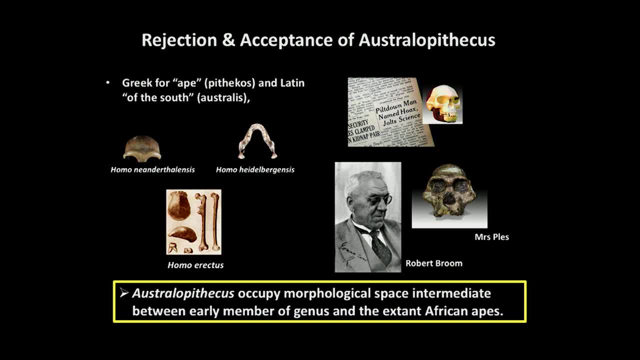 And also it didn't help that during that time Homo neanderthalensis had been discovered in Germany in 1856, Homo erectus had been discovered in Java in 1891, and Homo heidelbergensis had also been discovered in 1907. 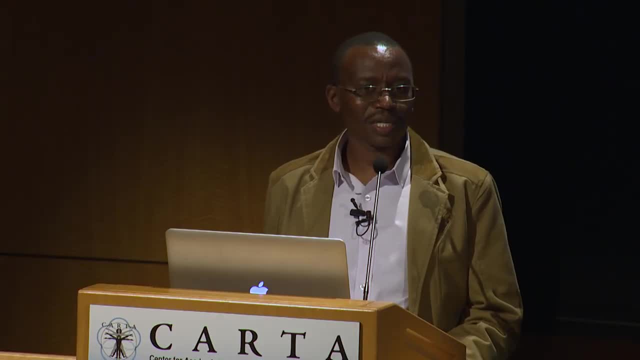 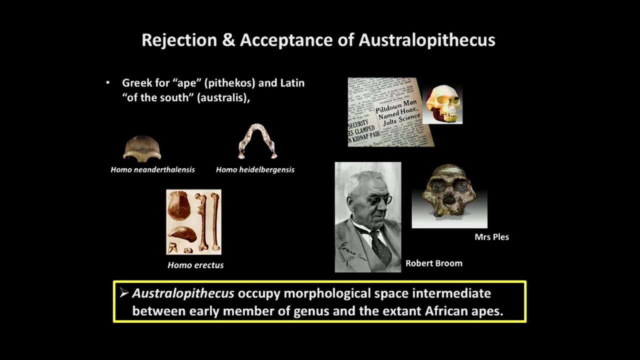 So there were already specimens that were already human-like, that were competing with the theory that Raymond Dart had indicated that Australopithecus africanus was ancestral to the humans And also because of the small brain, it was believed that the Australopithecus 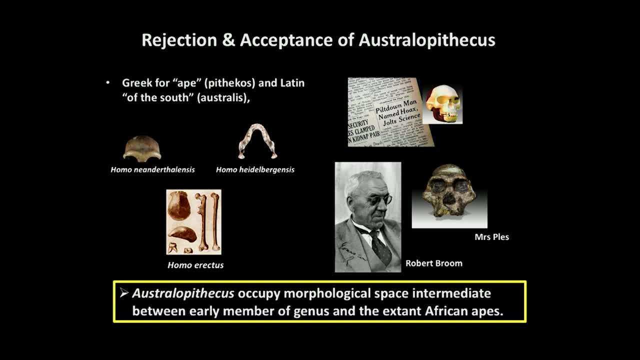 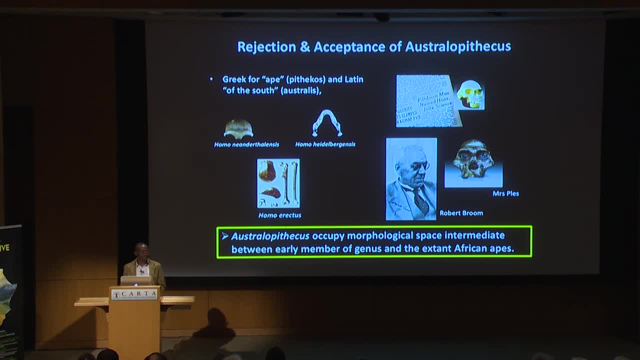 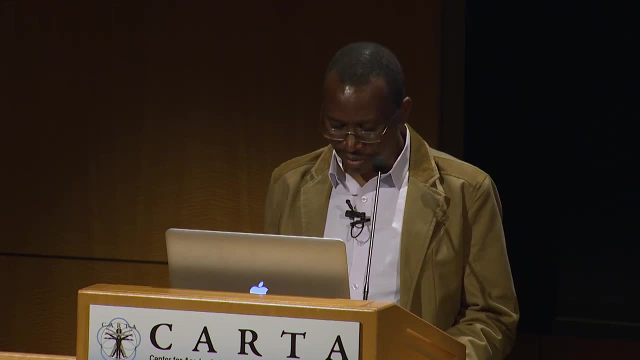 or the ancestors to humans, should have a big brain, and so Australopithecus africanus was contrary to what the scientific community believed at the time. But science has proved that that was right and we now believe there is a general consensus. 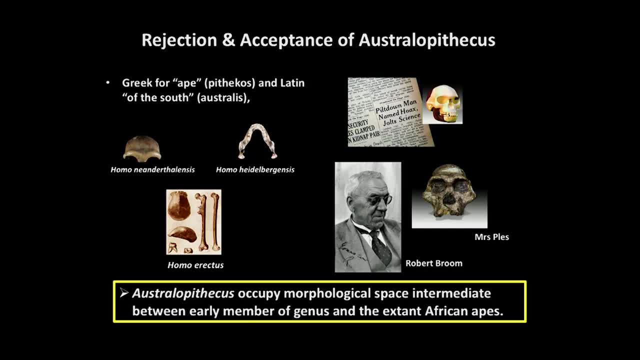 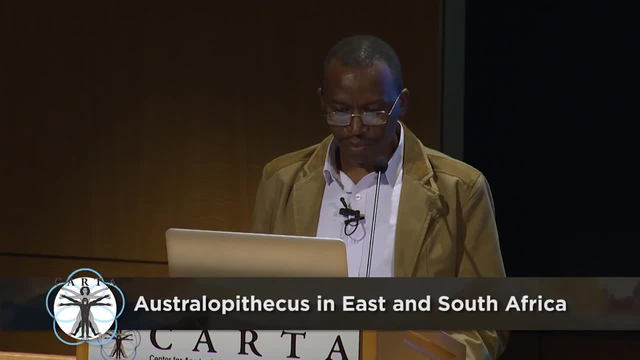 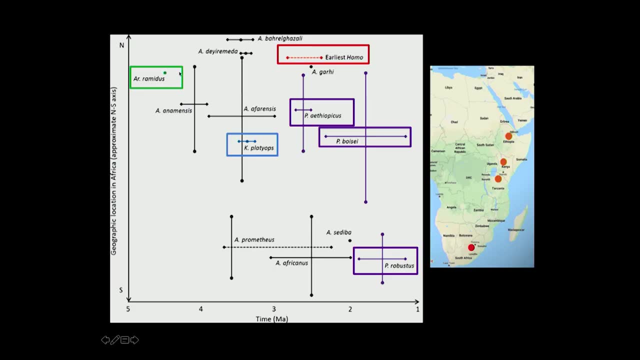 that Australopithecus occupy a morphological space intermediate between early members of genus Homo and the living African apes. Sometimes it's much more difficult for Australopithecus, which is there, and Kenyanthropus here, early members of Homo Paranthropus. 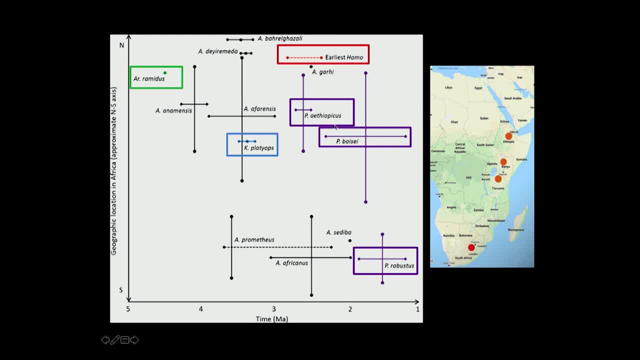 which we have Paranthropus aethiopicus in East Africa, Paranthropus boisei also in East Africa and Paranthropus robustus in South Africa. They merge these into the genus Australopithecus. 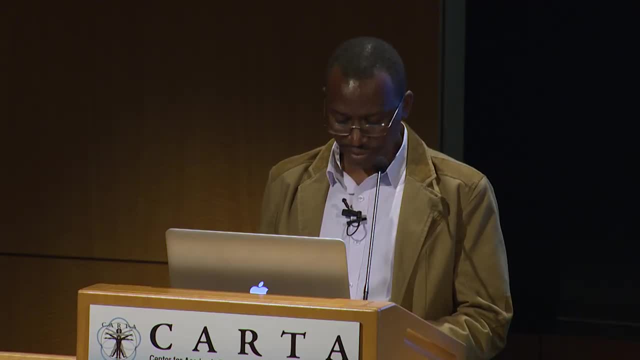 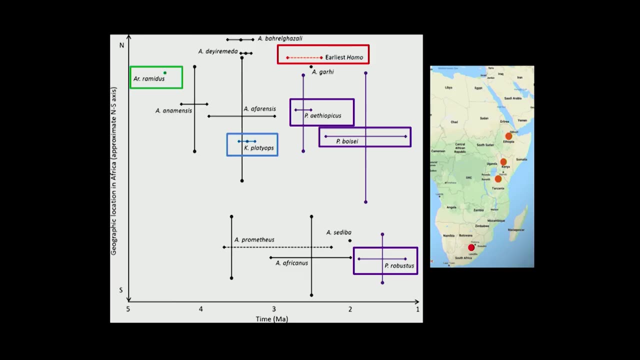 but this becomes too restrictive because they are clear anatomical differences between all the between the four groups, and these presentations does excludes members that are at any time referred to as Adipithecus Paranthropus Kenyanthropus. 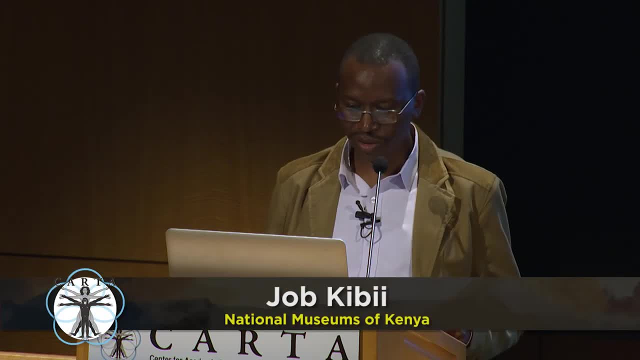 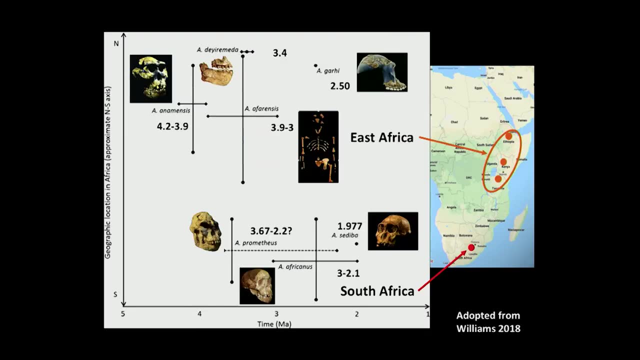 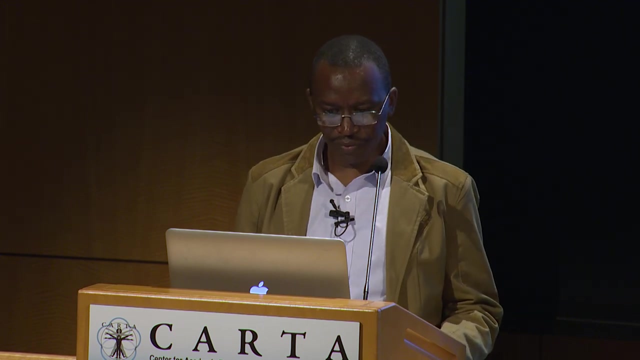 and Homo, and restricts the discussion on only members that have been referred as Australopithecus and in in East Africa and South Africa. In East Africa, we have a number of species that have been identified, and these are the ones. 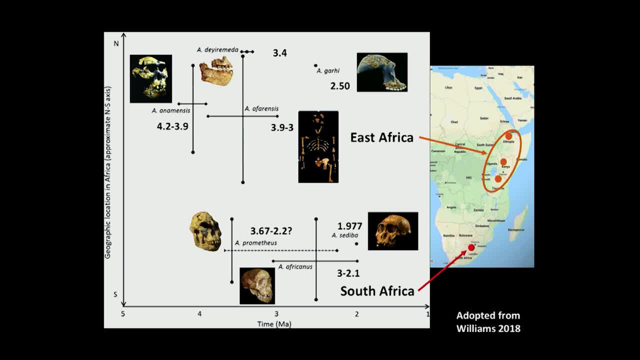 that have general consensus that they are within the genus Australopithecus. We have four species. we have the latest that have been discovered in Ethiopia. This is Australopithecus deilamidae. I hope I'm pronouncing that right. 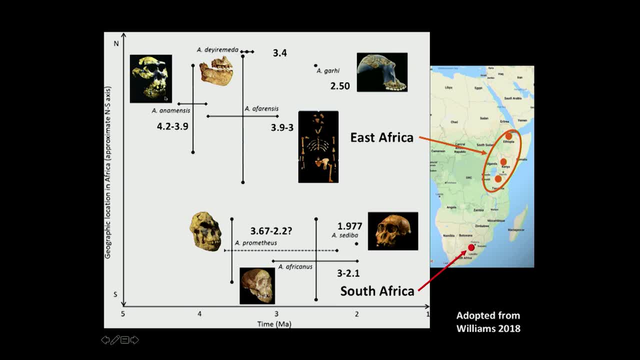 Bahan can correct me. These. Australopithecus anamensis discovered in Kenya. Australopithecus afarensis discovered in Kenya, Tanzania and Ethiopia. Australopithecus garae discovered in Ethiopia. 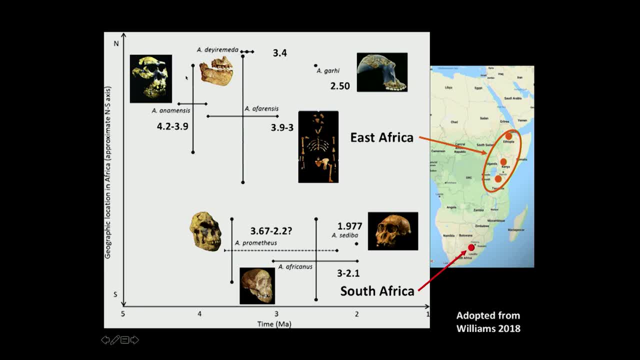 And the vertical lines indicate a species that have been found in more than one site. If it's just a dot, like in garae, it indicates it has just been found in just a single site And the horizontal line indicates the span. 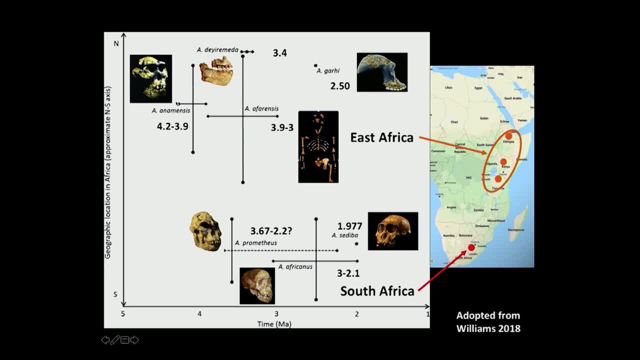 If it dates. there are dates that extend from, let's say, for example, anamensis 4.2 to 3.9 million years. but if it's just a single dot, that indicates that specimen has just one single date associated with it. 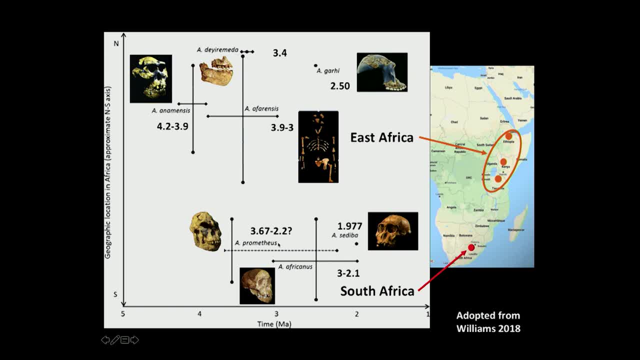 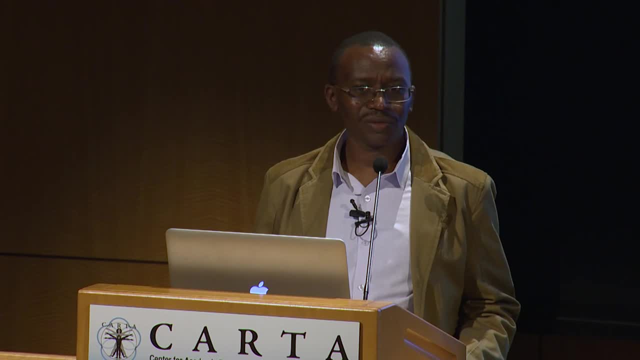 In South Africa we have Australopithecus prometheus. that was named in 1948, then kind of it was controversial whether that was. the specimens represented a species, a new species, and it was dropped off. But last year there were discoveries that named 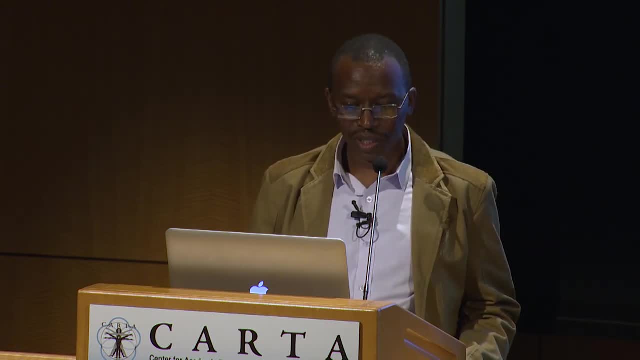 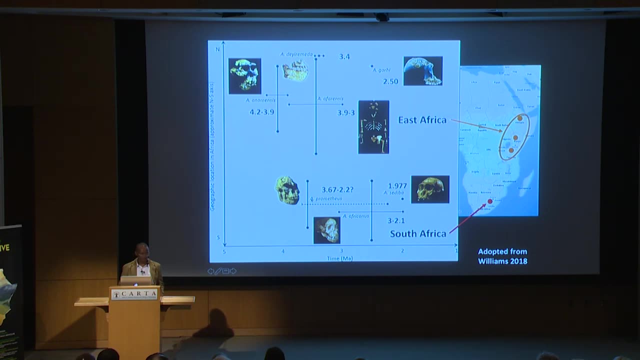 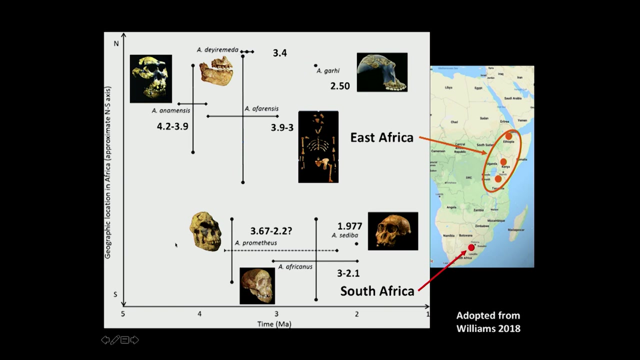 Australopithecus, revived the name. It's still controversial whether it's scientific to revive a name or whether the name should have fallen out of use. And the dates are still also controversial. We have dates that are at least 3.67 million years. 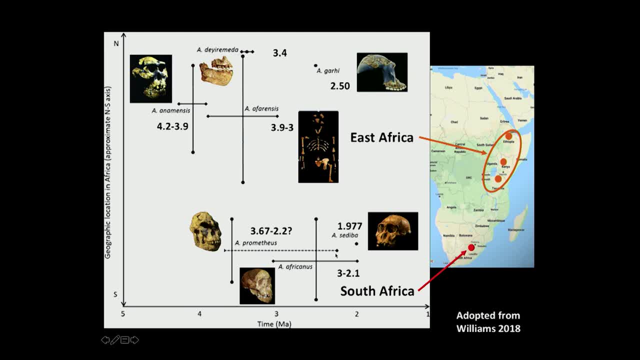 and some who suggest that the species in fact dates to less than 2.2 million years. So that's why we have that dotted line. In South Africa we also have Australopithecus sediba at 1.97 million years and Australopithecus africanus. 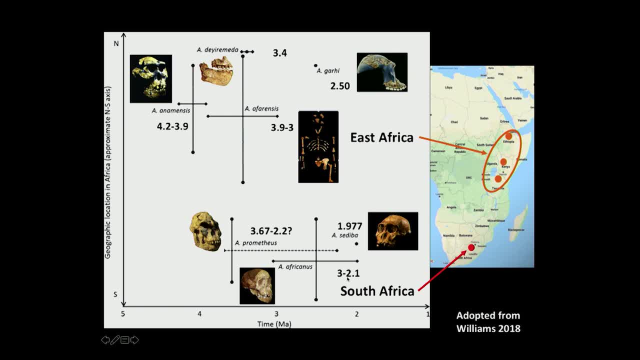 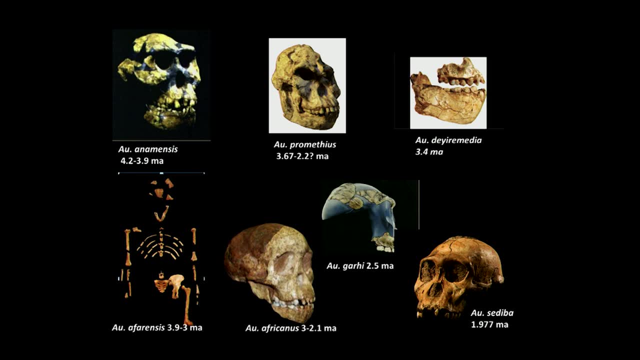 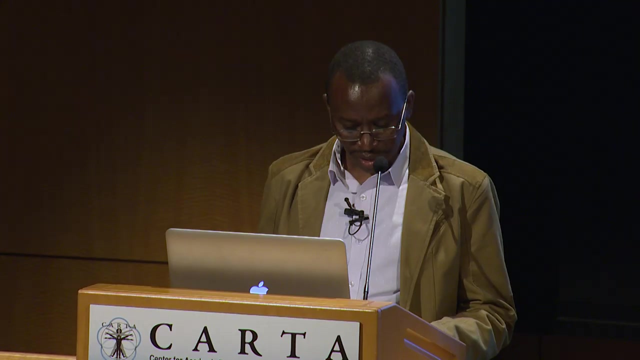 at 3 to 2.1 million years. While each of the species has its own particular morphological characteristics, time constraints do not permit discussing each species in isolation. Instead, I'll focus on morphological traits that are rather consistent right through that lineage. 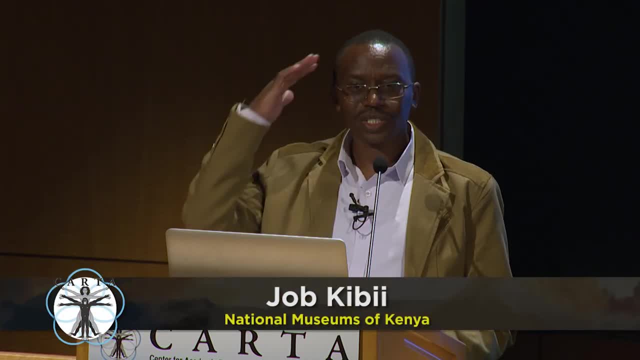 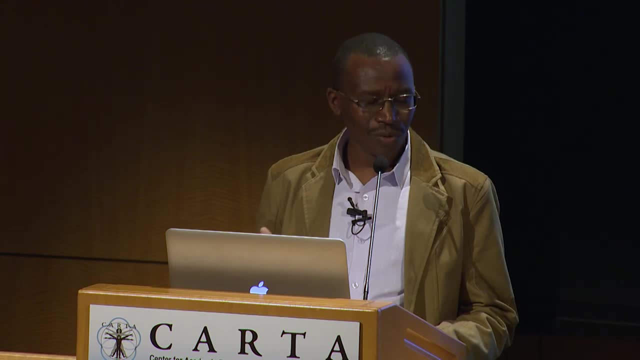 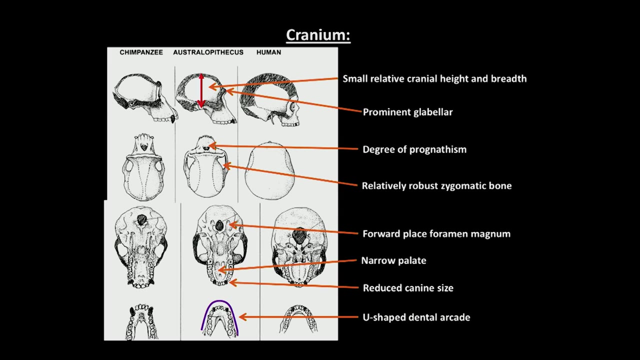 So what I'll do is I'll go down from the cranium, indicating what's common and how we understand, whether that contributed to who we are and what implications it has When you look at the cranium of Australopithecus. 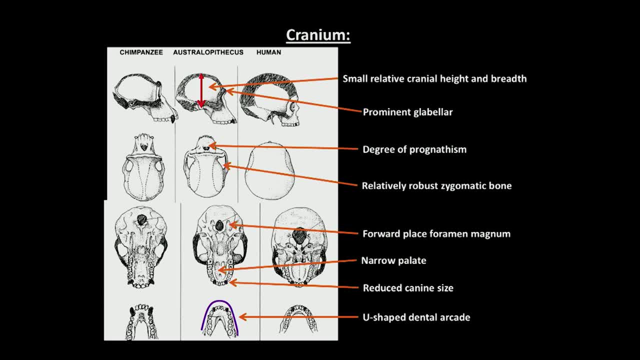 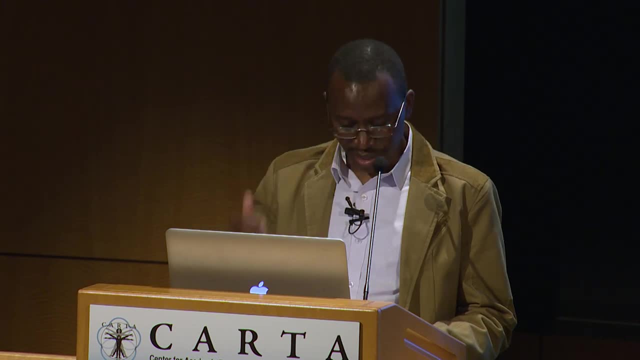 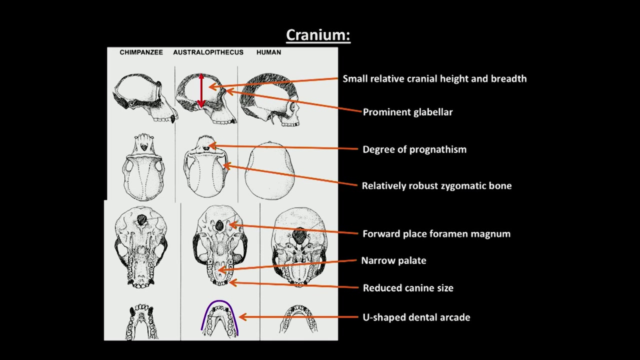 it shares several cranial characters, including a four word-placed foramen magnum, indicating that this genus was bipedal. They had small brain size, small relative cranial height and breadth, prominent grabera, which is this region here, and relatively robust zygomatic bone, and also they had a jutting jaw. 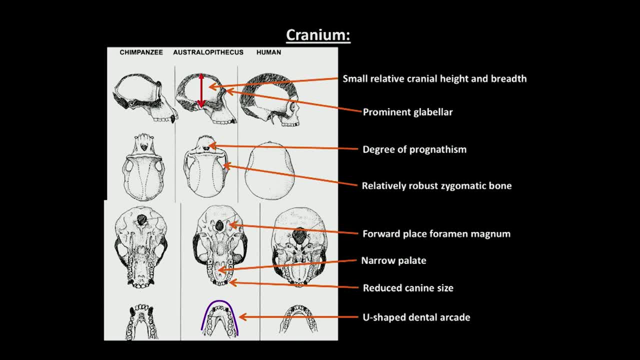 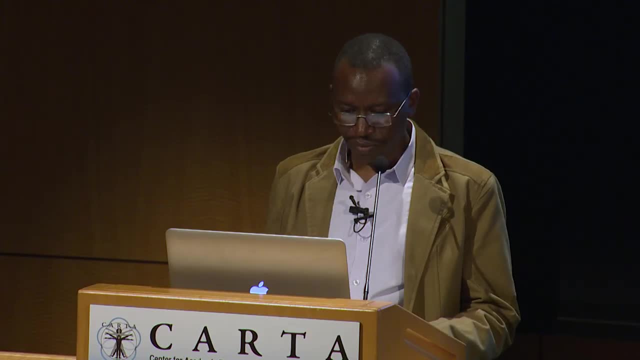 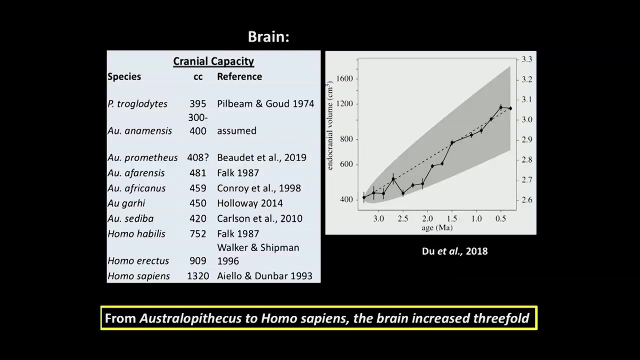 Those are just some of the characteristics. They also had U-shaped dental arcade. the chimpanzees have almost a rectangular dental arcade and the modern humans- we have a parabolic dental formula. When you look at the brain, the general trend in human evolution is an increase in cranial capacity and this trend becomes 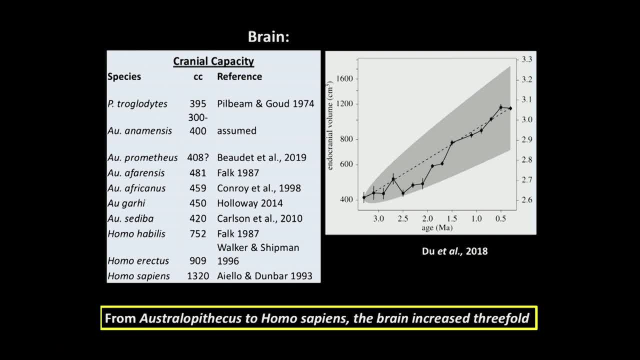 marked in the genus Homo and usually it's often associated with consumption of meat. We know that brain size increased more than three-fold from Australopithecus to our genus species. So you can see the Australopithecus here. they had very small. 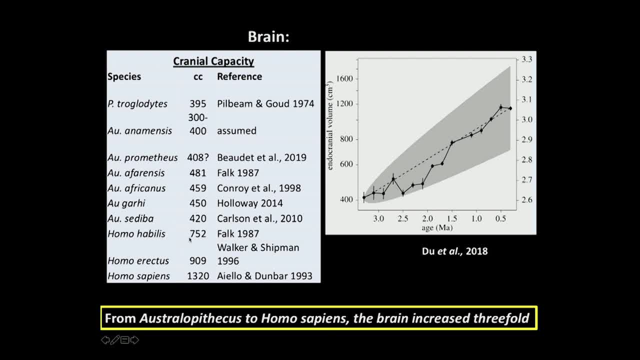 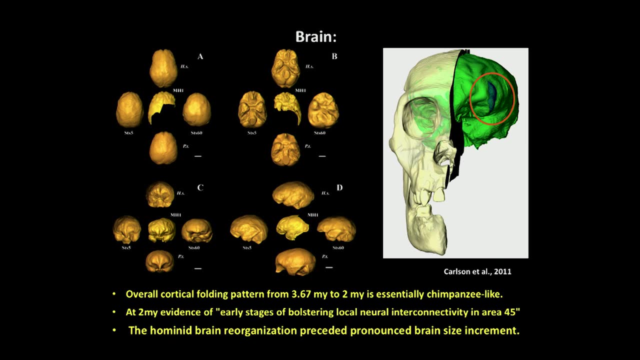 brain size and when you come to us it's more than it's almost about three times what you see in the Australopithecines. One critical question in human evolution is the timing, The timing and mode of early human, early hominid brain evolution As later as 2010,. 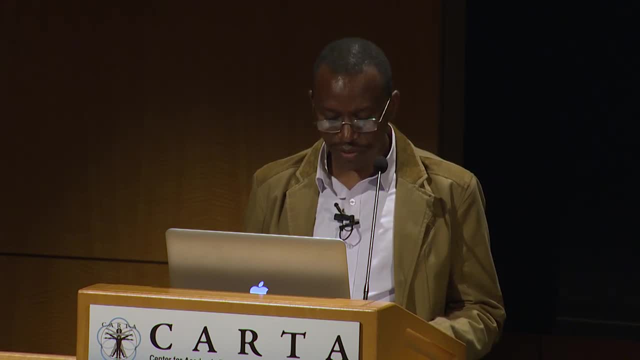 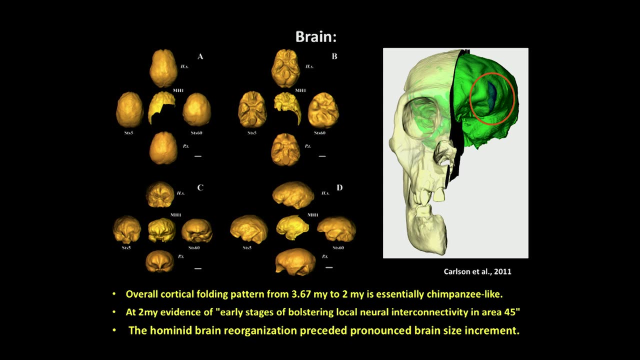 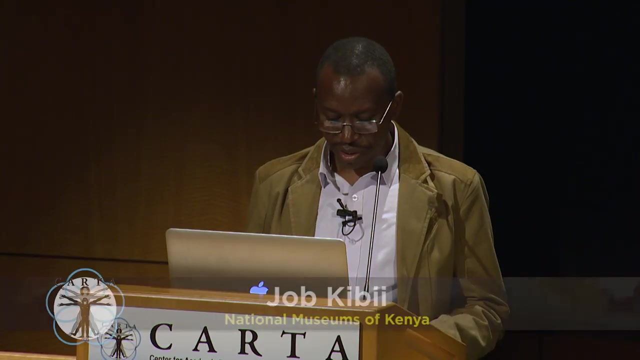 it was generally assumed that brain size increment preceded brain reorganization. From 3.6 million years- that's when we have the Australopithecus prometheus- to two million years, which is represented by Australopithecus sediba, research indicates that Australopithecus 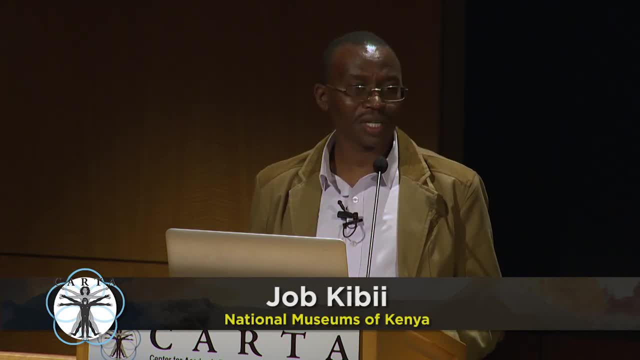 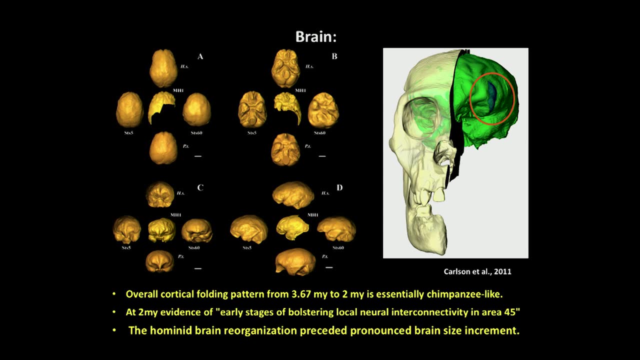 cortical folding patterns in the brain were essentially more than three-fold. in the brain, chimpanzee-like Brain volumes are also at risk at the upper end of chimpanzee variation. However, Australopithecus sediba, which is represented here, and also 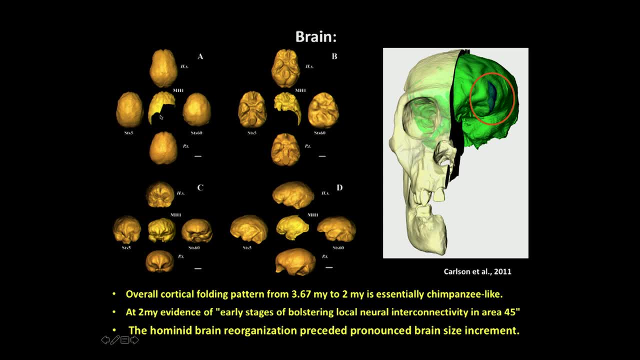 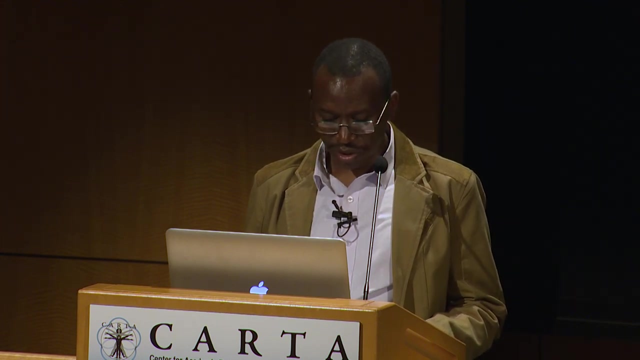 this is sediba, which was discovered in 2008.. Australopithecus sediba display human-like local protrusion in the inferior frontal area, which is that region that's highlighted here and which the researchers led by Chris Carlson. they call this as an implication of early stages of bolstering local neural. 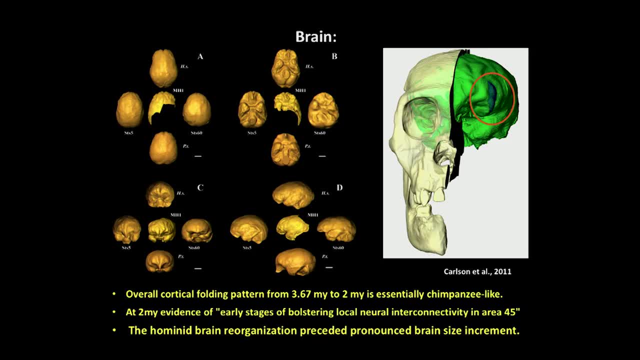 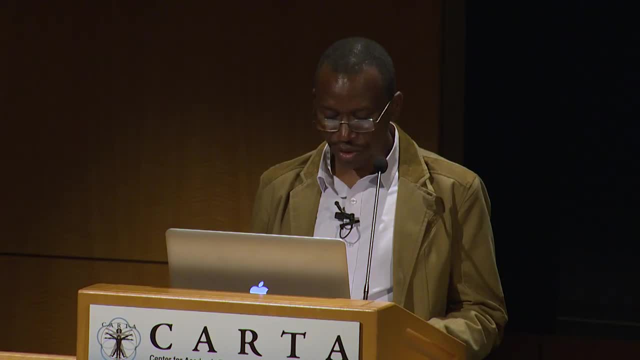 connectivity in area 45, in which, they argue, is related to speech. Thus the current consensus is that there is a gradual neural reorganization of the orbital frontal region in the transition from Australopithecus to Homo, but not gradual enlargement before transition. So 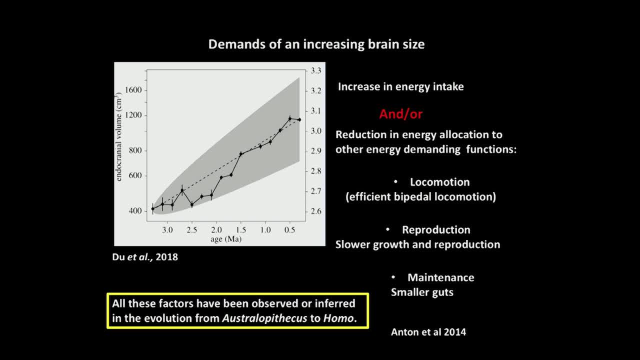 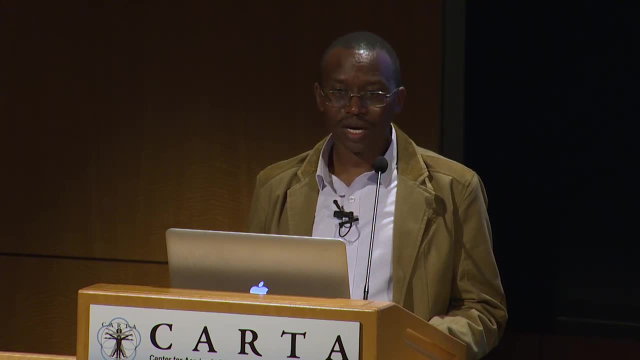 what does an increase in brain size demand? An increase in brain size demands an increase in energy intake and or a reduction in energy allocation to other energy demanding functions, For example by adopting a more efficient bipedal locomotion having a slower growth and reproduction. 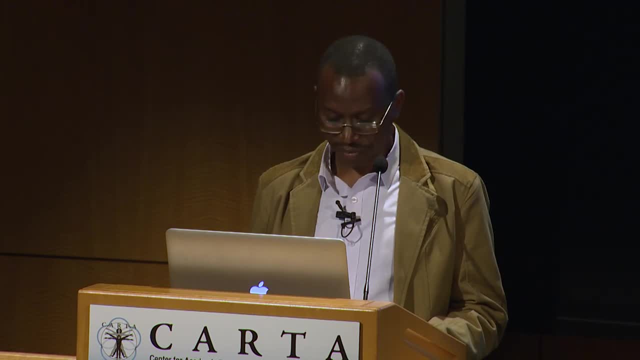 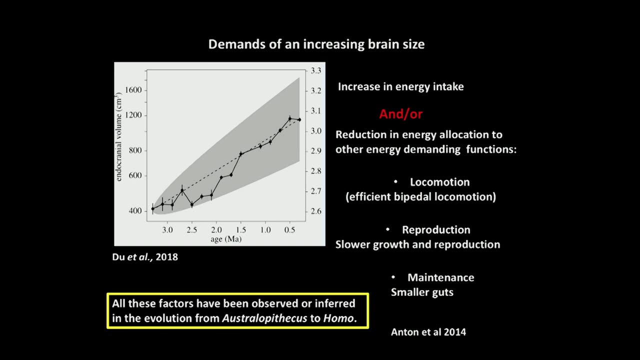 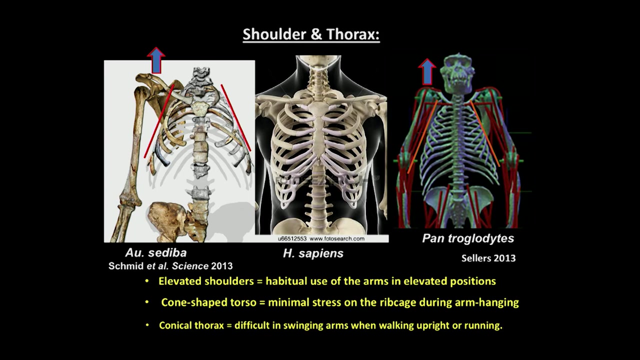 late and having smaller guts. All these factors have been observed or inferred in the evolution from Australopithecus to Homo. If you look at the shoulders and the thorax, Australopithecus genus is characterized by a relatively elevated shoulders and a conical shape in the upper thorax, which 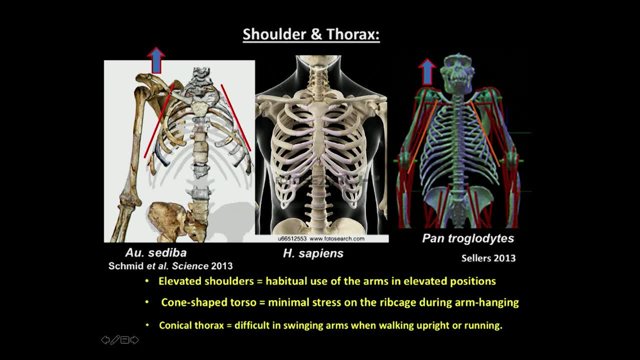 is. you can see, the shoulders here are elevated. This is a conical shape. This is a conical shape. This is a conical shape. This is an Australopithecus sediba. That's modern humans and that's the chimpanzees, The. 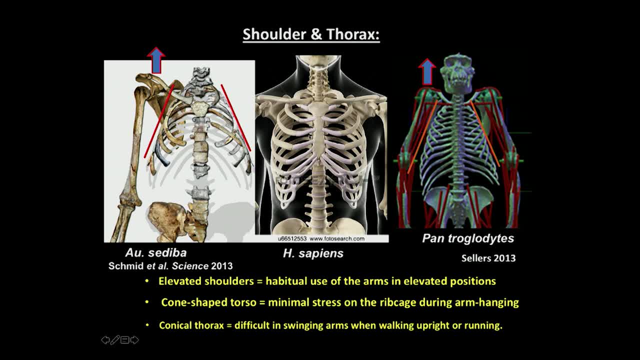 shoulders are elevated, So Australopithecus have this general shape, which is similar to what we see in the chimpanzees. The high position shoulders have been interpreted as indicative of upper limbs that were habitually used in overhead postures in the context of arboreal 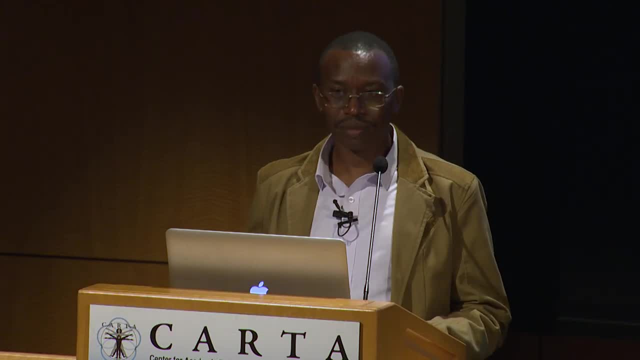 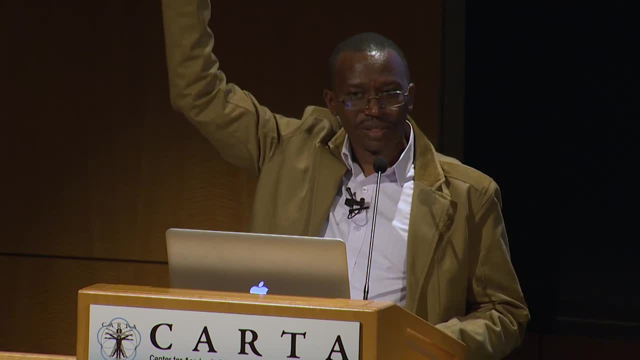 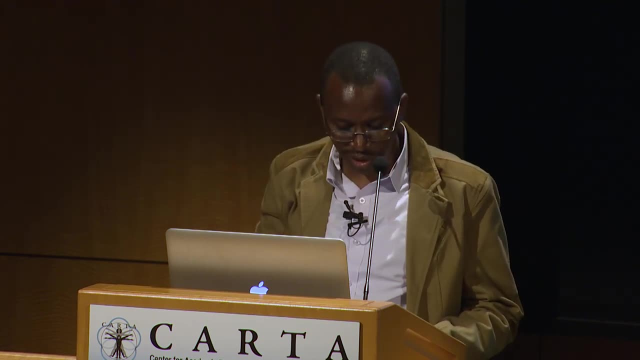 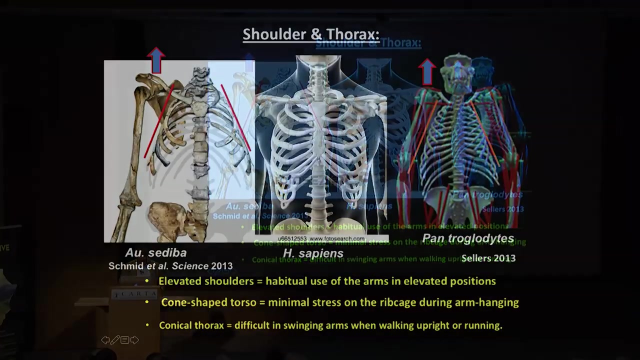 been using their arms like this, That's whether they were climbing or using that for movement on the trees. A conical shaped torso, as you can see on these, which is similar to what you see in the chimpanzees. the humans have a barrel. 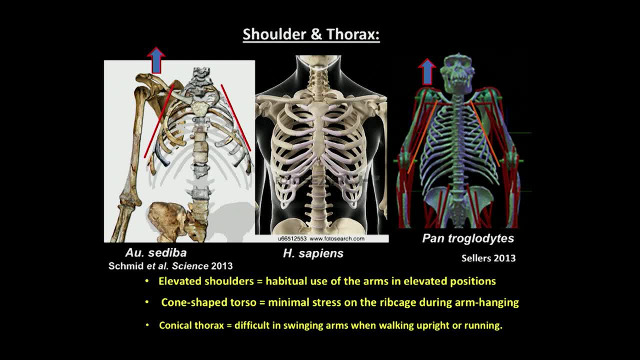 shaped torso. It is effective in the development of the human body. This is a conical shape. This is a conical shape. This is a conical shape. This is an is effective in evenly distributing stress on the ribcage during arm. 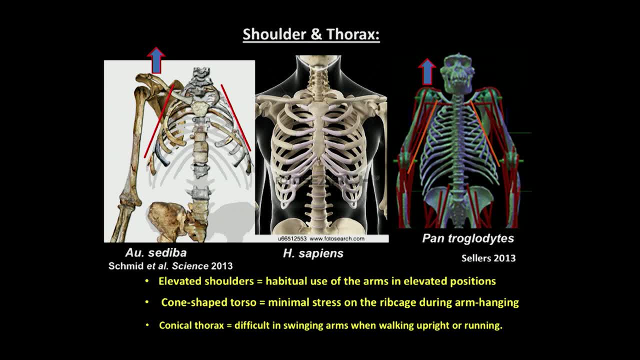 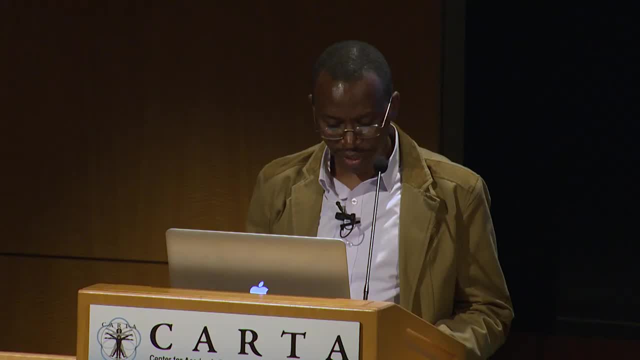 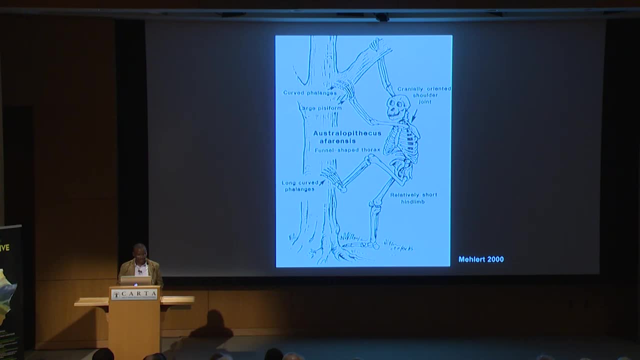 hanging. but also there is a drawback to that, because it makes it difficult to swing arms when walking upright or running. A barrel shaped thorax, as in modern humans, is well adapted for endurance, walking and running. This is a depiction of Australopithecus climbing. You have to agree with me. This has to be a. 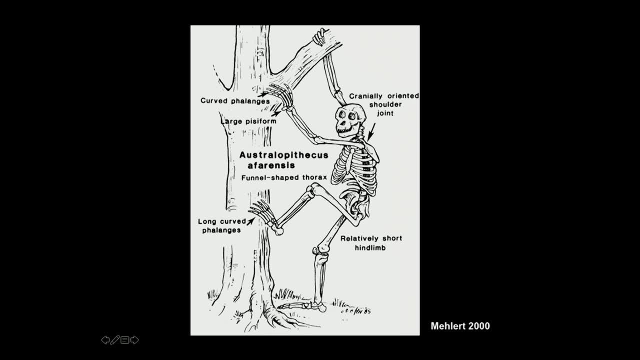 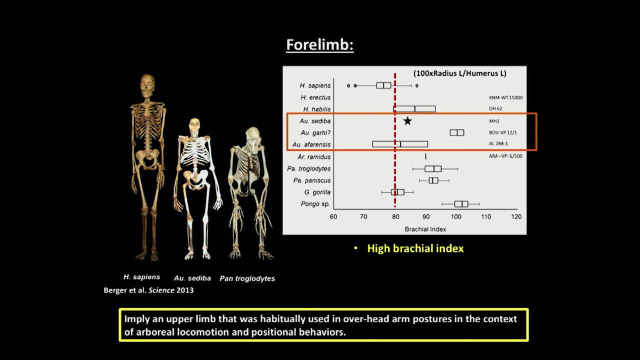 a very small tree if they are holding on the branch and also on the ground If you look at the forelimb. Australopithecus are characterized by long arms with particularly large joint surfaces and a higher branchial index. This is the higher branchial index is greater. 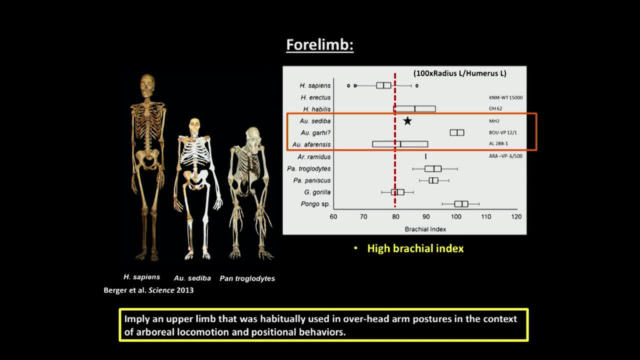 than the modern gorilla, but lower than the chimpanzees, which indicating retention of some degree of arboreal competency. This would also imply an upper limb that was habitually used in overhead postures in the context of arboreal commotion and positional behaviors. 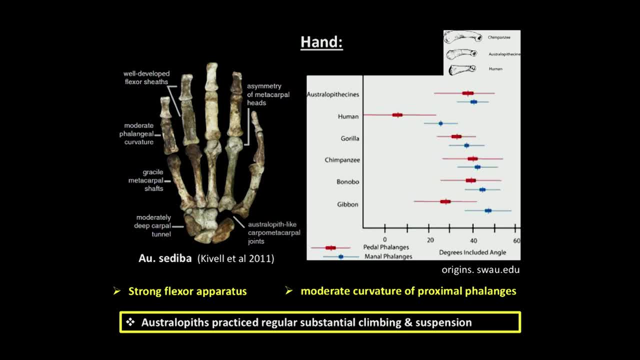 When we look at the hand, Australopithecus possessed long, robust and curved fingers with strong attachment sites for flexed muscles. The degree of curvature in the shafts of the fingers is correlated with frequency of arboreal behavior. Australopithecus phalanges are intermediary curved. 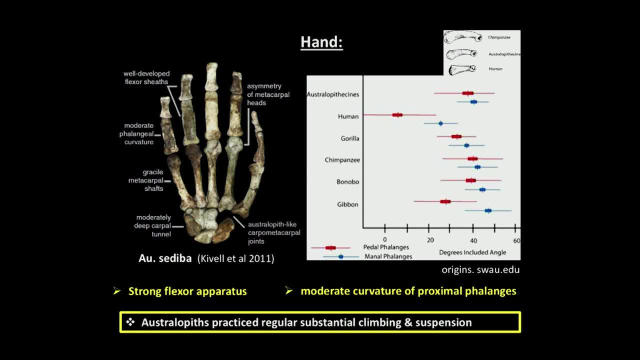 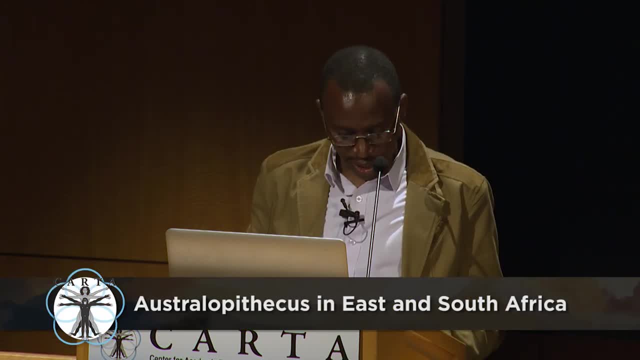 between those of modern humans and great apes, suggesting regular, substantial climbing and suspension. So the question is: did Australopithecus make stone tools And what we know is the earliest stone tools dated to about 3.3 million years? 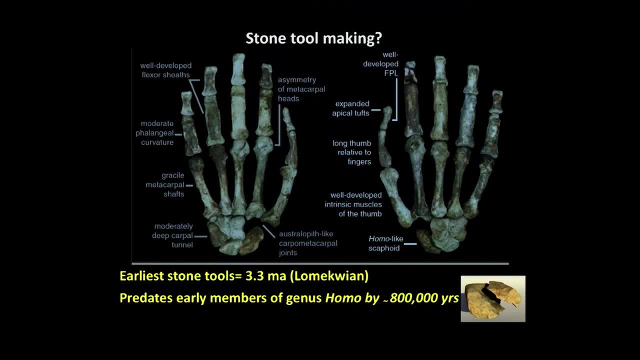 They are called Lomekwen and they predate the early members of the genus Homo by 800,000 years, and the genus Homo is thought to have made the stone tools, So most likely Australopithecus would have made stone tools. 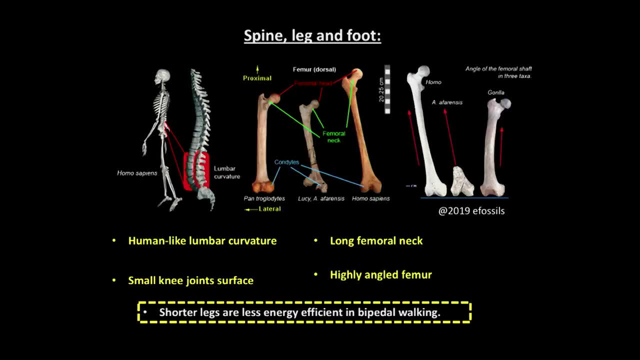 If you look at the spine and the legs, Australopithecus has five to six broad lumbar vertebrae that are curated to form a human-like lumbar curvature effective for weight transmission from the upper body to the pelvis, while also permitting the hips. 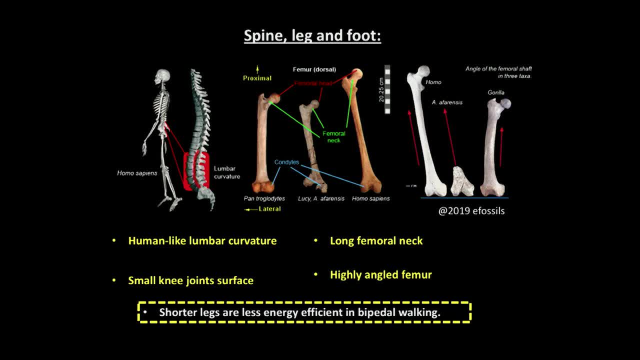 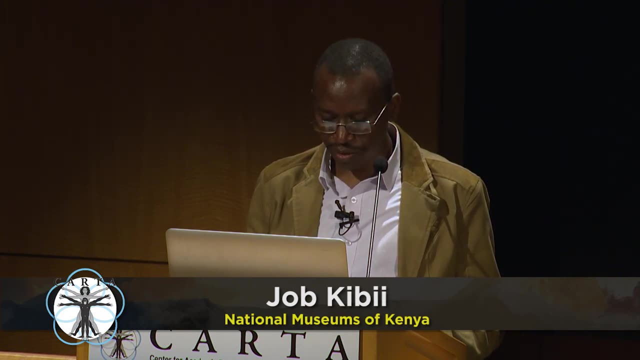 and the trunk to swivel forward during walking. Australopiths are characterized by relatively short legs, small femoral hands, small joint services and the small neck. the femoral necks, however, longer and anterior-posteriorly compressed than those of humans and chimpanzees, and more highly angled. 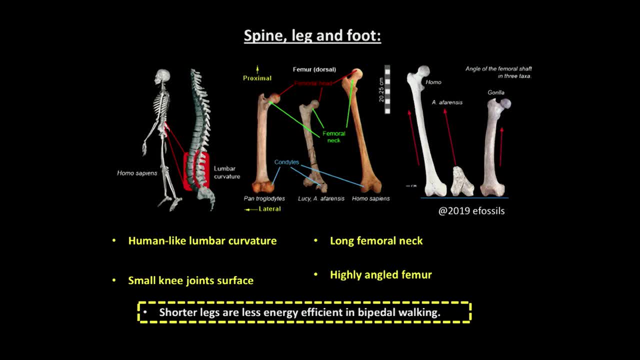 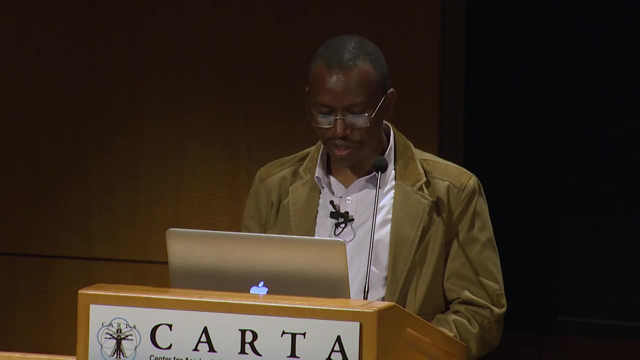 Shorter legs are less energy efficient. in bipedal walking, though, they help in lowering the center of gravity, hence increasing stability and balance while walking on an even substrate. Owen Lovejoy has suggested that long femoral necks increase the mechanical advantage of the hip muscle. 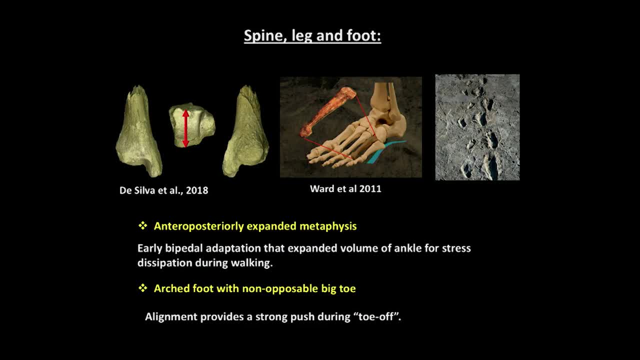 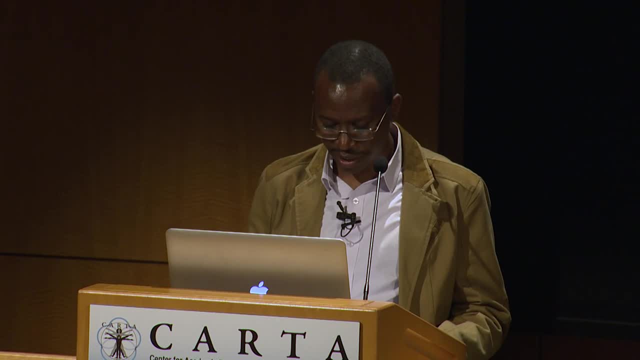 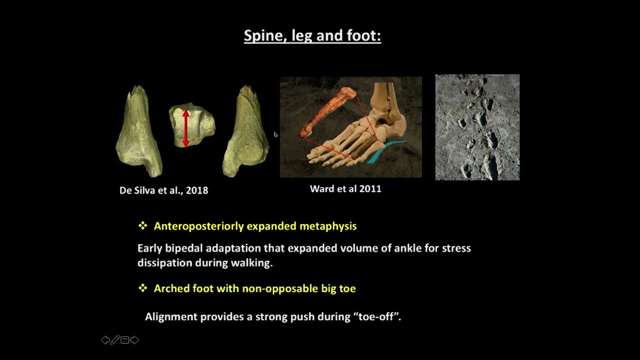 that stabilize the pelvis. When we look at also continuing on the spine and the leg, the distal tibia in Australopithecus is characterized by an anterior-posteriorly expanded metathesis. that's this region here that has been interpreted. 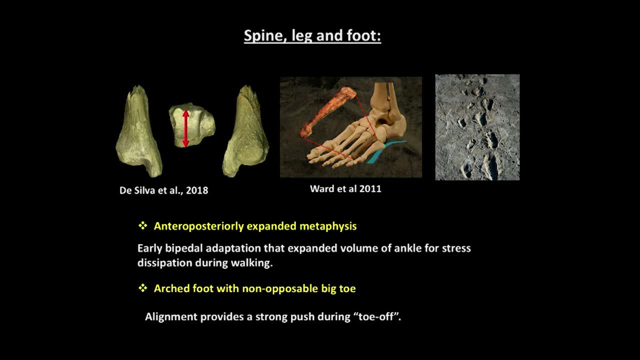 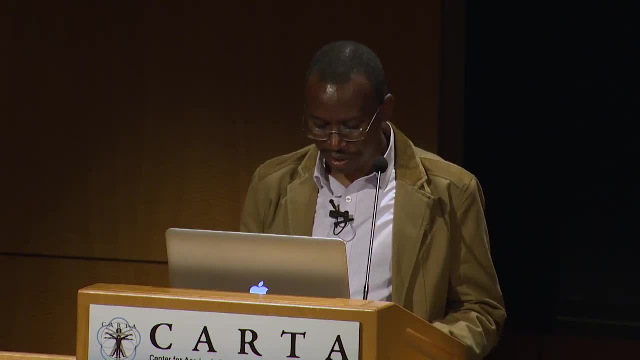 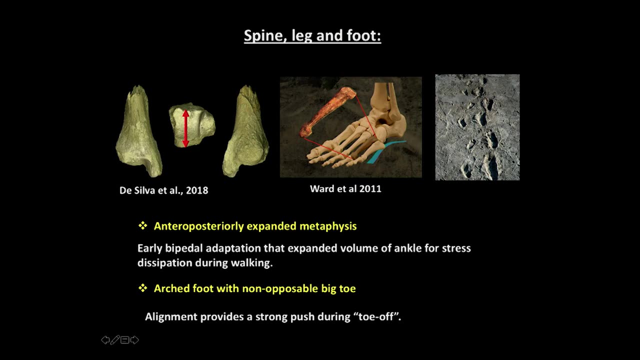 as probable early bipedal adaptation that expanded volume of anchor for stress dissipation during walking. The foot of Australopithecus has a large immobilized toe that's in line with other toes, as it's evident in the 3.6 million-year-old 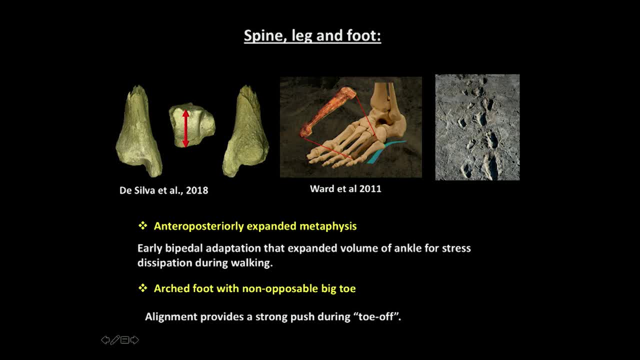 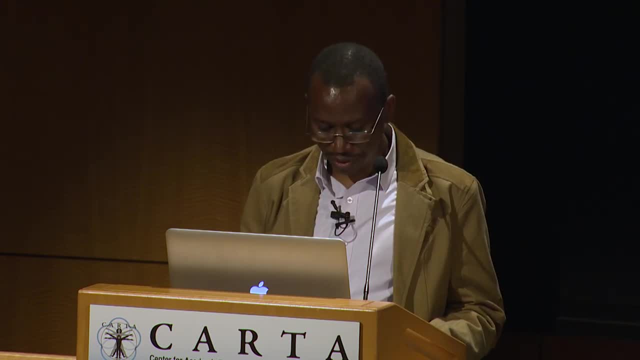 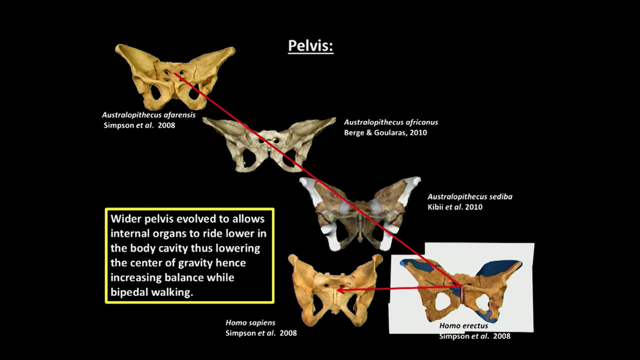 light-holy footprint and this alignment provides a strong push of dueling toe-off. While the pelvis of Australopithecus is human-shaped, it's extraordinary broad, with a wide side-to-side birth canal, small sacral and coaxial joints. 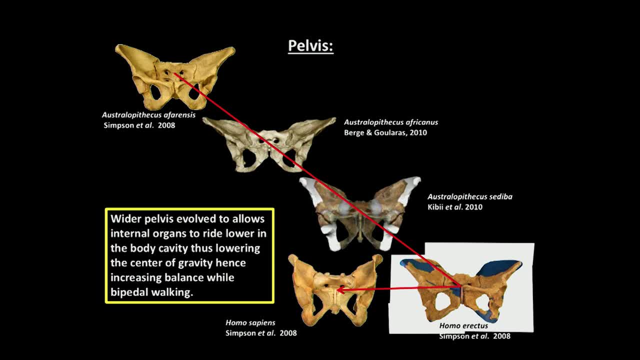 long pubic rami. Kevin Hunt has argued that a wide side-to-side birth canal, a wider pelvis, evolved to allow internal organs to ride lower in the body cavity, thus lowering the center of gravity, hence increasing balance while bipedal walking. 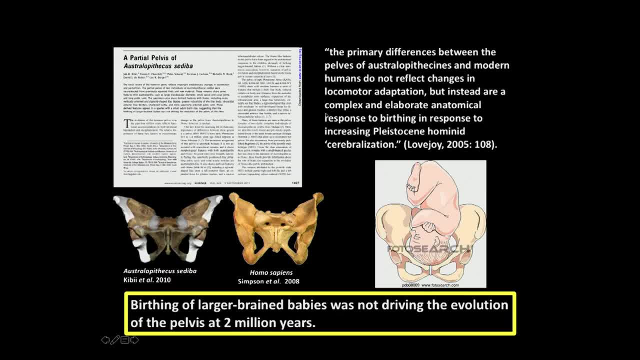 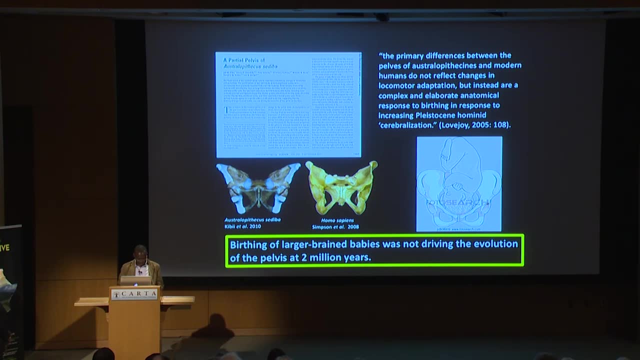 Prior to discovery of Australopithecus sediba shown here- and this is modern humans- it was assumed that homo-like architecture of the pelvis was a result of giving birth to large brain babies In 2005,- Lovejoy. 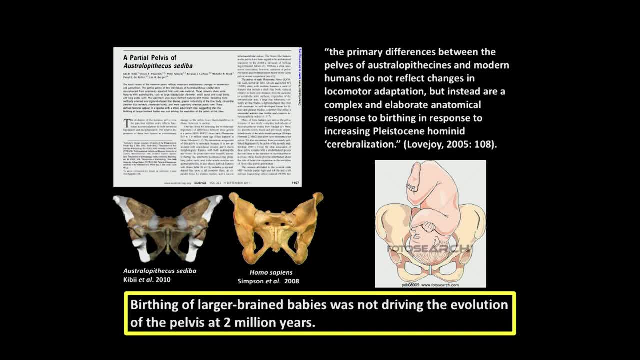 argued that the primary differences between the pelvis of Australopithecines and modern humans do not reflect changes in locomotor adaptation, but instead are a complex and elaborate anatomical response to birthing, in response to increasing prestocene hominid cerebralization. 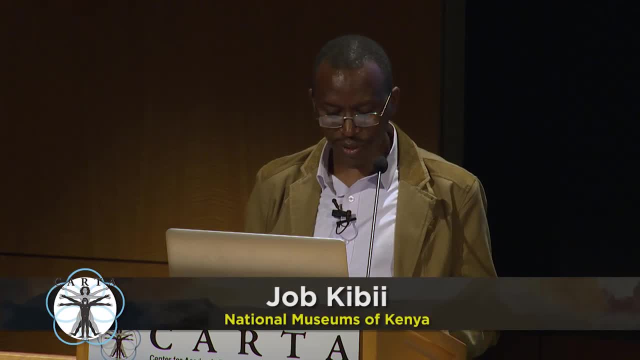 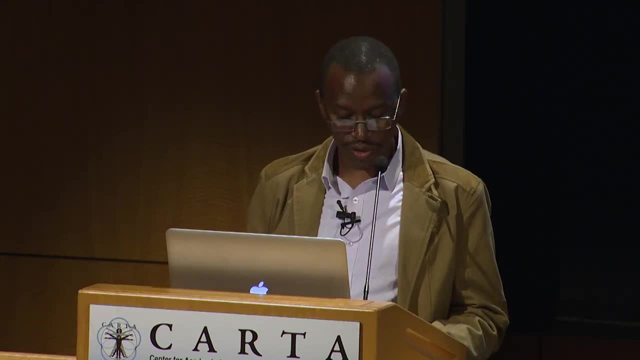 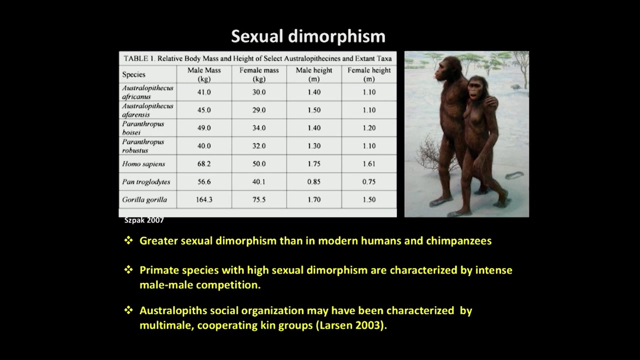 However, the homo-like pelvis Australopithecus sediba, coupled with a small adult brain, suggests that birthing of large brain babies was not driving the evolution of the pelvis at two million years. Looking at sexual dimorphism, Australopithecus exhibit a greater degree. 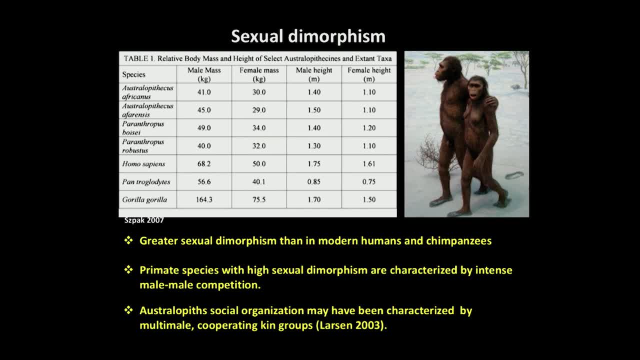 of sexual dimorphism than in modern humans and chimpanzees. They possessed body weights between 25 to 60 kilograms, with males at the high end and females at the low. Females weighed somewhere between 50 and 70% of male. 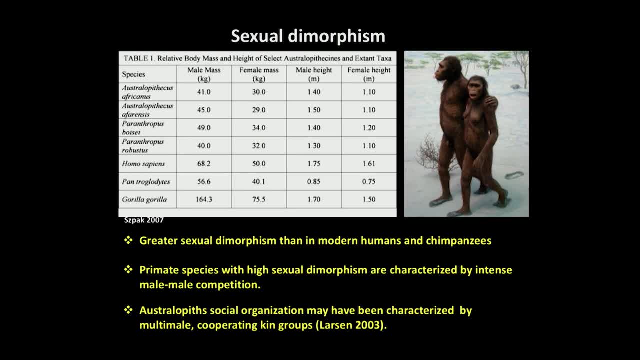 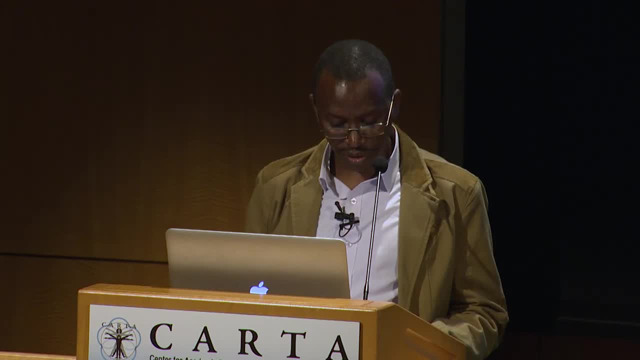 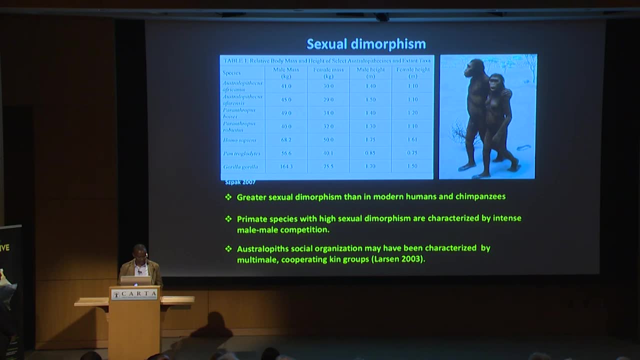 in modern humans, females weigh about 85% of the male body weight. The degree of sexual dimorphism has implications on social organization as well as mating systems. Primate species with higher sexual dimorphism are characterized by intense male-to-male competition. 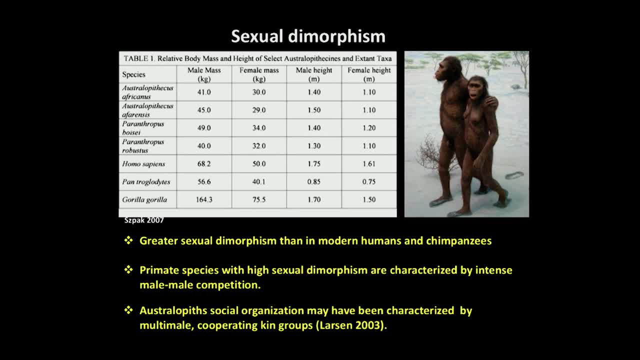 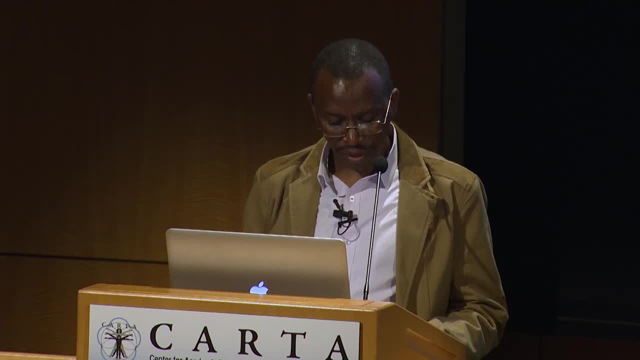 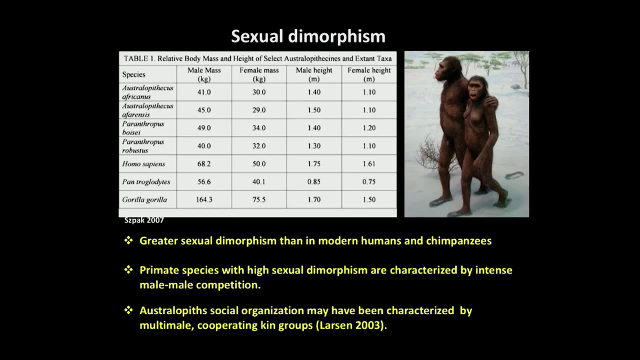 As Larson has observed, although chimpanzee adult males express aggressive behavior toward one another, they tolerate each other, live in multiple multi-male kin groups and are collaborative, especially in defending territory. Australopithecus social organization may similarly have been characterized by multi-male cooperating kin groups. 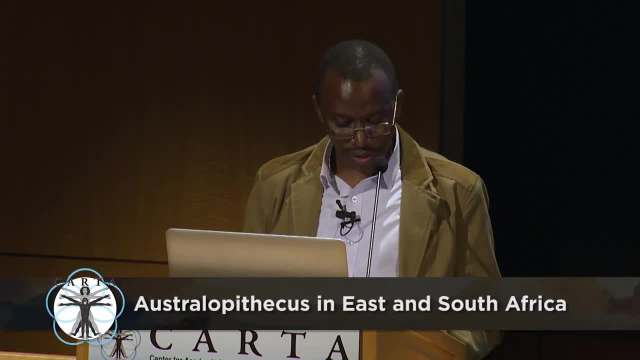 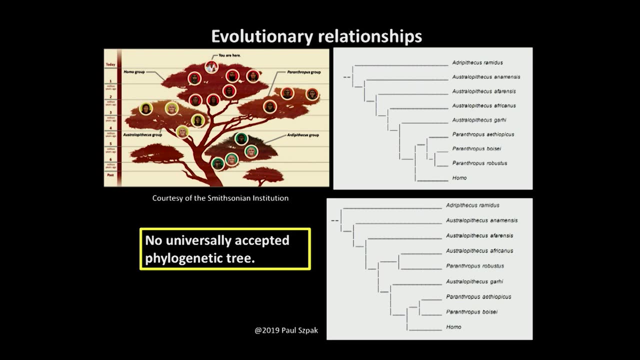 So what are the evolutionary relationships? Reconstructing hominid virology is extremely problematic and highly controversial. There is no consensus among perianthropologists on how to go about it. in the first place, Does one use age of the fossil geographical locality? 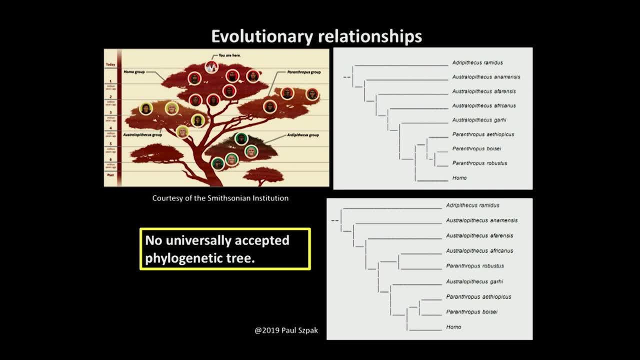 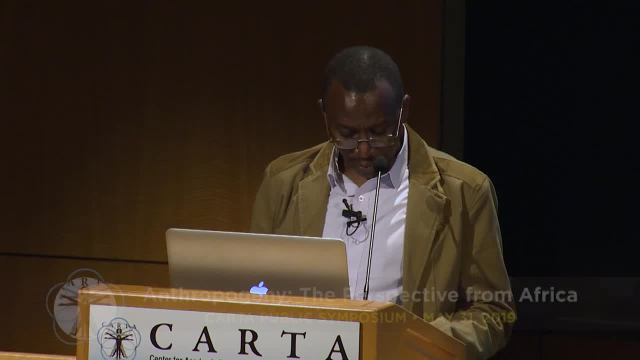 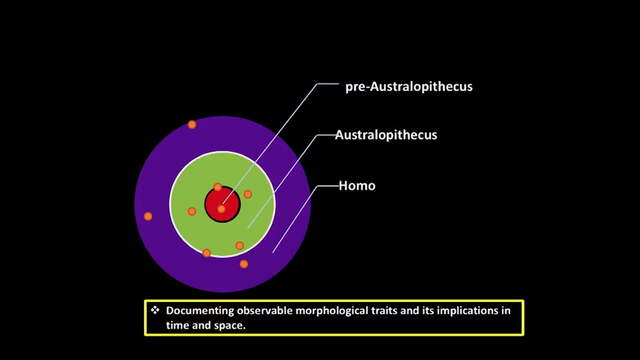 morphological traits and, if so, how many of those morphological traits to use. Thus, there is no single, universally accepted phylogeny. My preference is not in drawing lines connecting one species to another, but documenting morphological traits and reasoning about the implications of that. 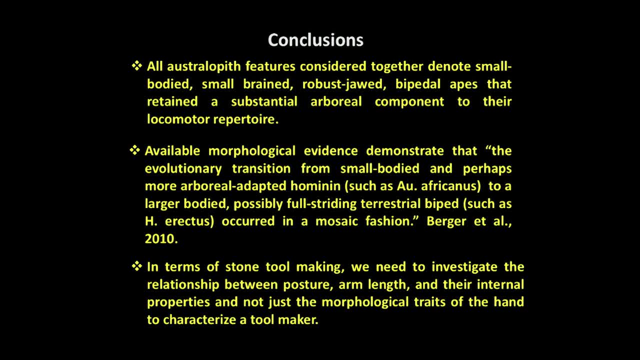 in time and space. In conclusion, there are three major conclusions that can be drawn from the studies we have about Australopithecines. One: all Australopithecines features considered together denote a small-bodied, small-brained, robust. 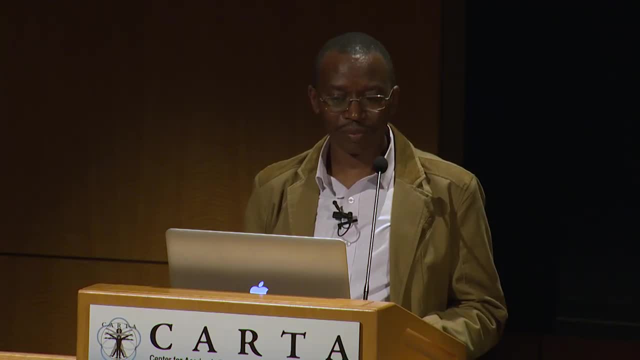 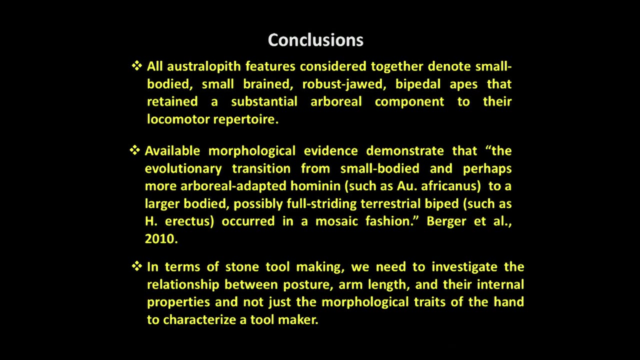 jawed bipedal apes that retained a substantial arboreal component to their locomotor repertoire. Available morphological evidence demonstrate that the evolutionary transition from small-bodied- and perhaps morphological traits- to small-bodied, more arboreal-adapted hominins, such as Australopithecus, 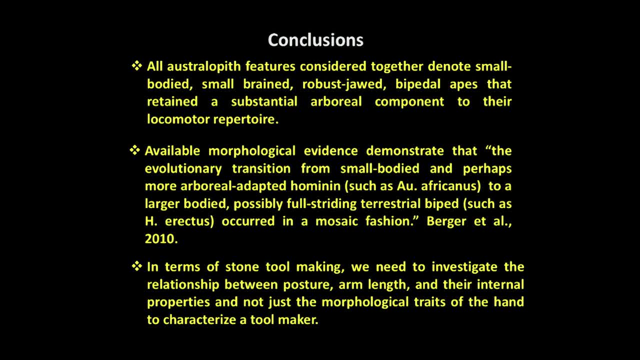 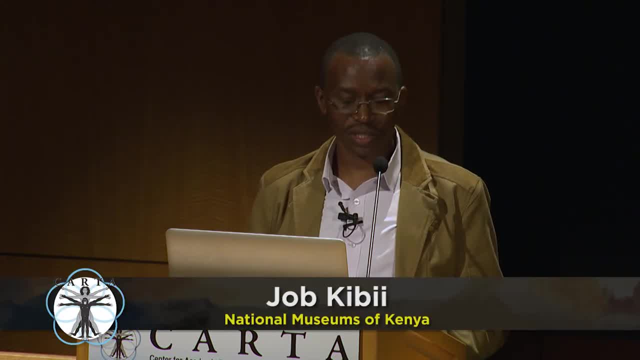 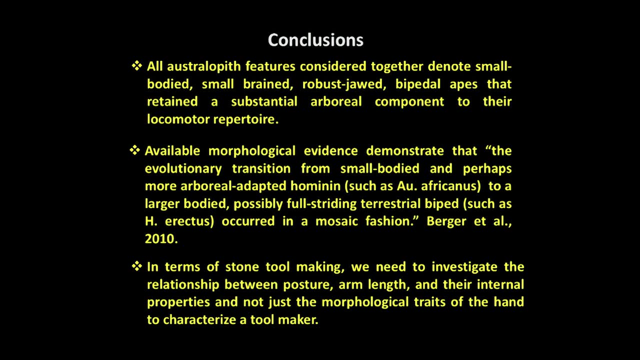 africanus to a larger-bodied, possibly full-striding terrestrial biped such as Homo erectus, occurred in a mosaic fashion. In terms of stone tool making, we need to investigate the relationship between posture, arm length and their internal properties, and not just the morphological. 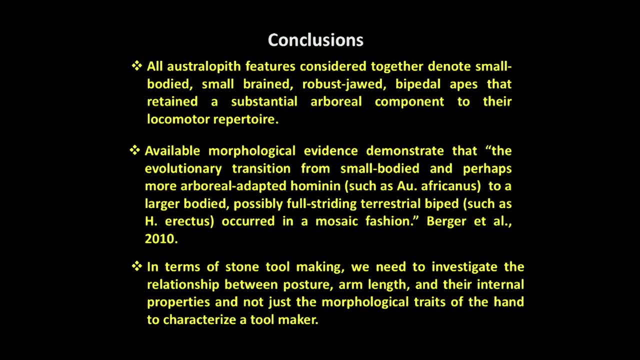 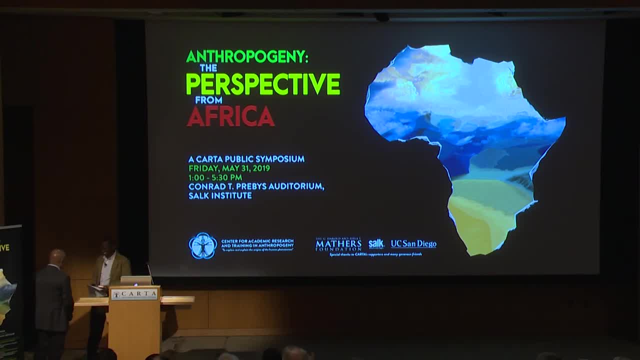 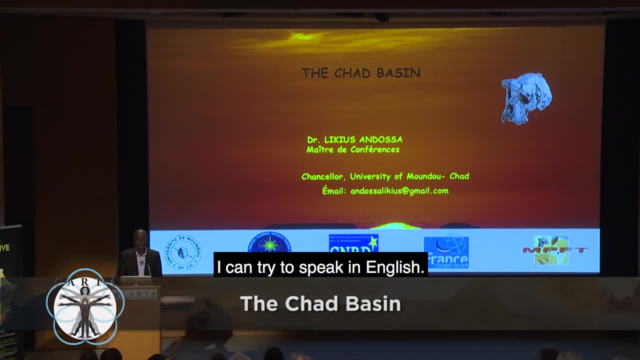 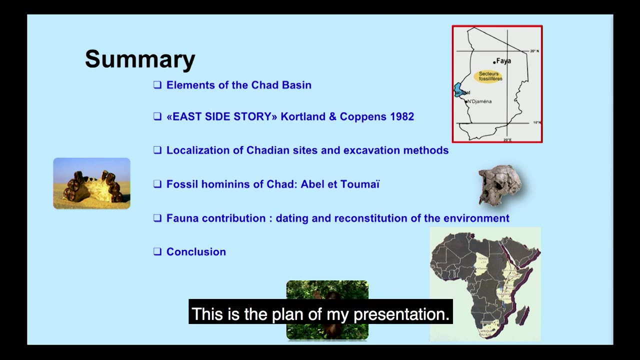 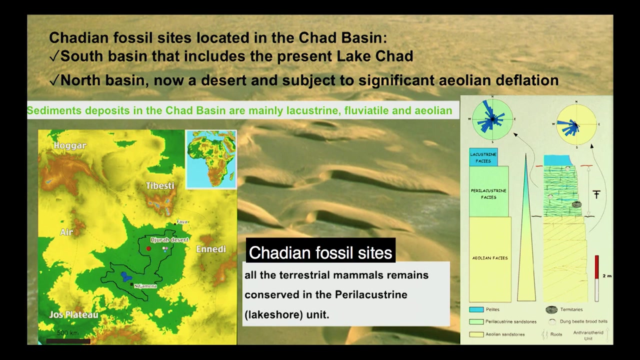 traits of the hand to characterize a tool maker. And with that, thank you. Good evening everybody. Sorry, my English is very bad. I can try to speak in English. This is the point of my presentation. Chaldean fossil sites located in the. 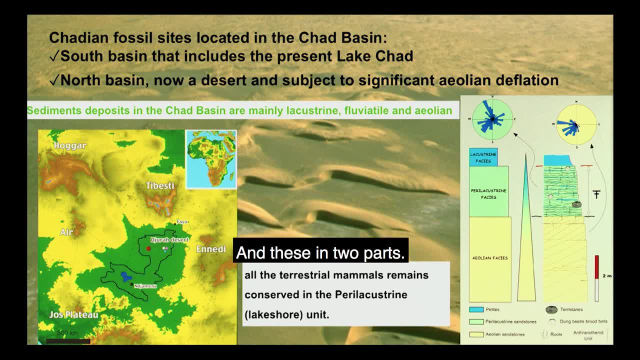 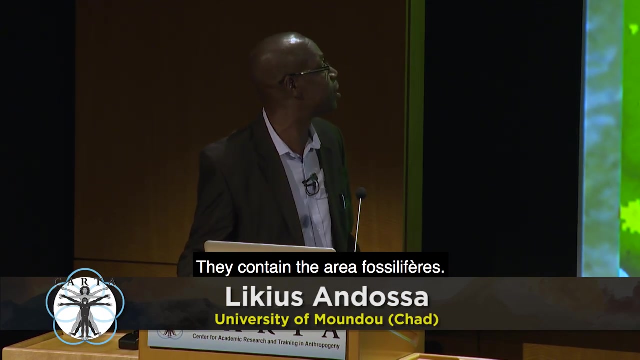 the Chad Basin and it's in two parts. The South Basin includes the present Lake Chad and North Basin now is desert and subject to syphian-aeolian deflation. They contain the aerofossilifer And sediment deposits in Chad, in Basin Chad. 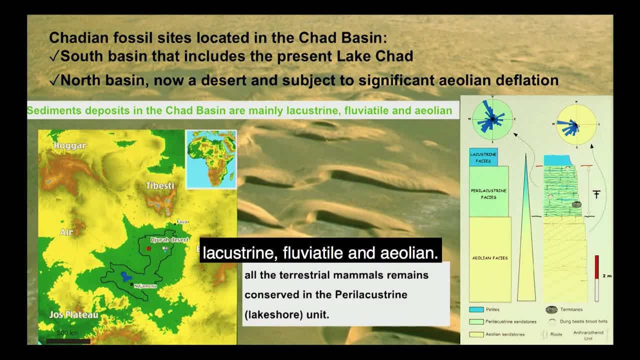 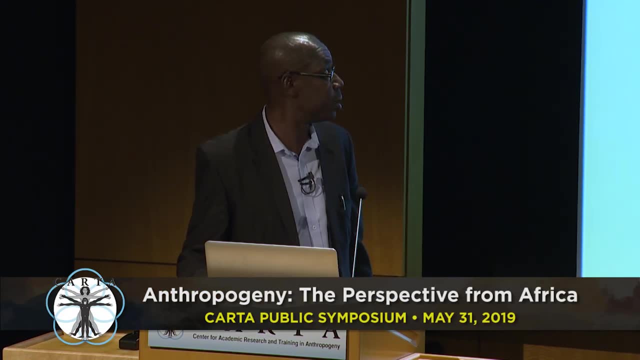 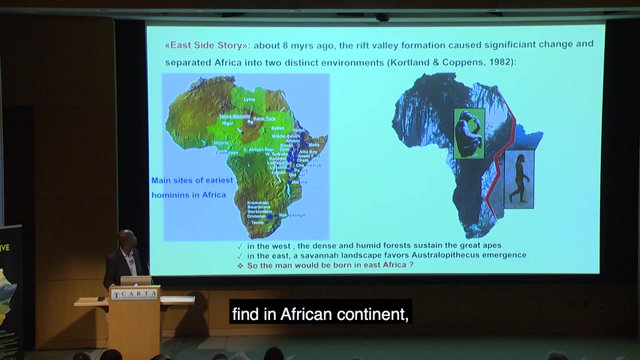 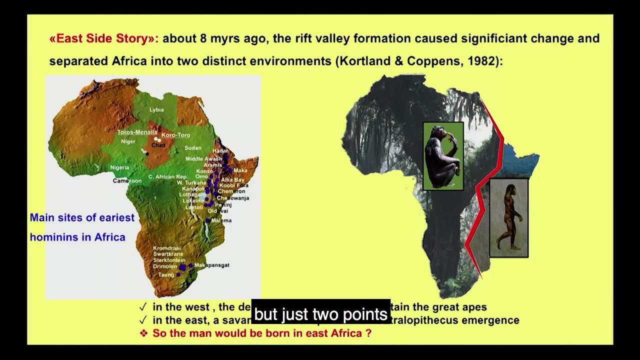 are mainly lacustrine, fluviatil and aeolian. All the terrestrial mammal remains are conserved in the peri-lacustrine unit And, as you know, most of all humans find in the Basin an African container. But you know just two points in Central Africa. 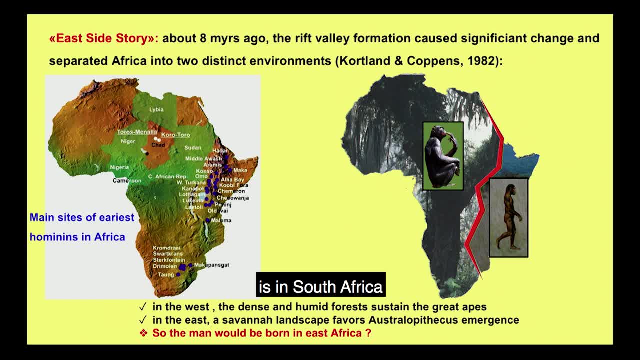 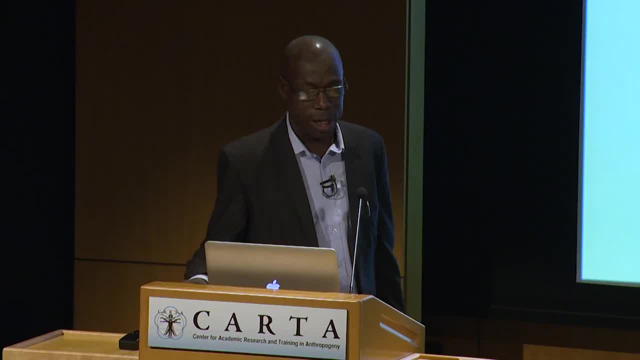 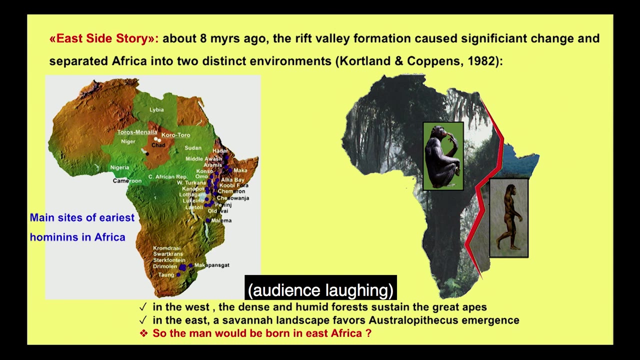 The most of part is in South Africa or in East Africa. This singular situation led some paleontologists to propose a scenario we call East-South Africa. The East-South Africa is a great story. This, according to this hypothesis, about eight million ago. 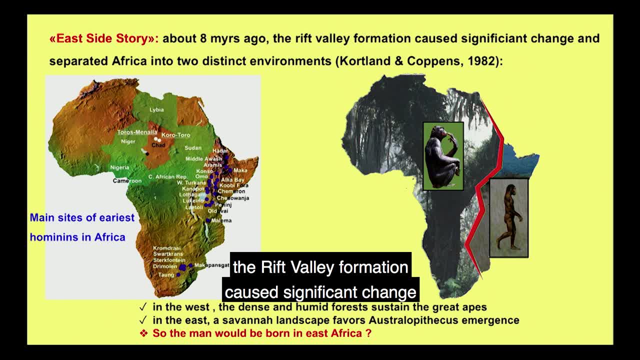 the rift valley formation caused significant change and separated Africa into distinct environment. In the West, the dense and humid forest sustains the great apes. In the East, a savanna landscape favors Australopithecus emergence. So the man will be born in East Africa. 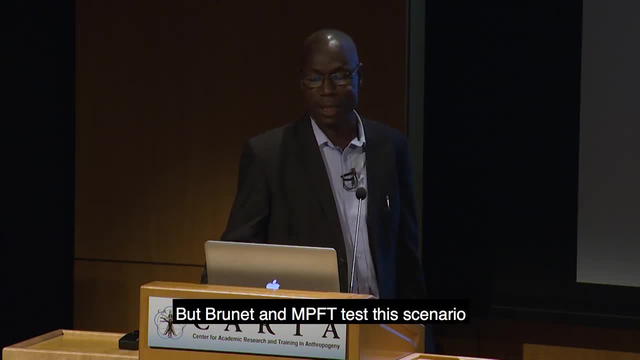 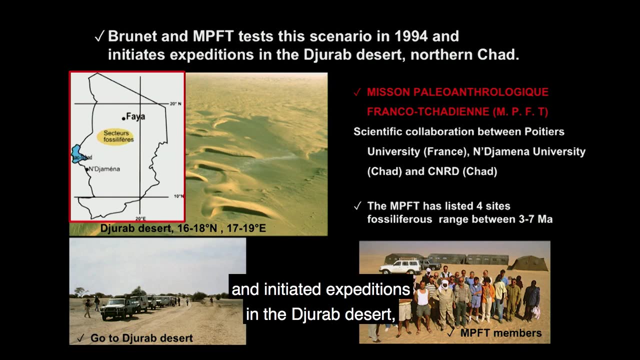 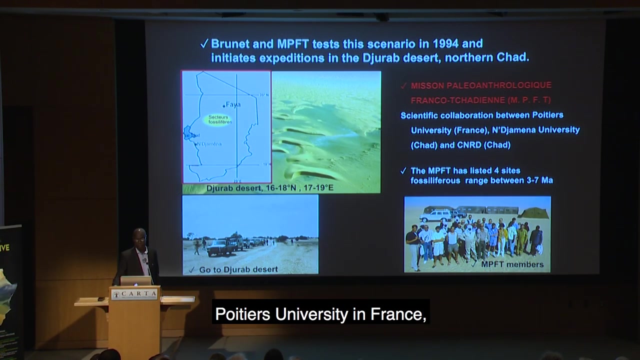 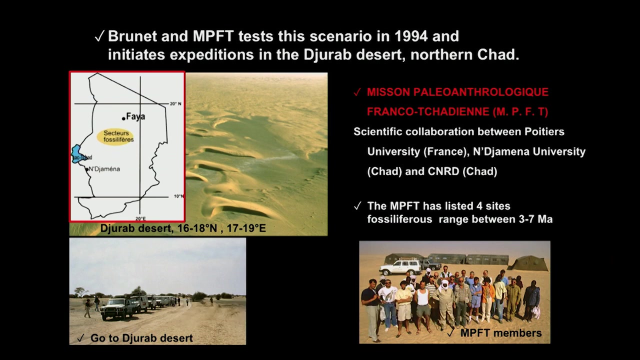 But Brunet and Mpefti tested this scenario in 1984 and initiated expedition in the Durape Desert, Northern Africa, The Zodiacal and Ch'at. The mission paleoanthropology Franco-Tiadian is a scientific collaboration between Poitiers University in France, Jamina university and Séniardé in Chad. 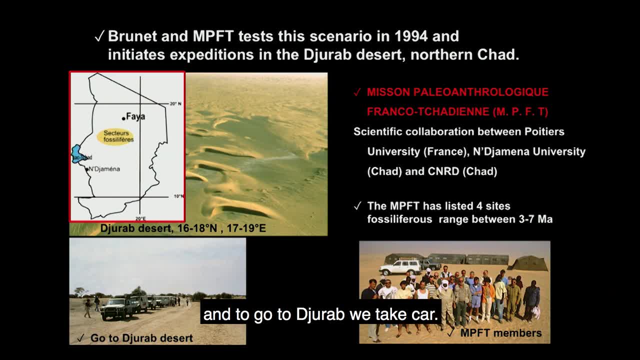 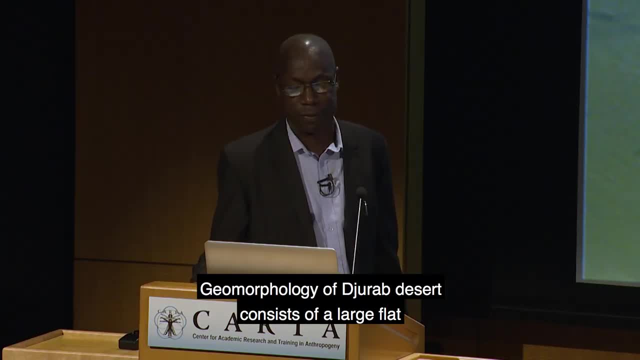 The Mpefti has listed for 6 fossil-fair range between three and seven million years, the area of fossil fuel. And to go to Djerab we take car. Geomorphology of Djerab Desert consists of a large flat. 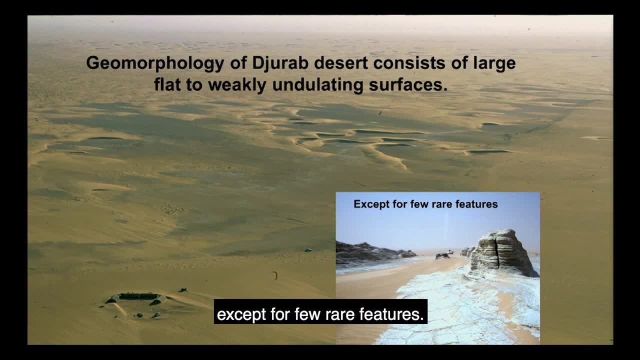 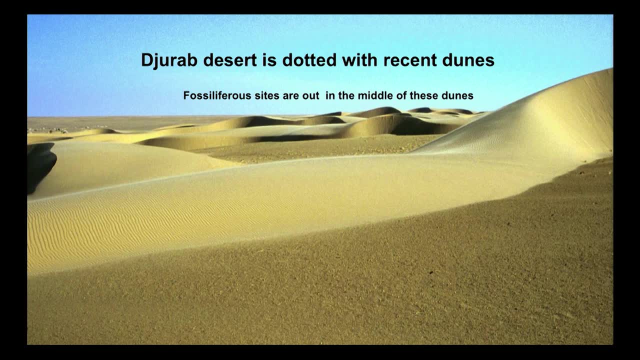 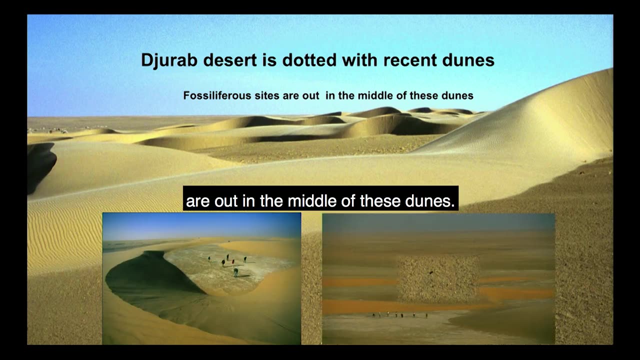 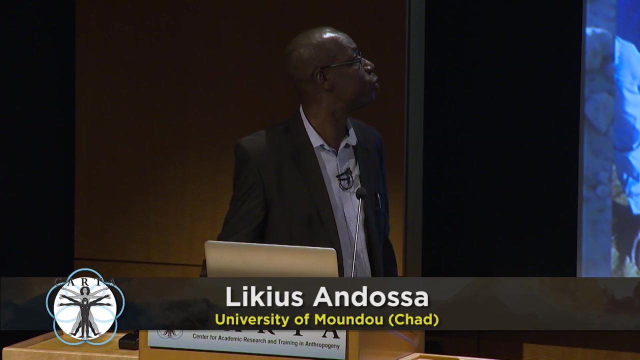 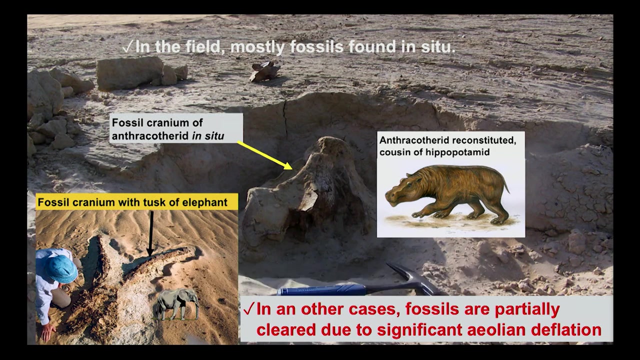 to wetly undulated surface, except for few rare features And Desert. Djerab is with recent June And fossil fuel are out in the middle of this June And the field mostly fossil found in situ, such as fossil cranium of Anthracoterid in situ. 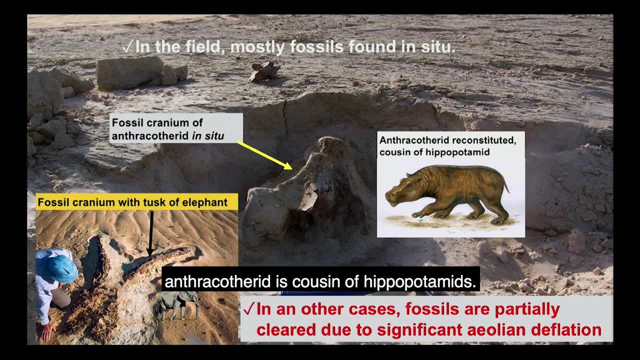 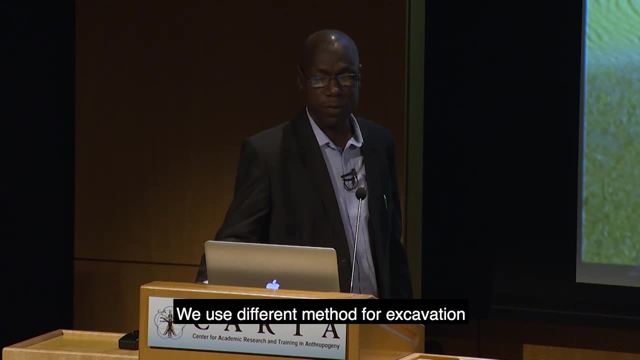 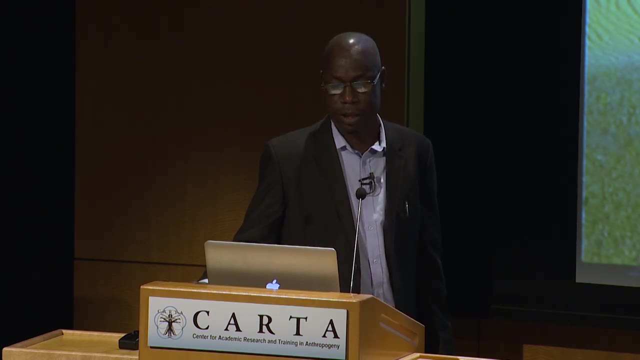 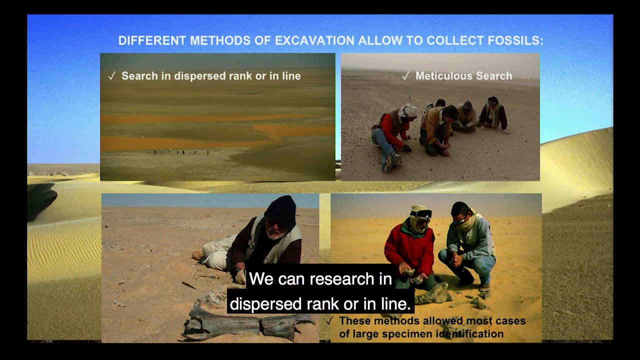 Anthracoterid is a cousin of Hippopotamids And other cast fossil are partially clearly due to significant aeolian deflation, such cranium with tusks of elephant. We use different method for excavation and always to collect fossil. We can research in dispersing line or in line. 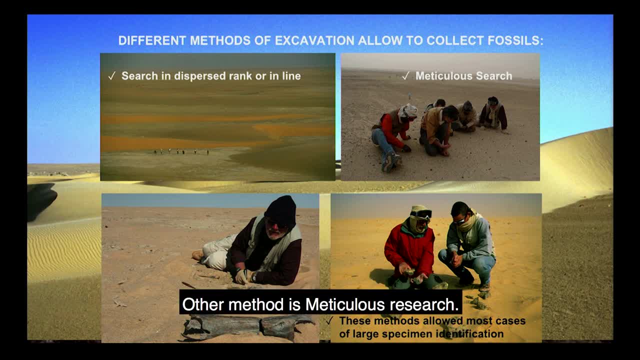 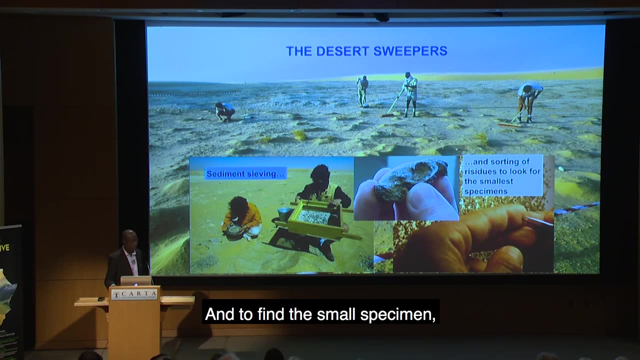 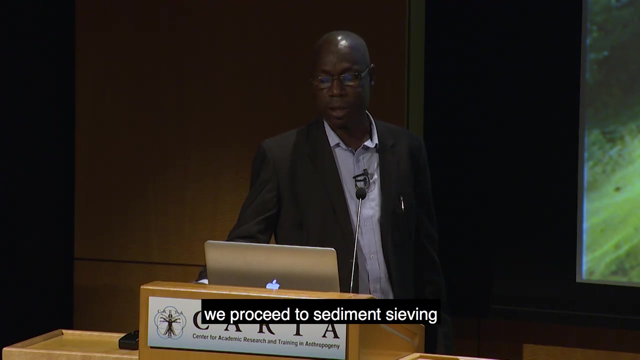 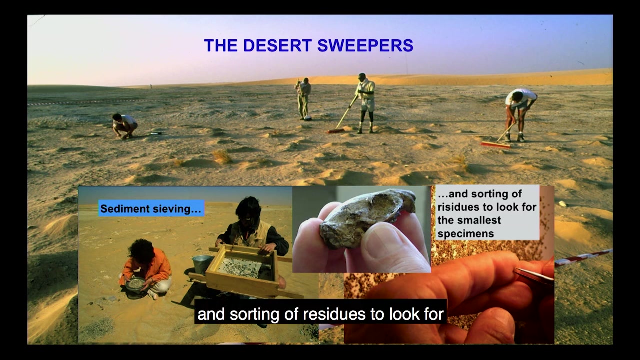 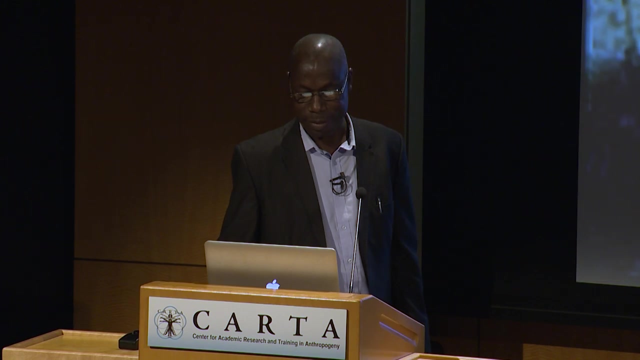 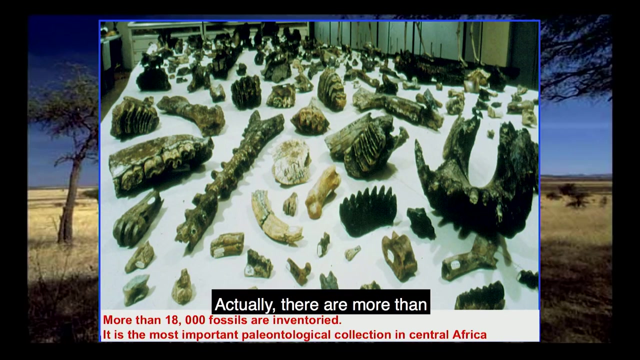 Other method is meticulous research. This method always most in case of large specimen identification And to find the small specimen. we transformed, we proceed to and we sorting of residue to look for the smaller specimen. The different method- Actually we are more than 18 fossil are inventory. 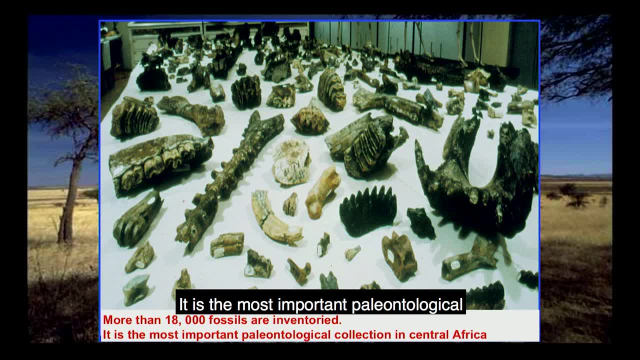 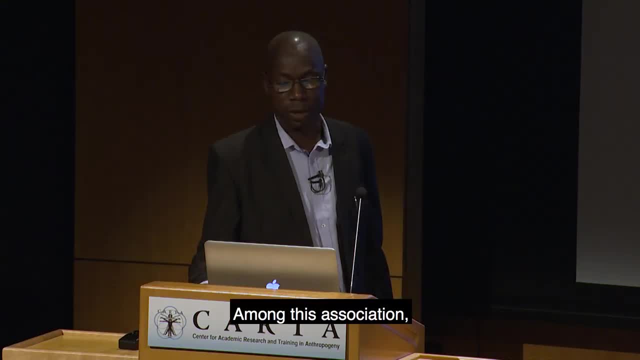 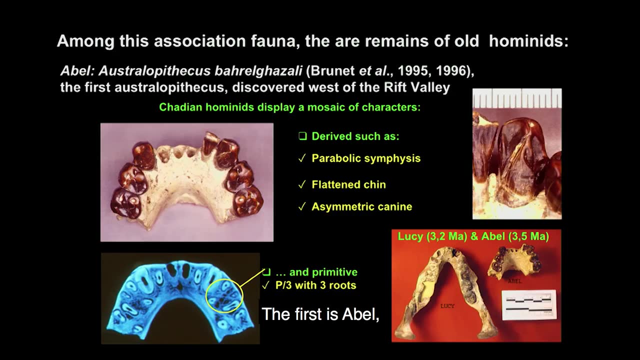 It is the most important paleontological collection in Central Africa. Among this association there are remains of all we need. The first is Abel. The name scientific is Australopithecus, But this is the first, The first Australopithecus discovered west. 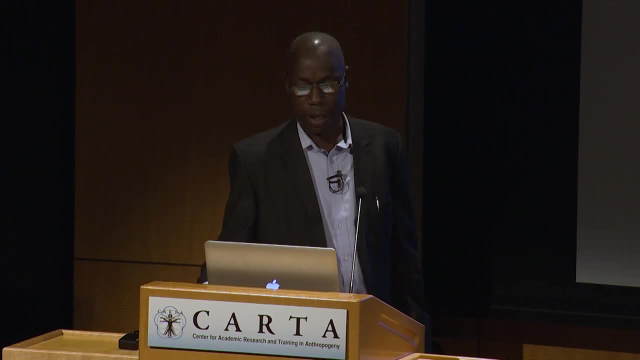 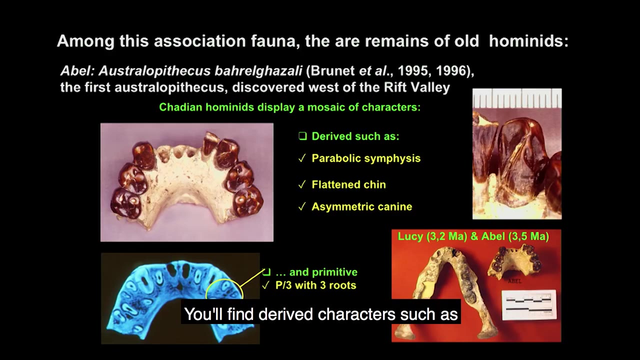 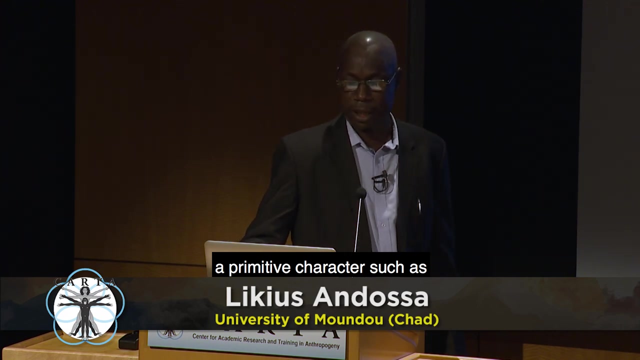 of the valley, Africa, Chardian omenis, display, a mosaic of character. We find there is character, such parabolic symphysis, flat net shanks, asymmetrical canine. And we find also a primitive character, such premolar with three roofs. 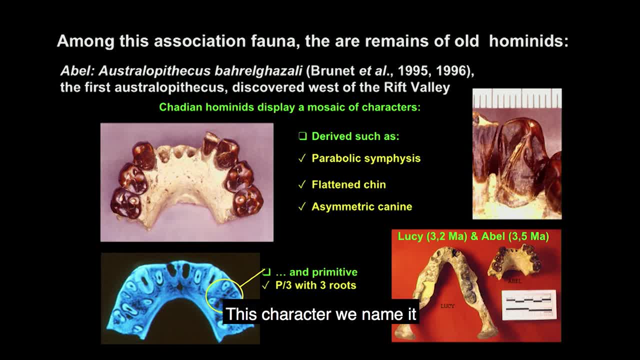 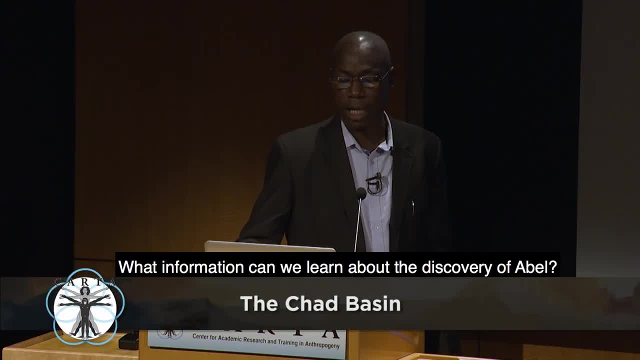 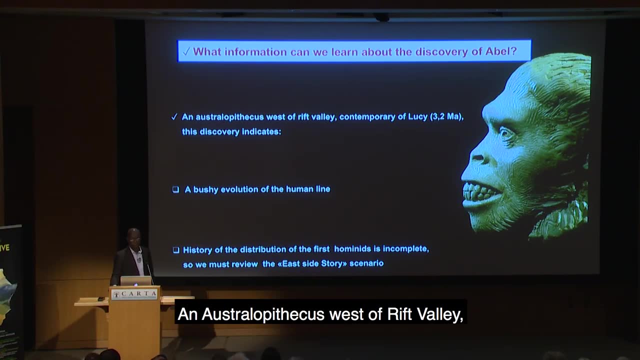 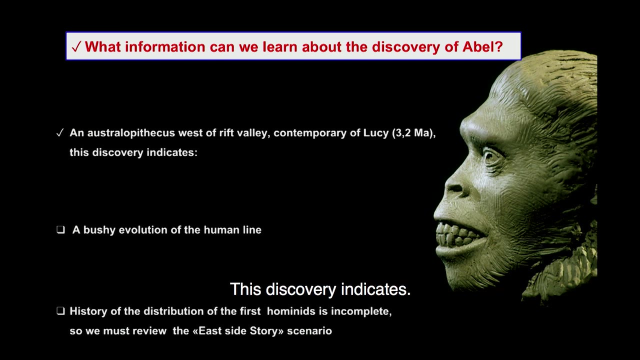 This character, we nominate a new Australopithecus, Bar Elgazali. What information can learn about the discover of Abel And the Australopithecus west of Rift Valley contemporaries of Luisi? This discover Indications? 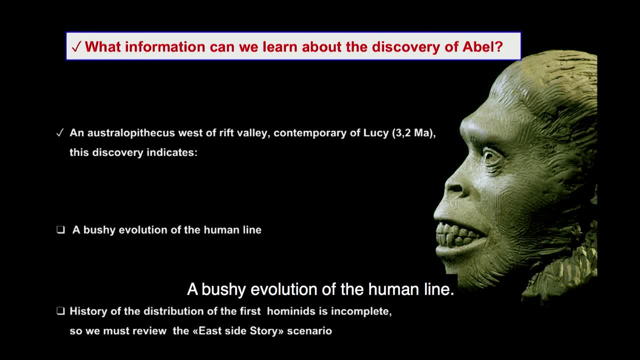 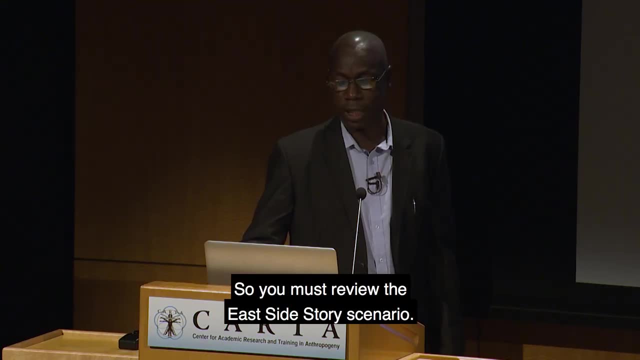 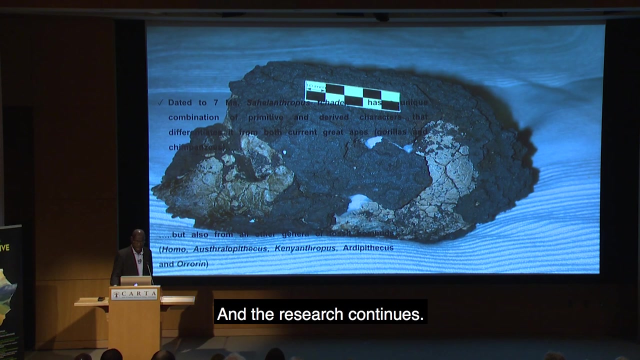 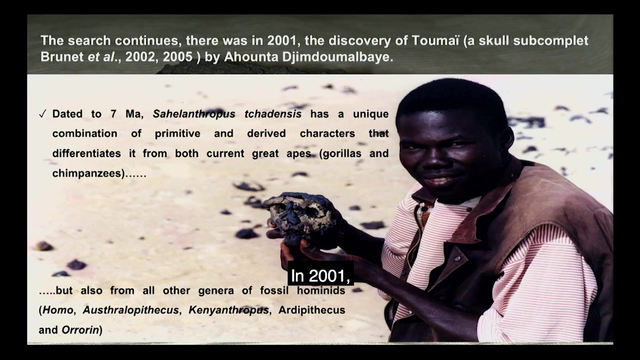 assets, a busy evolution of the human line. And second, the history of the distribution of the first is incomplete, So you must review the East Side Story scenario And the research continued in 2001.. We discovered another hominid who called Tumai. 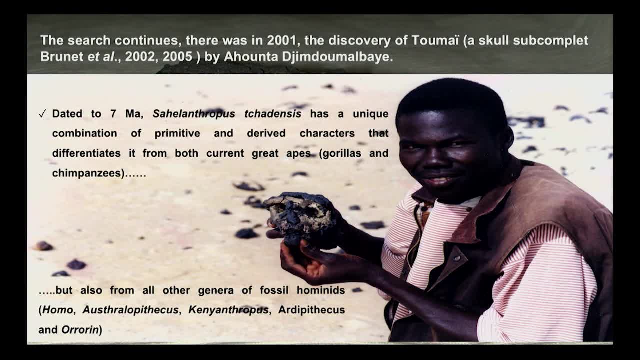 That is, to 7 million. The silent tropical chameleons Have a unique combination of primitive and derived characters that differences it from both current great apes, Gorilla and, but also from all other genera of fossil hominids, Homo. 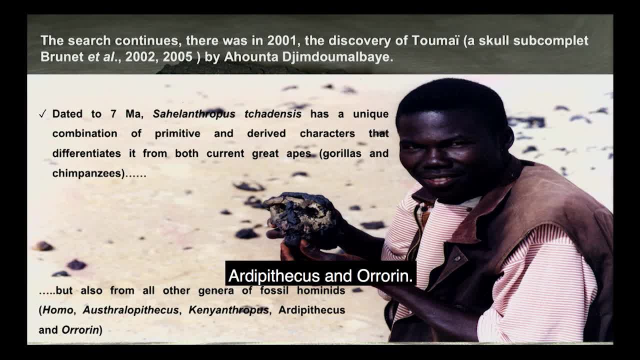 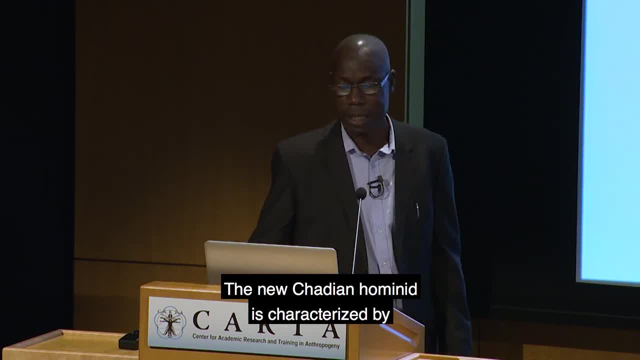 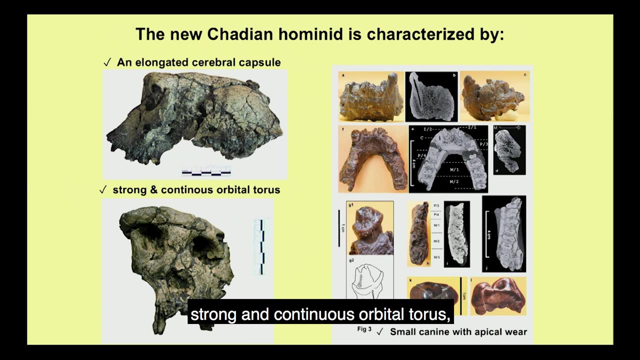 Australopithecus, Kenyantropus, Ardipithecus and Aurorin, The new Chadian hominids, Is characterized by an elongated cerebral capsules, strong and continuous orbital torus. He have also small canine with apical wire. 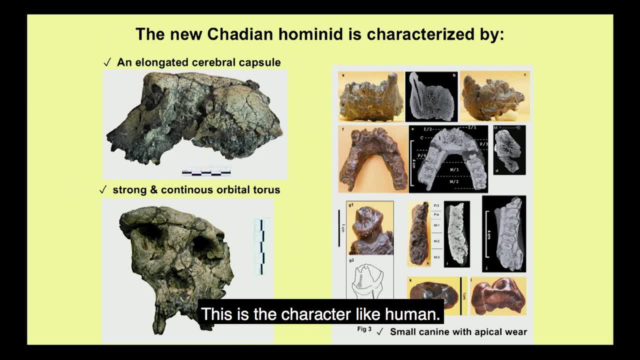 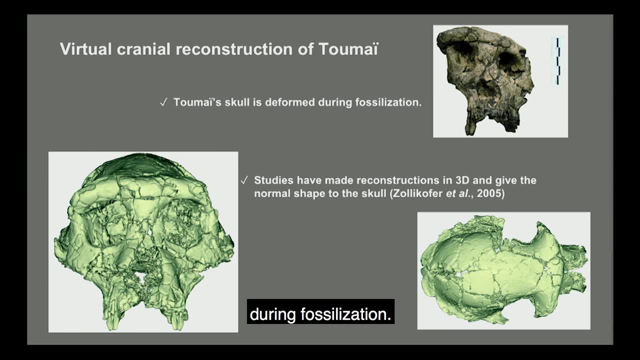 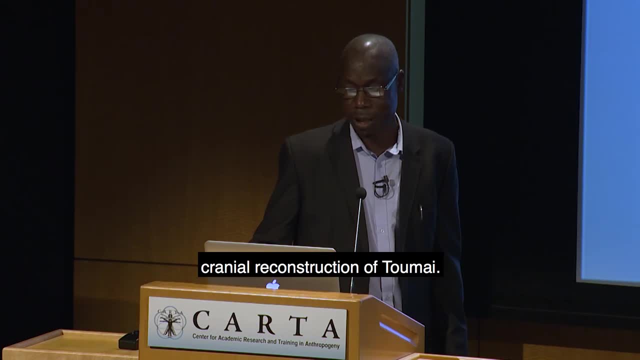 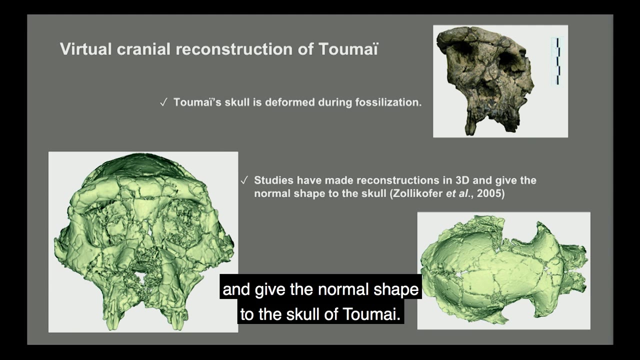 This the character, like human And Tumai school is deformed during fossilization. We do study for virtual cranial reconstruction of Tumai A study. have made reconstruction in three dimension and give the normal shape to the school of Tumai. 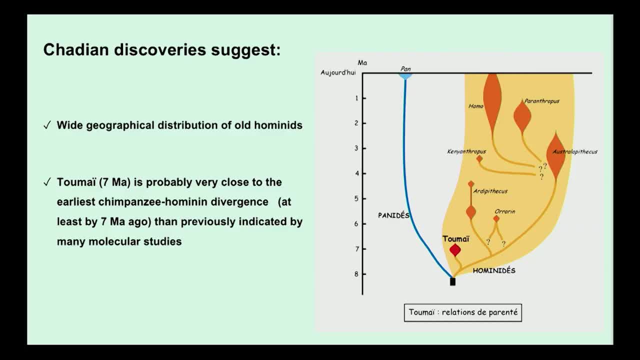 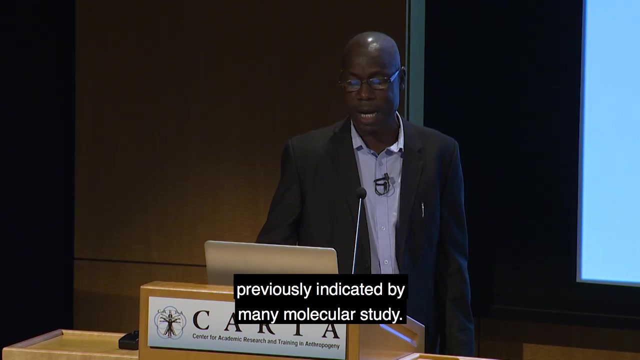 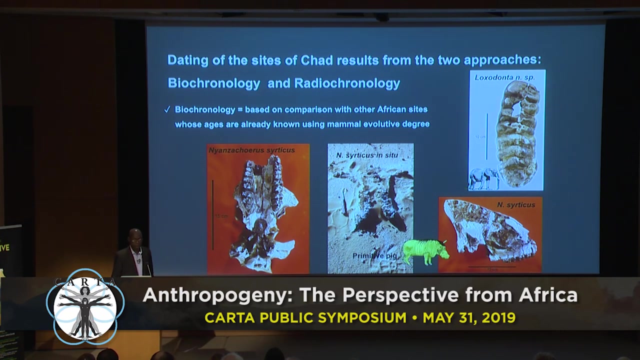 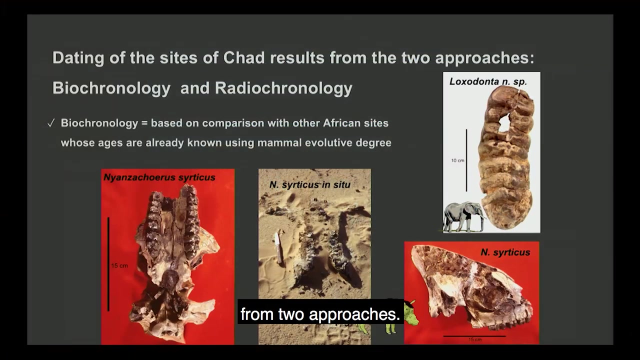 Chadian discover suggests: Primo, what geographic distribution of old hominid "the set of Chadian from two approaches: biochronology and radiocronology. Biochronology is based on comparison with other African sites with age are early. 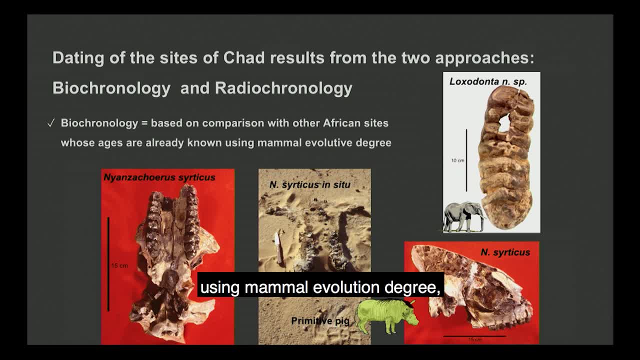 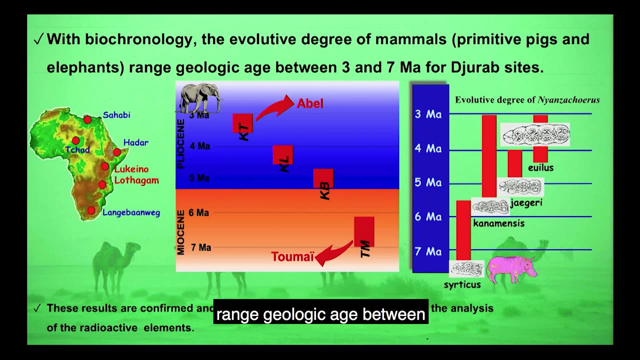 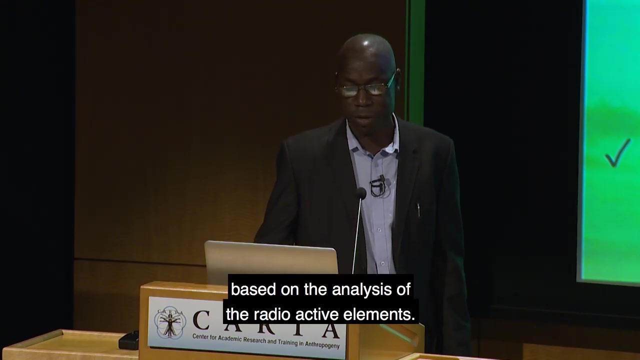 dinos. using mammal evolution degree, notably, and primitive peaks, Radiochronology. the evolutive degree of mammal range between 3 and 7 million for durable seeds. These results are confirmed and refined by radiochronology based on the analysis. 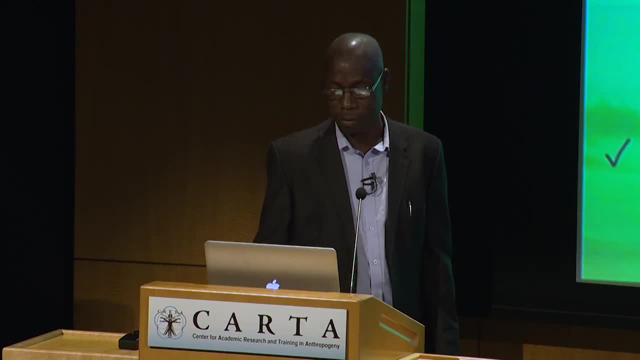 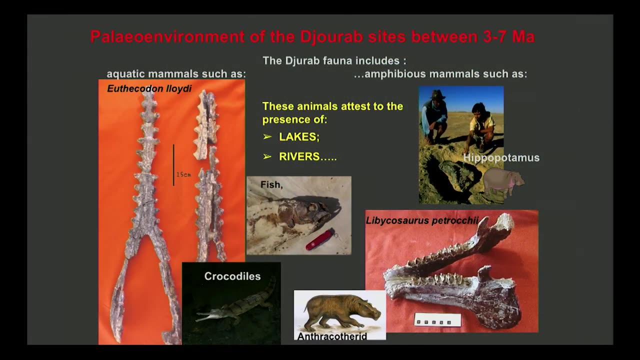 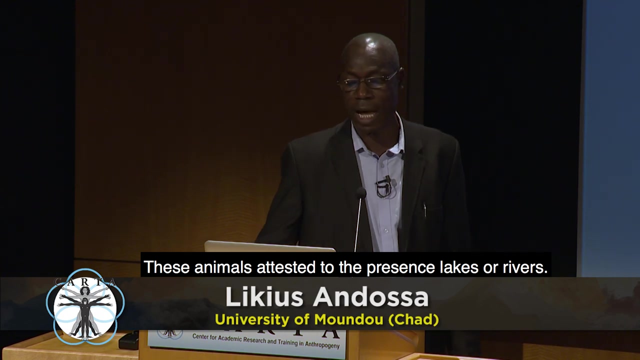 of the radioactive elements. We also do reconceive of paleoenvironment of the durable seeds. The durable seeds include aquatic mammals such as crocodile fish and amphibious mammals such as hippopotamus, and These animals are tested to the presence of lag or river. 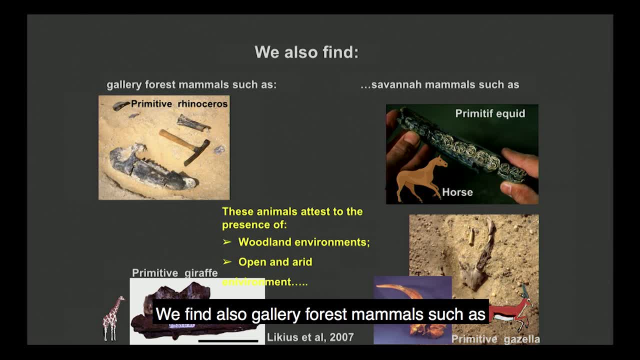 We find also gallery forest mammals such as primitive rhinoceros and primitive giraffe. We find also savanna mammals such as echids and primitive gazella. These animals test the presence of woodland environment or open and arid environment. Different methods of analysis of the disease. 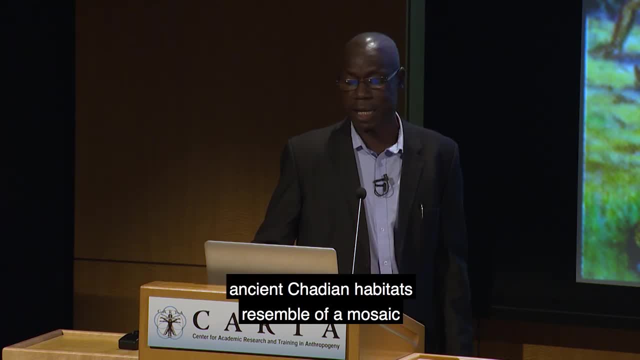 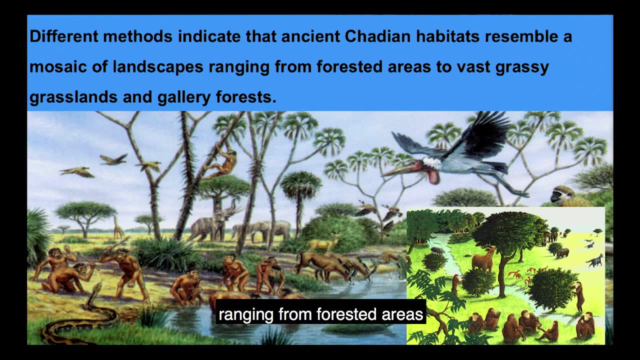 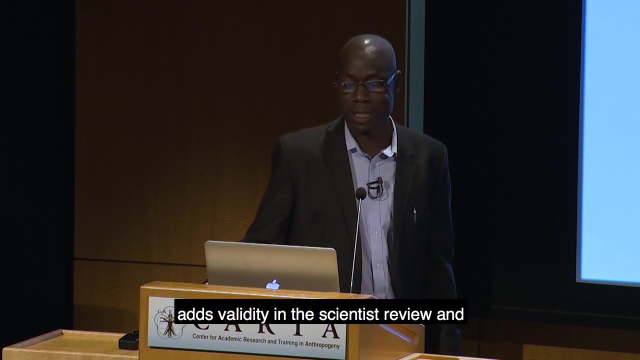 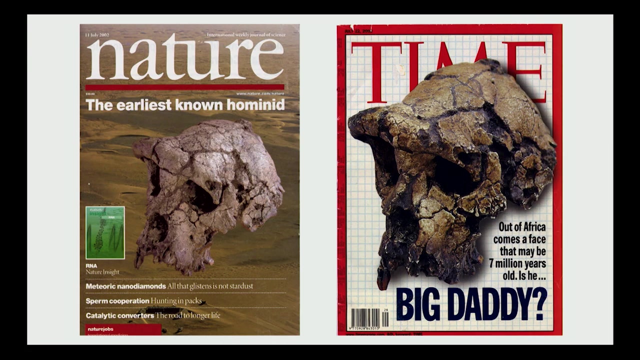 and the method indicates that ancient Chadian habitat resemble of a mosaic of large carpens ranging from forested high rise to vast grasslands and forest gallery. All of these results are valid in the scientist's review and We will get it by other journal. 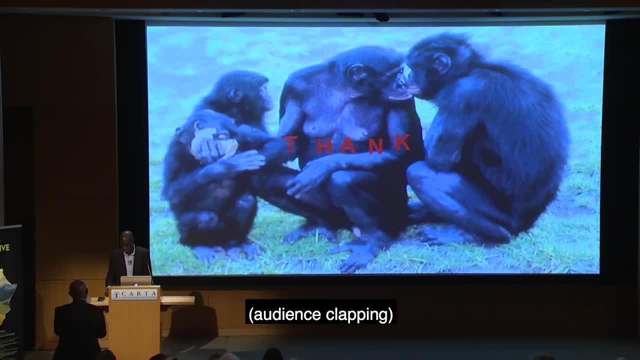 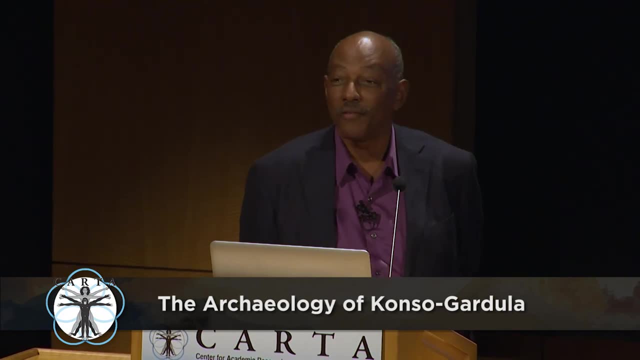 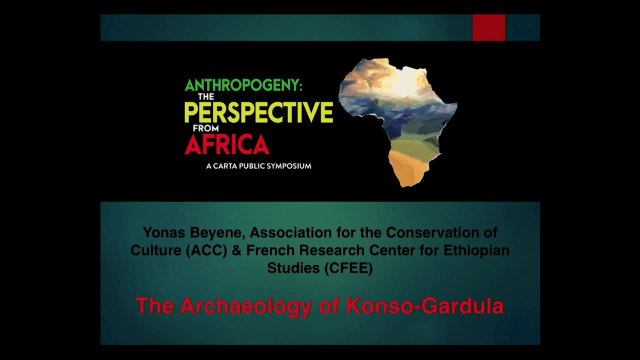 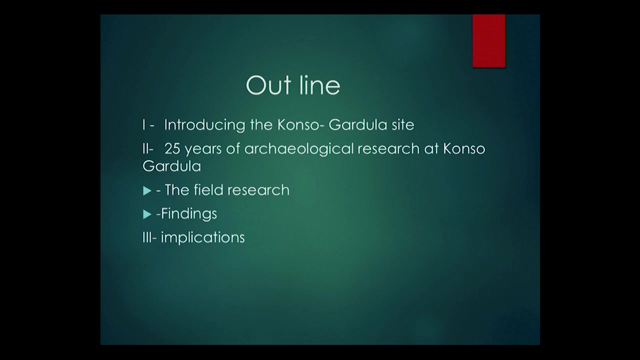 Thank you. Good afternoon, ladies and gentlemen. I'm very happy to be here and present the archaeology of the Konso-Gardula sites in this institution. My speech, My speech outline, will be: first: I will start by introducing the Konso-Gardula sites. 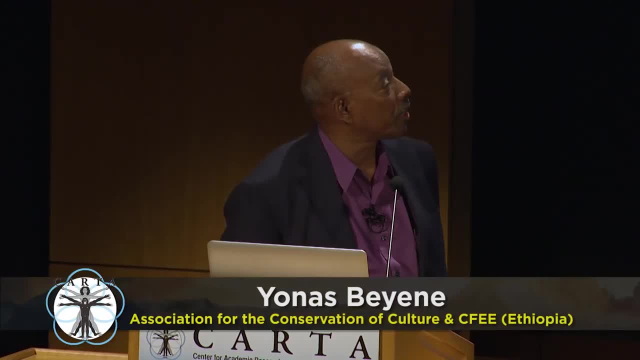 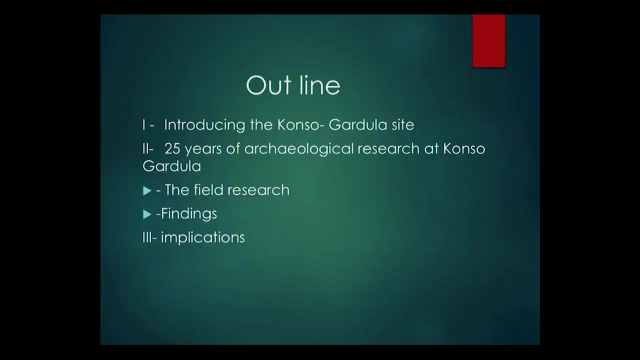 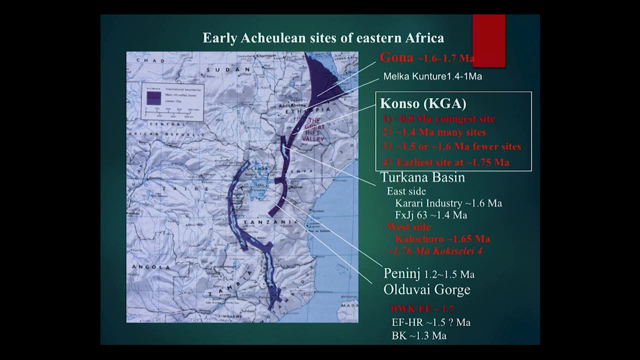 Then I will go through the 25 years of archeological research at Konso-Gardula, focusing on the field research and findings, and I will touch upon some of the implications. What you see here is map of East Africa and, as the Konso-Gardula site is well known for its Acheulean 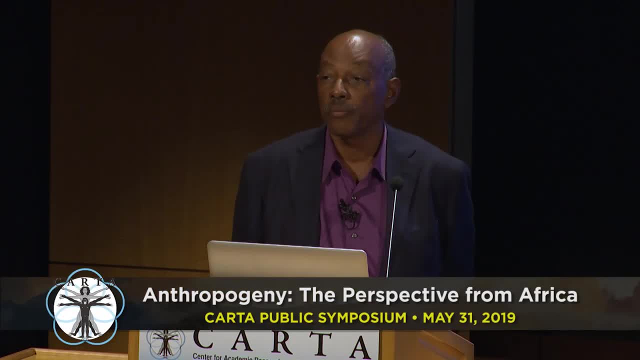 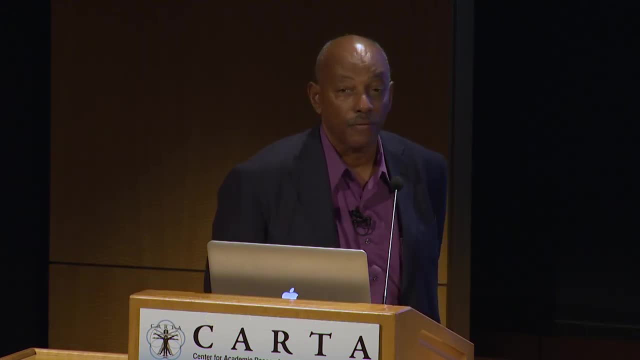 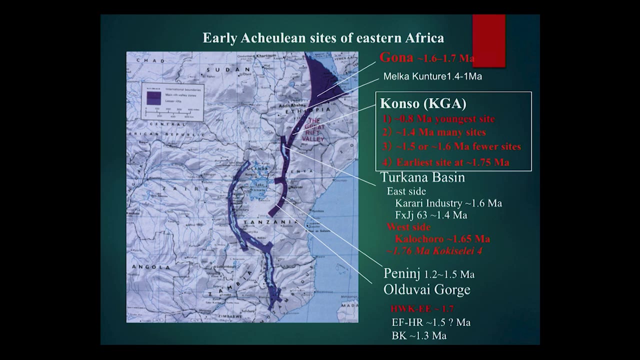 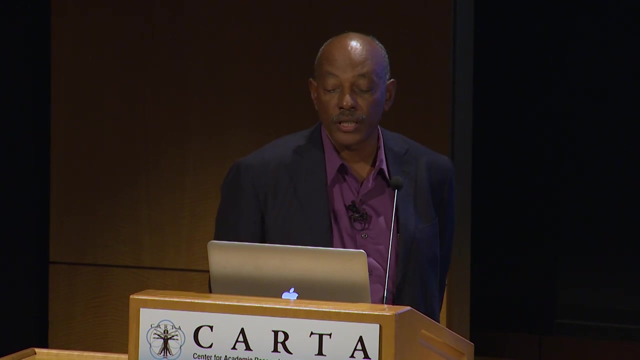 occurrences, meaning stone tools made on large flakes, shaped on large flakes, which appeared as of 1.75 million years ago. My focus will be on sites that are known for what they have in the representing this technology. Konso-Gardula is one of these sites. 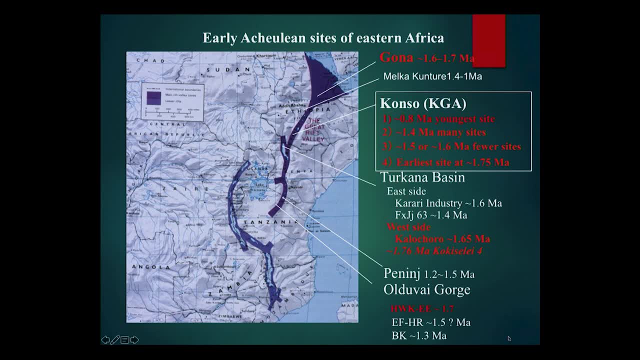 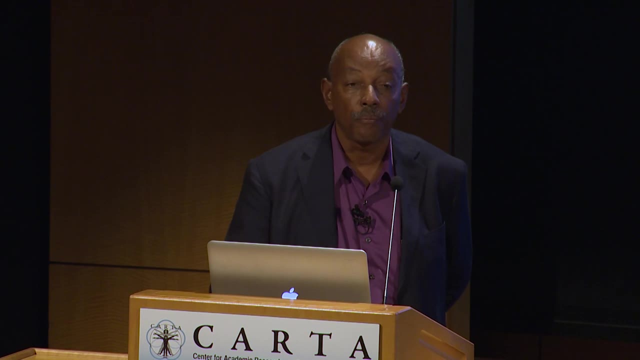 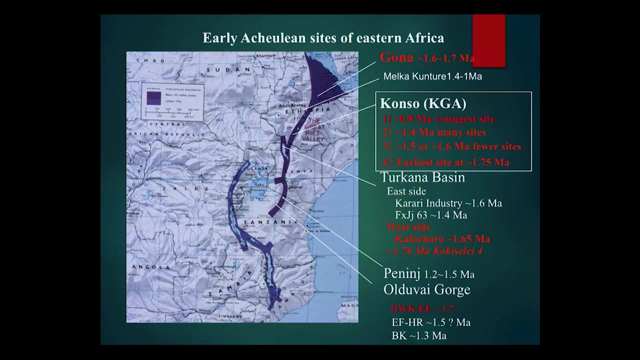 Together with the Kokasele sites, which is located here in West Turkana. Konso-Gardula is the oldest Acheulean site, with hand axes that are dated to be 1.75 million years old. And it's not only these sites, but there are also other sites. 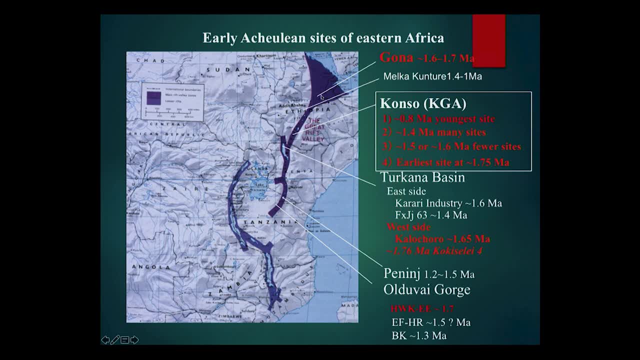 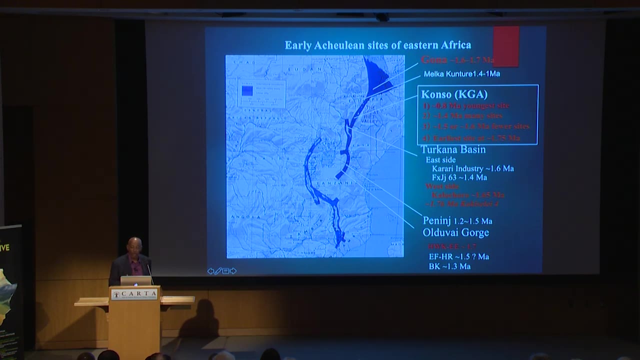 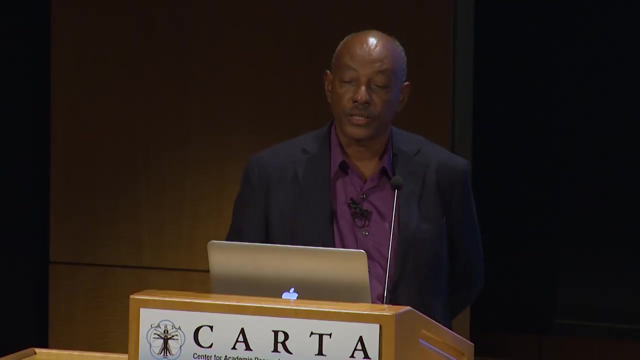 in East Africa. Further north is the lower Awash Valley in Ethiopia and in Turkana Basin in the Olduvai Gorge. we have many other sites, But all are not as old as these windows that we have. This is the distribution of the sites. 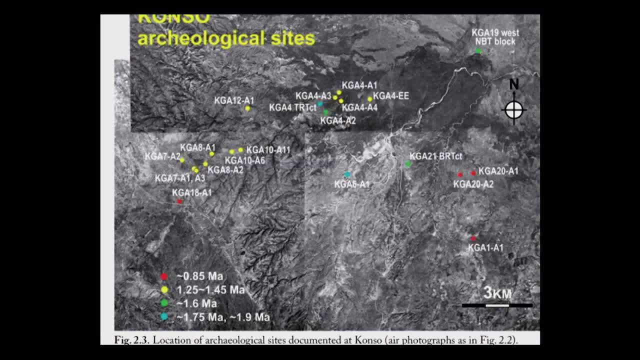 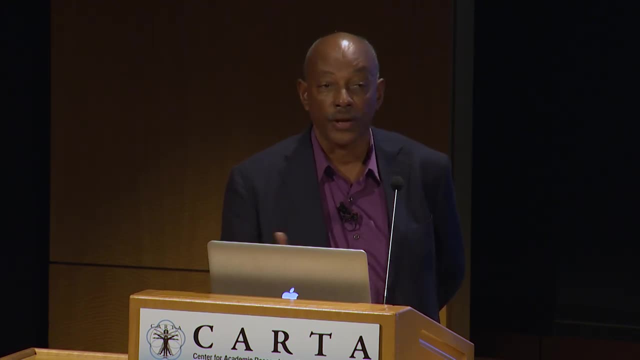 within the Konso-Gardula. We discovered this site, the Konso-Gardula, in 1991 in a project that was run by Dr Brohani, my colleague here. We were working together in those years. We were surveying the whole rift of the Ethiopian part. 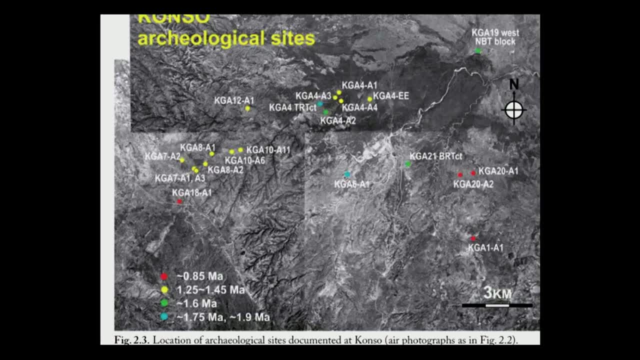 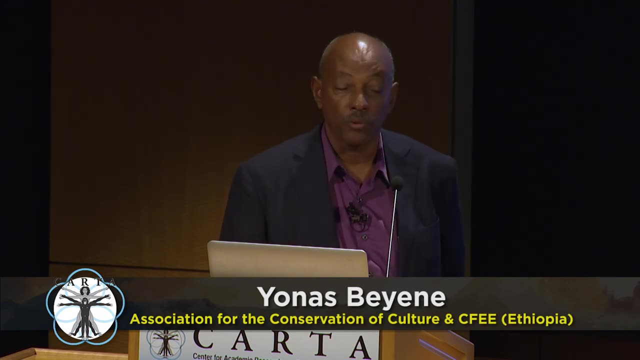 of the Rift Valley And we discovered several sites. One of these sites happened to be the Konso sites, And this site was a focus of attention for people who were interested in that period, the period between 800,000 and 2 million years old. 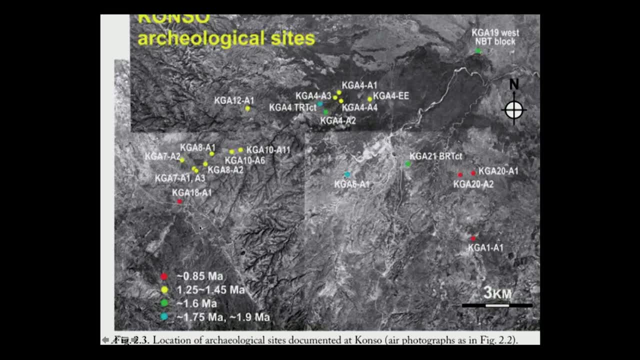 As you can see here, the oldest sites at Konso-Gardula, dated to around 1.75 million years ago, are very rare And it's only one site that we have, And when we come to around 1.6 million years, we have also few. 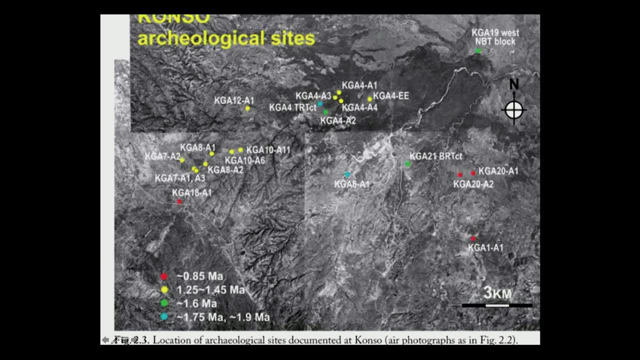 few sites, but as of 1.45 million years ago- the yellow shows us the distribution of sites- The Acheulean becomes more abundant And by around 850,000 years ago we have more Acheulean sites everywhere. 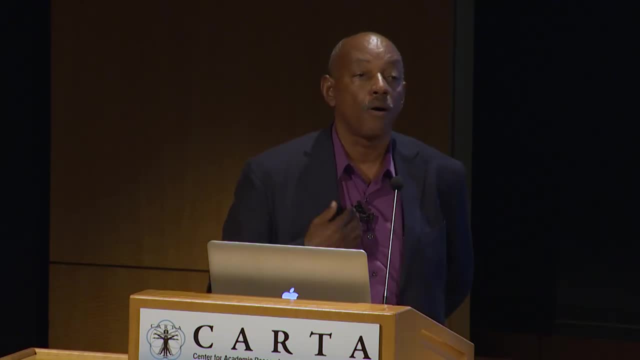 So not only Acheuleans that we have in Konso, but also older one technologies are also represented in sediments which are older than 1.75 million years old And all the way to 1.5 million. Here you have a composite stratigraphic section. 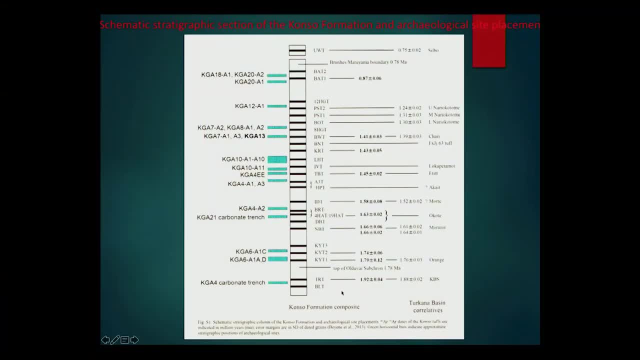 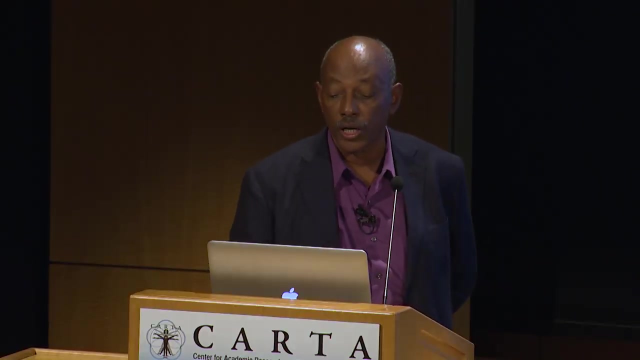 of the Konso site. This section represents 200 meters thickness of sediments, which has about 30 tough layers- the fascious layers- which were datable, And around 13 of these were dated- Radiometrically dated, And they were also correlated with already dated tough 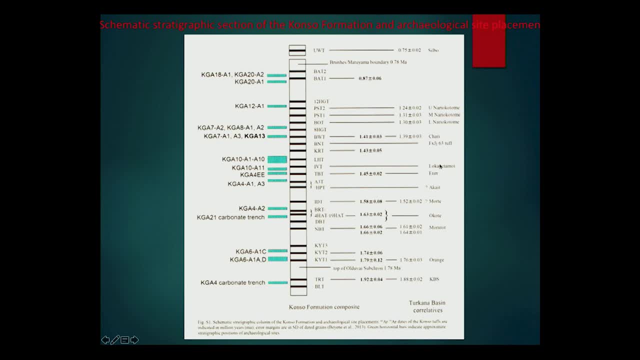 tough layers on the in the Turkana Basin. So we have archeological occurrences from the lowest here at around 1.92, which are represented by old one technology, meaning simple core flake techniques, But the oldest Acheulean staunters represented by handaxes. 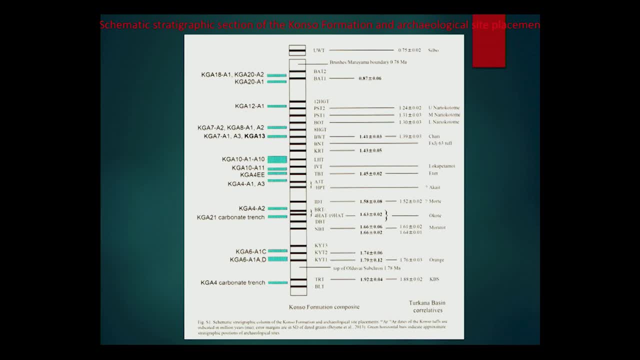 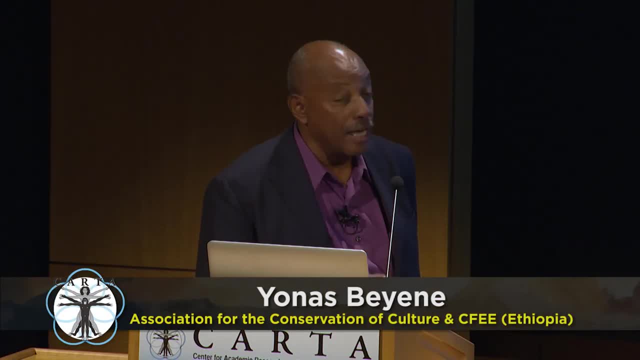 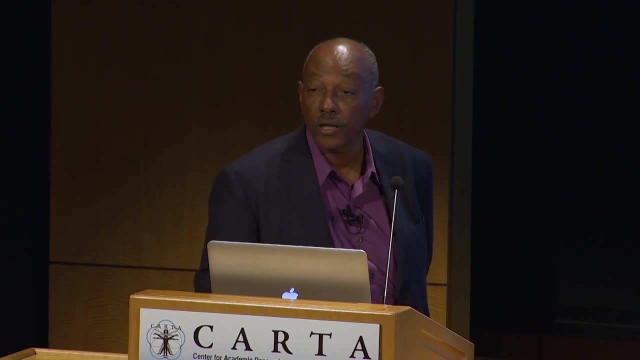 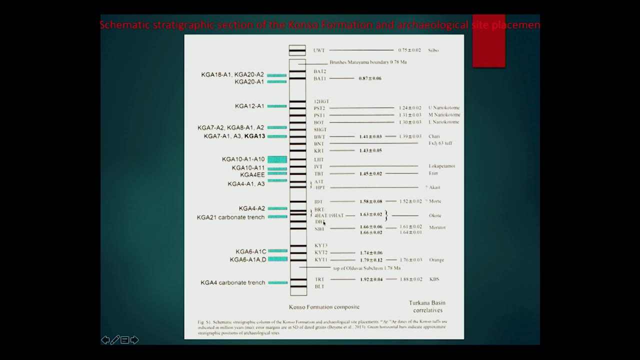 And this age is matched only by the sites that are found in Kokoseli in Western Turkana. As we go higher in the stratigraphy by around 1.63 million years, we have another important Acheulean site, meaning a site with abundant handaxes. 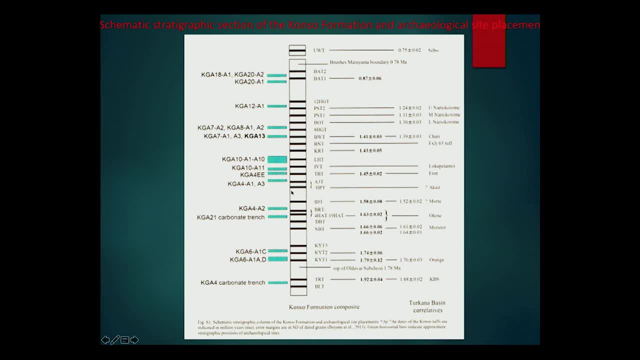 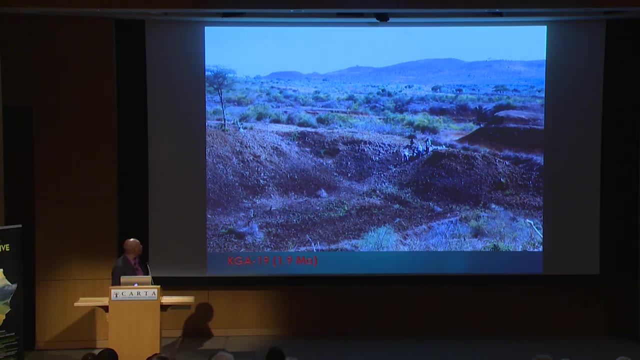 But the sites are very. it is only a single site But as of around 1.45 million years, we have the number of sites that increases and the technology also refines through time, as we'll be looking through. This is to show you one of the sites. 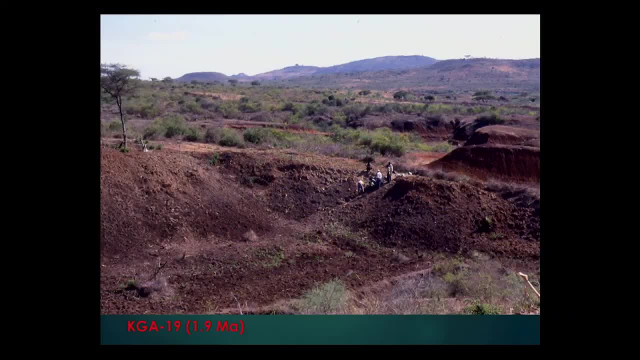 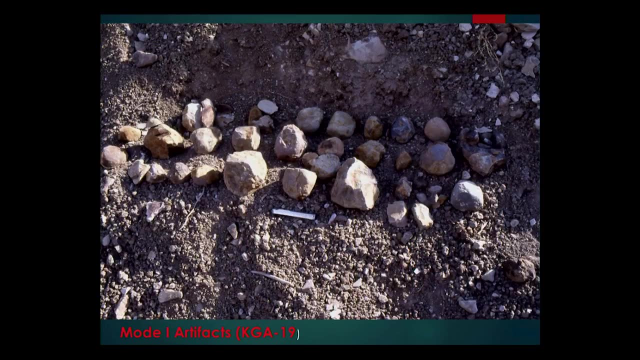 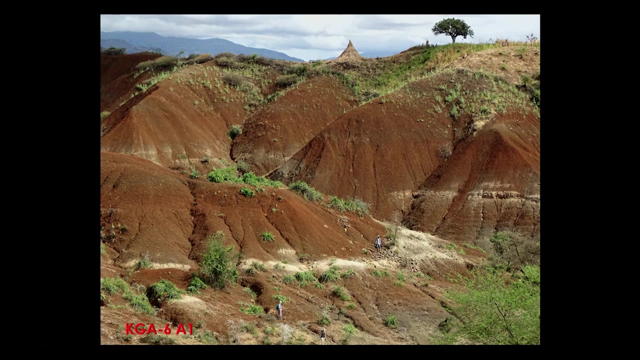 the older one, site dated at 1.9 million years, a site called KJ19, and the older one. artifacts represented- Although an artifacts represented there are, as you see here- are represented by the cobbles and flakes. This is another site which is dated. 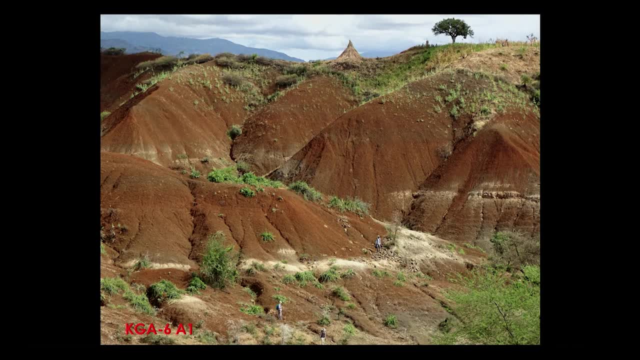 the site that is dated at around 1.75 million years ago, which we call KJ 6A1. And what you see here are two tufts here. Here you see two tufts. The archeological excavation is conducted here. 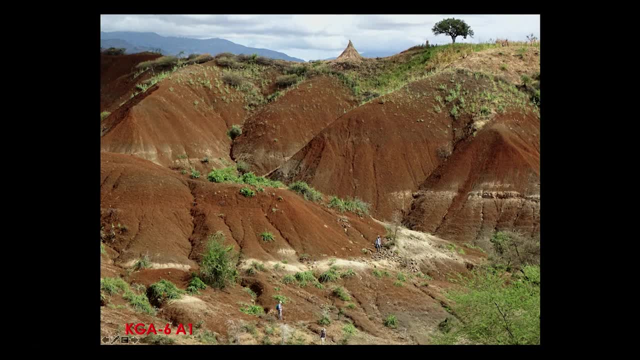 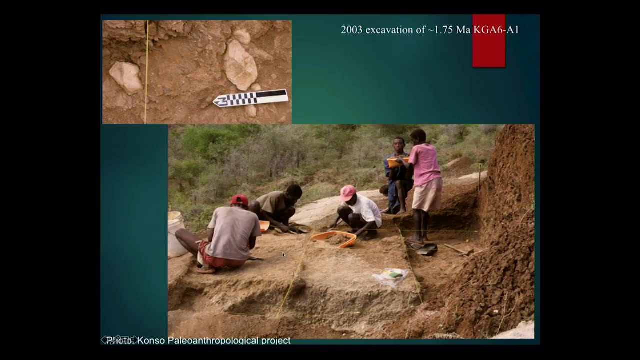 And the tufts. the upper tuft that you see is dated to 1.74, that is the KYT 2 tuft And this is the excavation And, as you can see, up there we have hand axes made on large flakes. 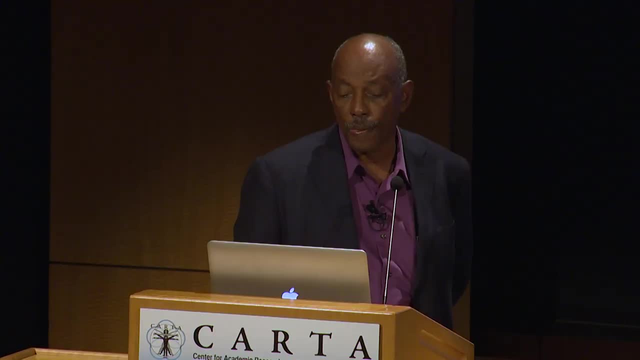 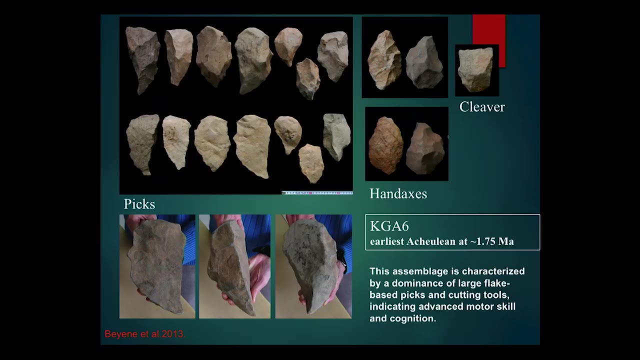 discovered in situ through excavations And the assemblage as a whole. when you look at it it is- you can see that it is flake-based. You see large flakes. This is the ventral of the. this hand axes and peaks. 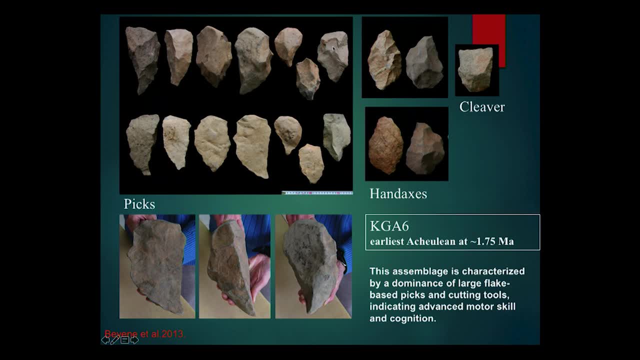 And shaping is minimal. And we also find peak forms, peaks, large peaks made on large flakes. So, as you can see here, the shape is not. the shape of hand axes is not well attained and shaping is not that great as other Acheulean hand axes. 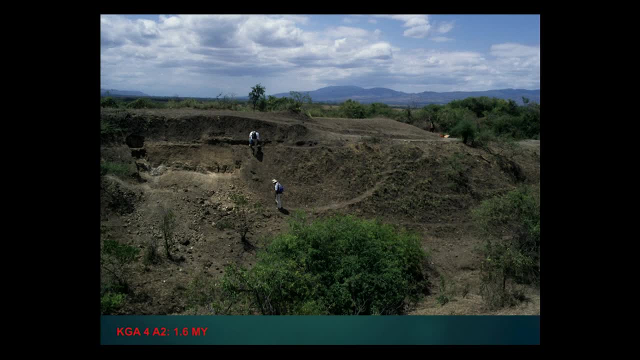 This is the second oldest site that we have at KJ 4A2,, dated at 1.6 million years ago. You have here the hand axe, tuft, and the archeological layer is just you see, and the archeological layer is just above. 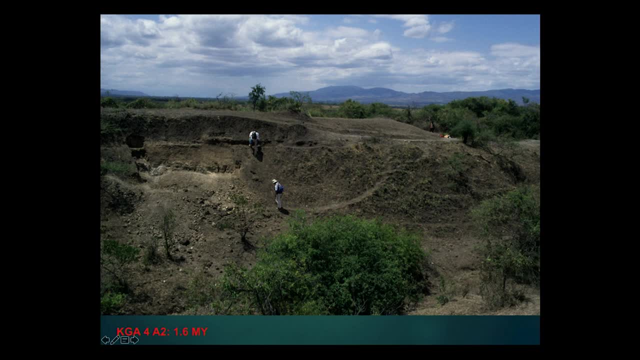 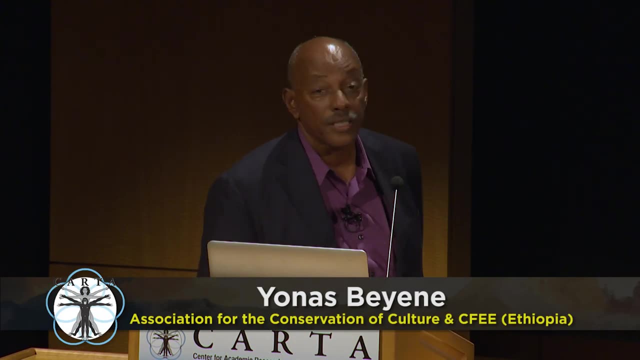 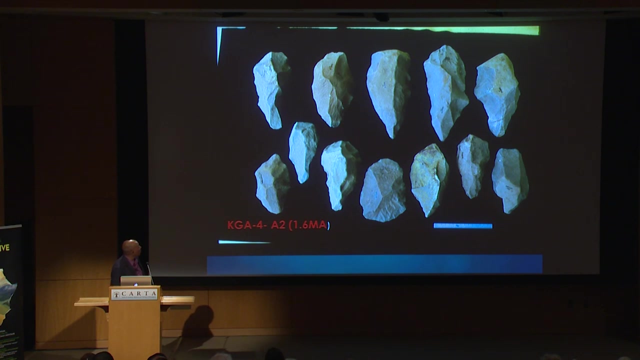 the hand axe tuft and what we our excavation was conducted just here because our burden on this site was higher, And the artifacts that were the Acheulean hand axes that were retrieved from the KJ 4A2 look like this: 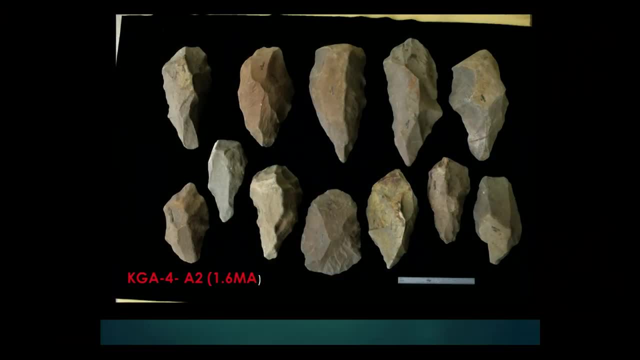 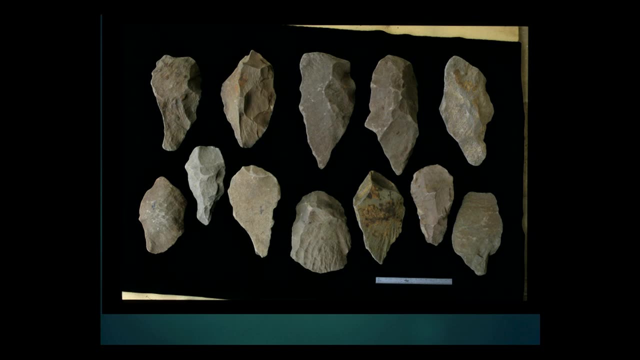 They are better shaped than the ones that we saw at KJ 6A1.. And we see again, And we see again all these hand axes shaped on, made on large flakes detached from mega cores. Big boulders were used as a core. 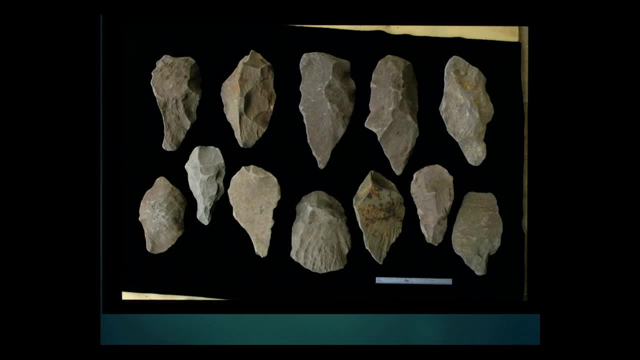 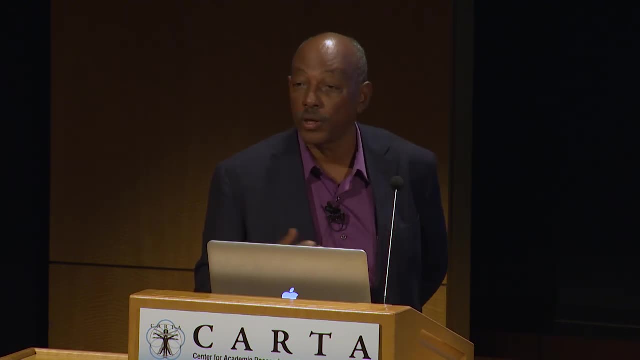 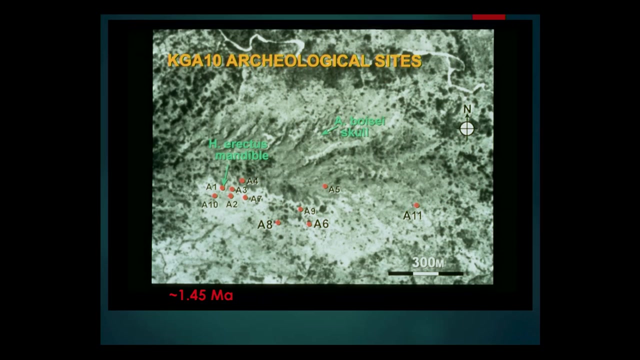 to detach these large flakes in order to make these hand axes. The other most important site that we have in the Konso series: we have about 21 sites in Konso, 21 localities. Out of the 21 localities, the KJ 810,. 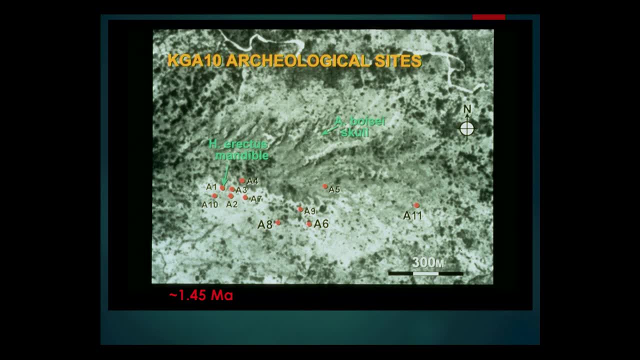 archaeological locality is the most, one of the most important ones. We have about 11,, as you can see, there's 11 locusts, archaeological sites that we excavated, And from this site we also found Homo erectus and Australopithecus boisei. 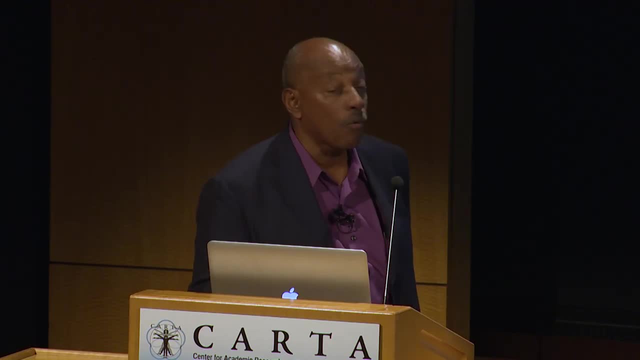 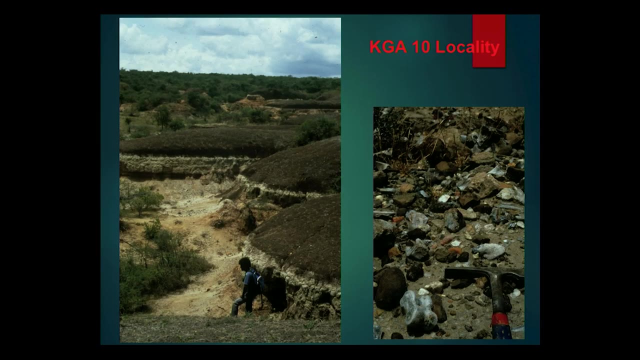 skulls discovered, dated to around 1.45 million years ago, And the Konso Konso, Konso, Gordulla, KJ 810 locality looks like this: This is the first picture that was taken of this site in 1991.. 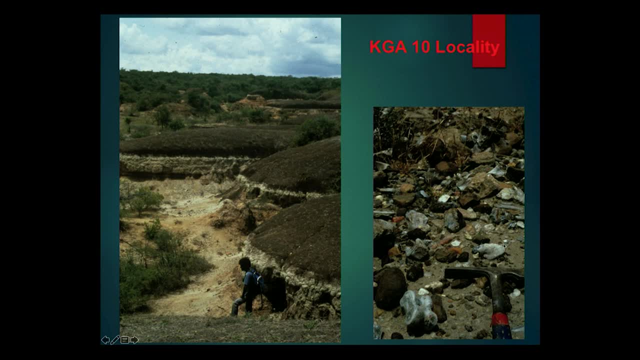 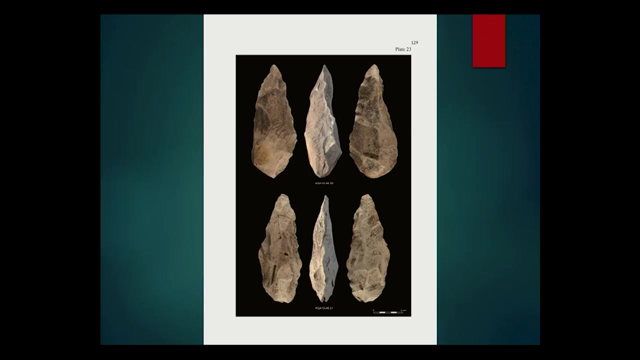 And on the right side you see how the fossils and the artifacts were eroding out of the sediments when we first arrived there. The KJ 810 archaeology shows Acheulean hand axes which are better shaped compared to the former ones. 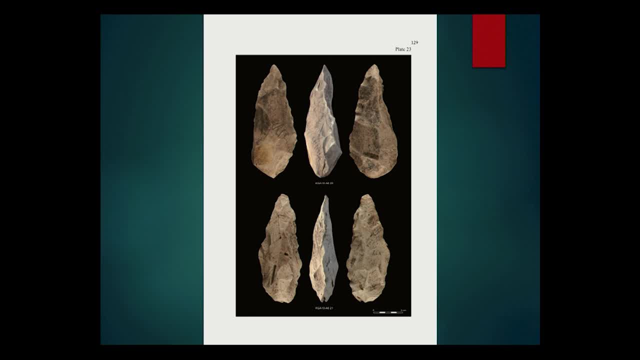 Here you see a crude form of lanceolate, kind of crude hand axes, But we see bifacial shaping, contrary to what we saw into the mostly unifacial shaping, And we see the edge regularization also coming into focus And in general, 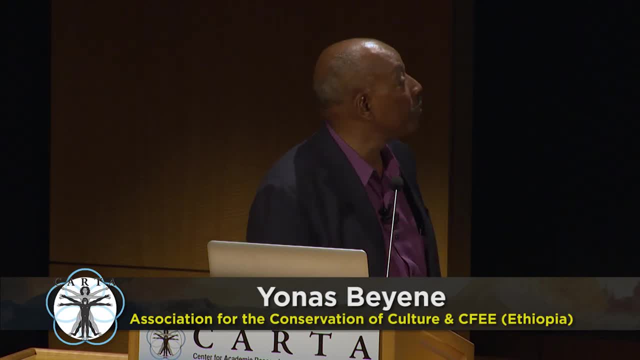 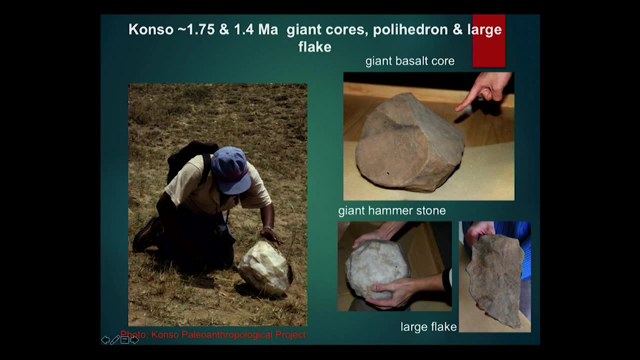 from the 1.75 million years to 1.74 million years ago. from the 1.75 million years to 1.74 million years. we see the oldest site here at KJ 6A1, big boulder. 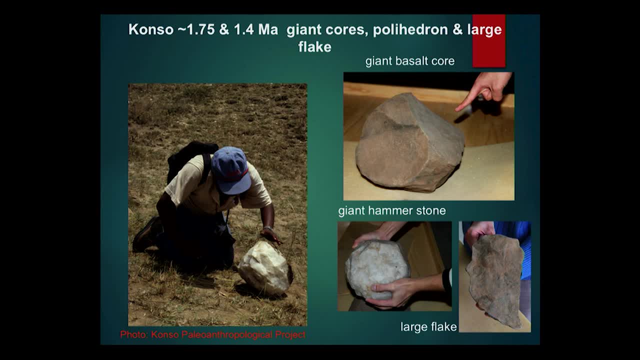 big boulder which was used as a core, from which large flakes, as you can see, were detached and shaped, And by KJ 4 time at around 1.4,. we continue to see large boulders which were used as cores. 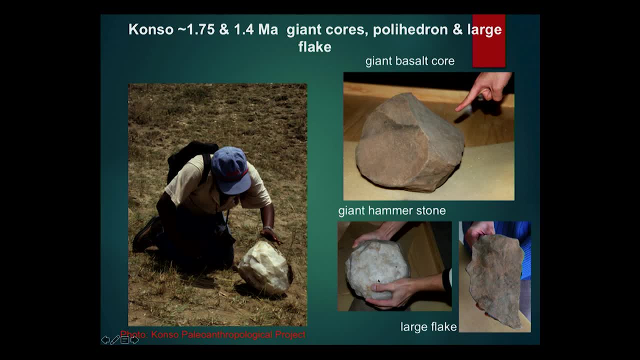 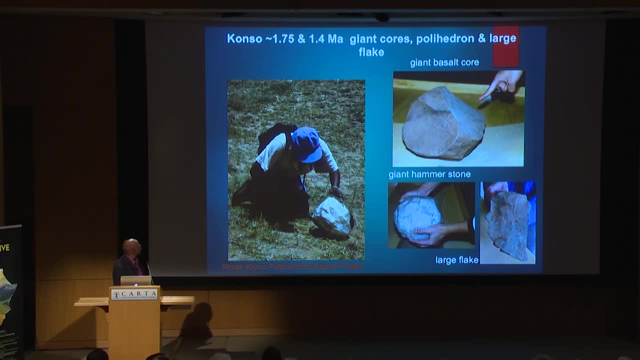 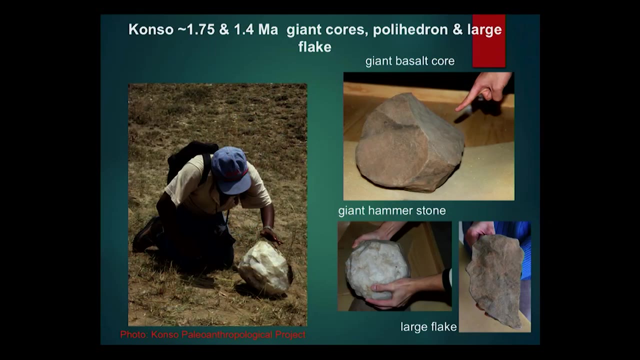 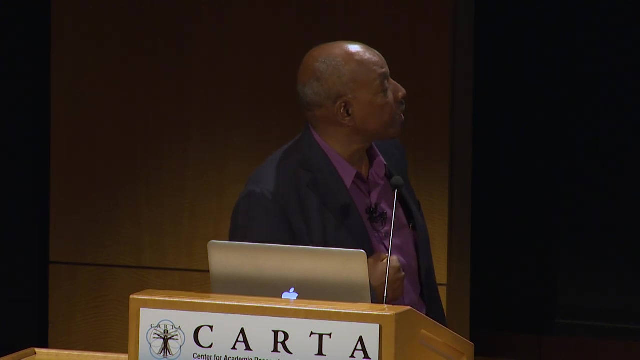 with large giant hammers that were used to detach large flakes. So the 1.75 to 1.4 million years Acheulean in Konso can be summarized as such When we come to the younger age. 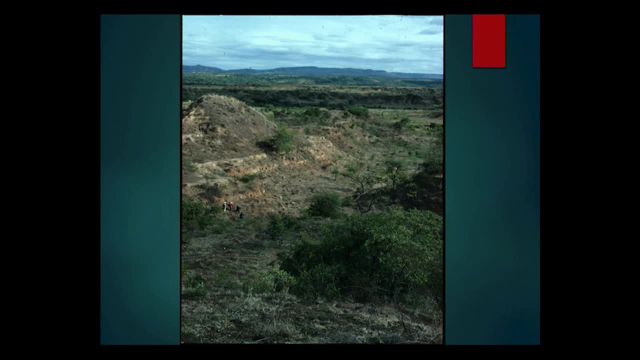 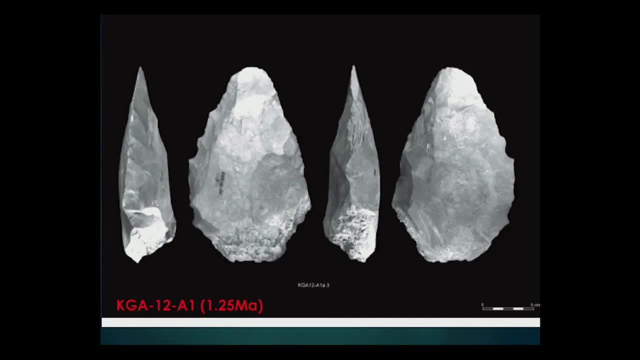 And you see multiple layers of tufts out there which are calibrated with tufts that are found in the in the Kobyfora formation further south in the Turkana Basin And from this KJ 12A1 site by around 1.25 million years ago. 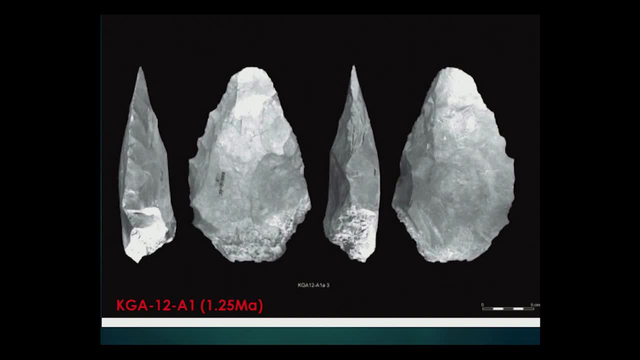 we have better shaped hand axes. we have better shaped hand axes. The reduction is well done. The flaxum200 bucket cost bill is $50 plus The flexant count of the Madeleine envelope from Koreais is $100,000.. 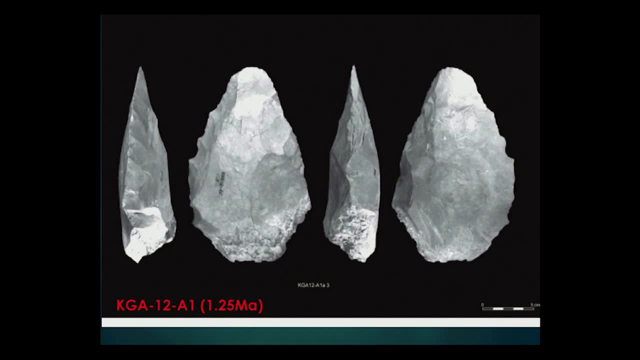 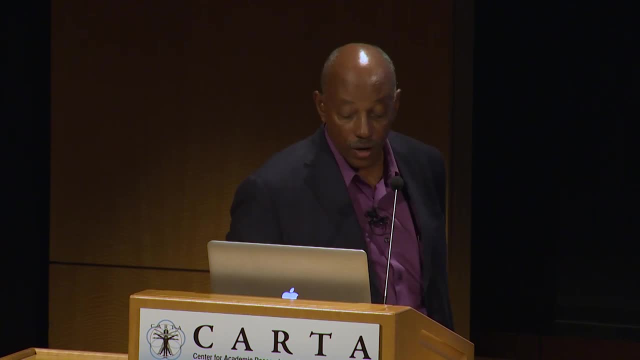 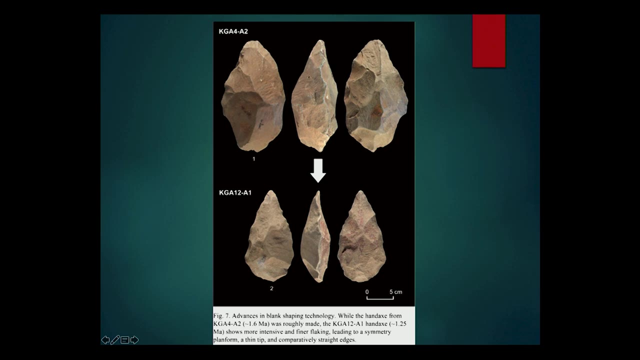 age is better regularized and the planform symmetry is almost attained. And when we compare the KGA-12A1 artifacts, hand axes, which we have here down, compared to the KGA-4A2, the 1.6 million years old, 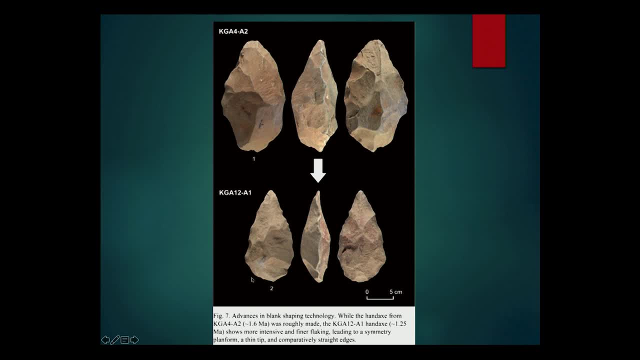 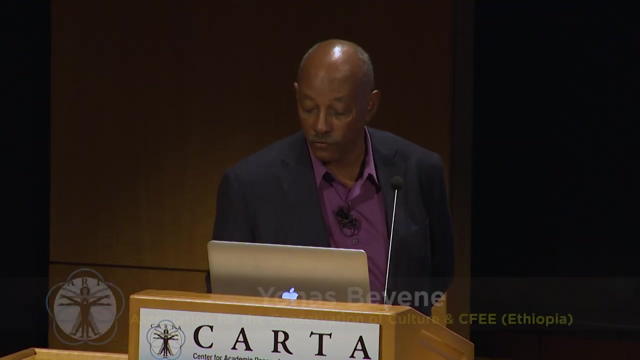 hand axes. we see better planform symmetry here in contrast with this one. The edge regularization is better and the planform symmetry and the scar counts and the invasiveness of the flexed scars is very special, And not only that: around the same time 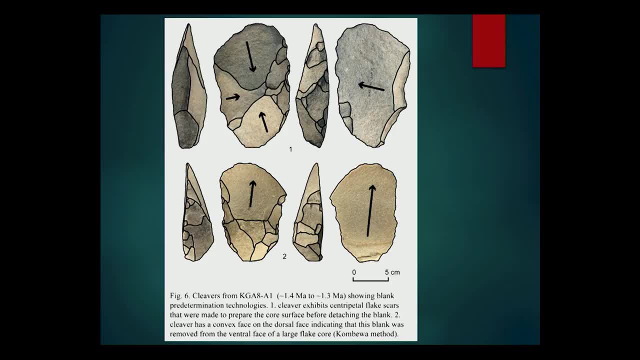 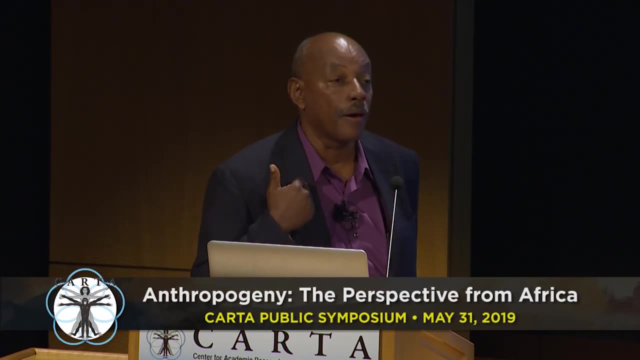 at a site called KGA-8A1, between 1.4 and 1.3 million years ago. we see predetermination of the flex that they were going to detach. The hominids knew what kind of flex they were going to detach from the core. 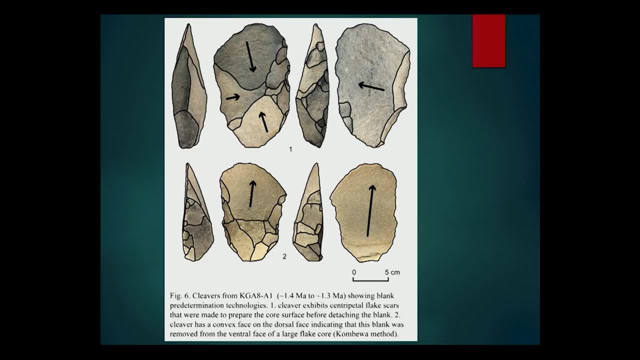 from the mega core that they had. So we see here the predeterminations. the guys, those hominids, had the mental template of the flex that they detached. This in the upper section you see the rods, the arrows, which shows that the preparation of 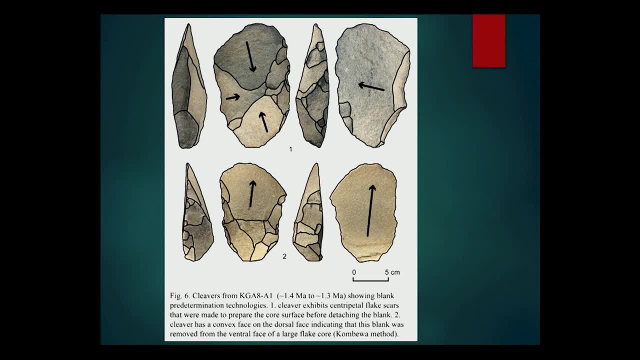 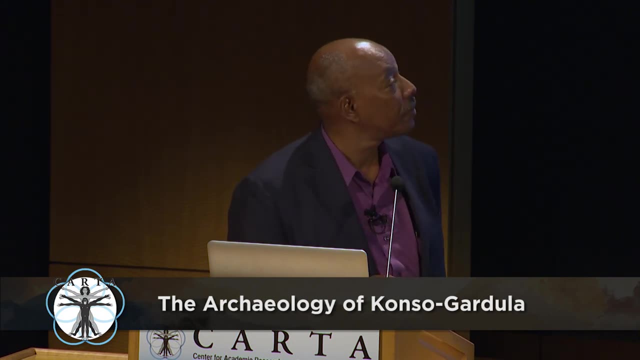 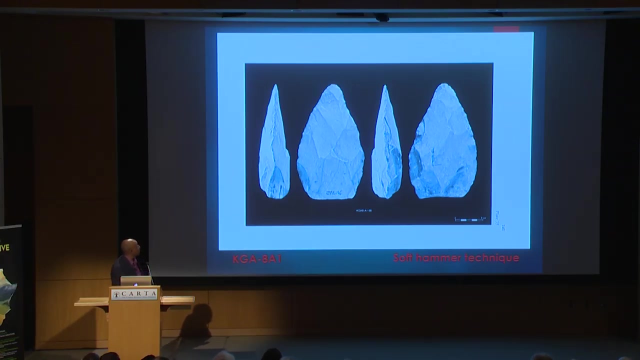 which shows the preparation of the core before the last detachment of the flake at the end. So we see a technique that is commonly known as zakamboa in that area. Not only that, we also think that from the techniques that are applied on this handaxe, on this biface, 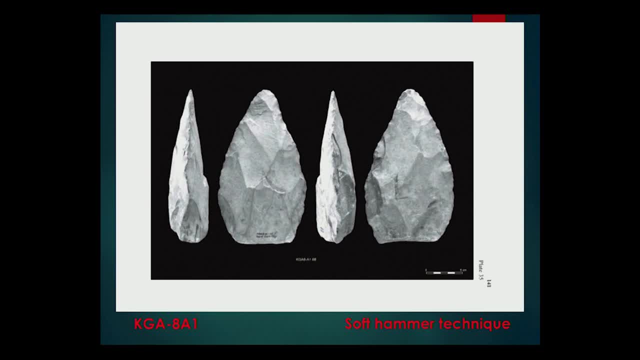 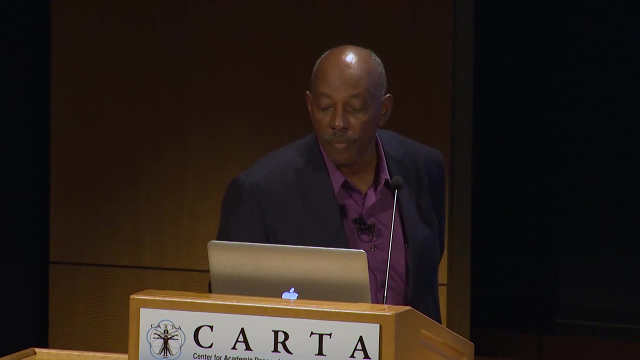 by 1.3 million years ago- we are- we can permit ourselves things- that perhaps soft hammer techniques, shaping using soft hammer techniques in order to make better, regular, better shaped, almost three-dimensionally symmetric stone tools was attained, It was evident by 800,000 years ago. 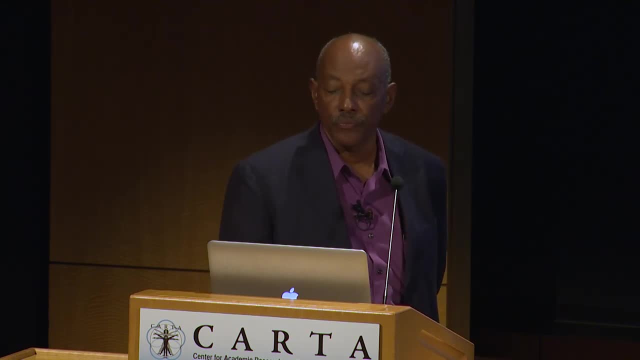 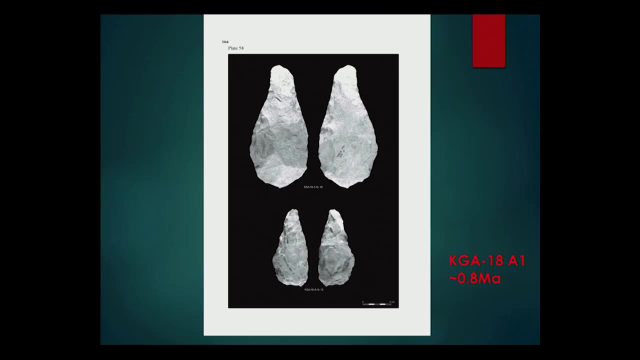 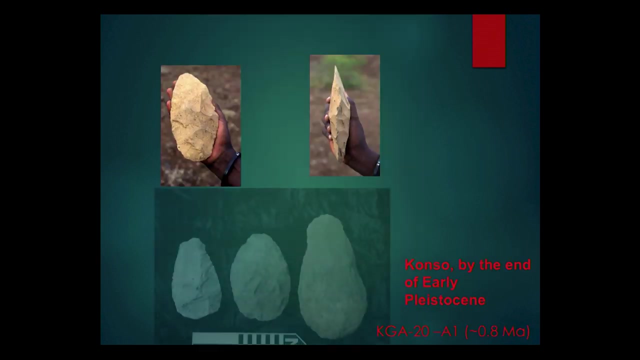 at another site that we call KJ 18 A1.. We see better refinement and the choice of raw materials. Rocks is more diverse. They went for more fine-grained rocks and the 3D symmetry as you can see it here. 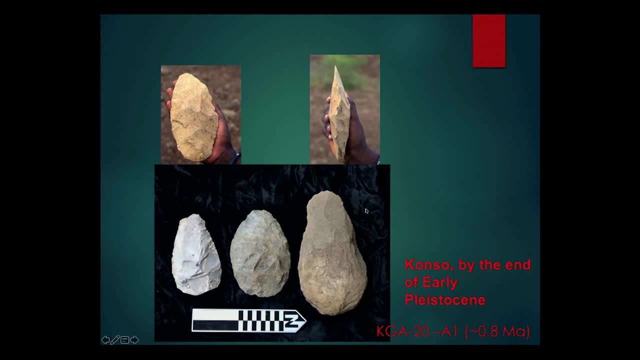 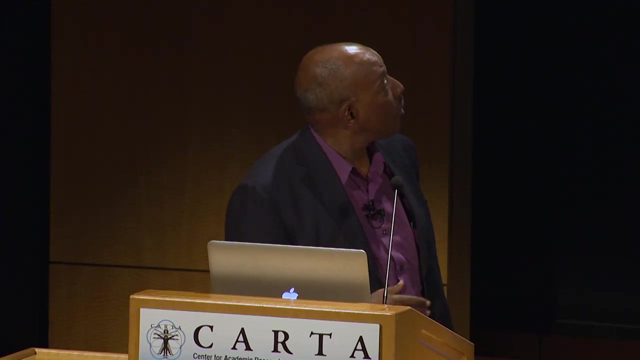 is attained and large, bigger and well-regular kind of handaxes were also made and the edge and the regularization it was attained. So the Acheulean industry, the technique of making handaxes, which is started by around 1.75 million years ago in Konso. 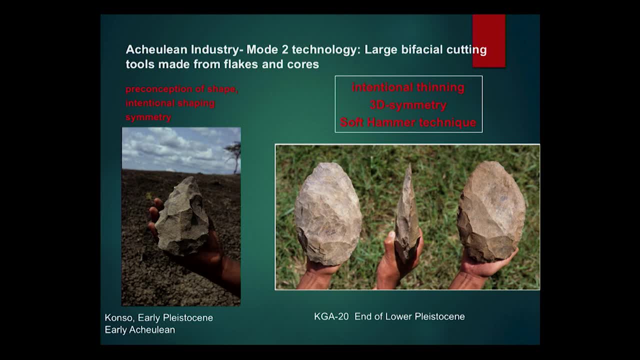 By the way, this is one of the oldest in the world, together with the ones that we have in east, in west Turkana. From the preconception of shape, as you can see here on the left, an intentional shaping. 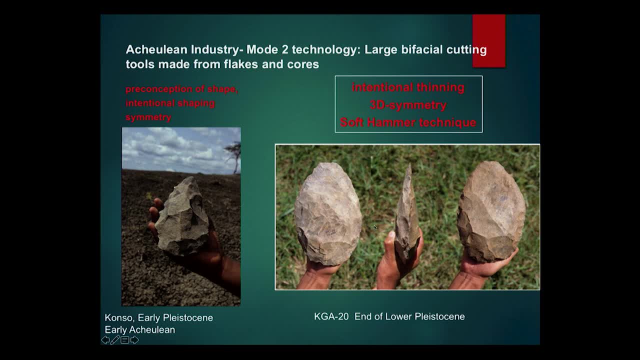 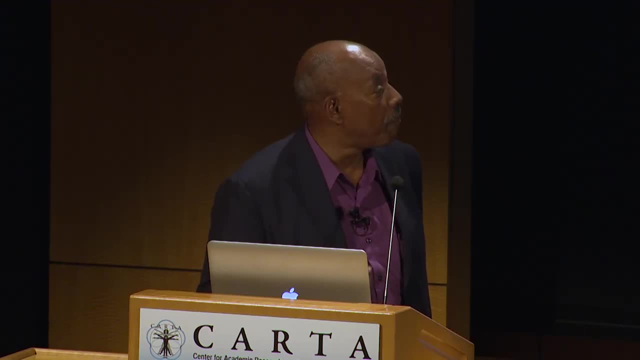 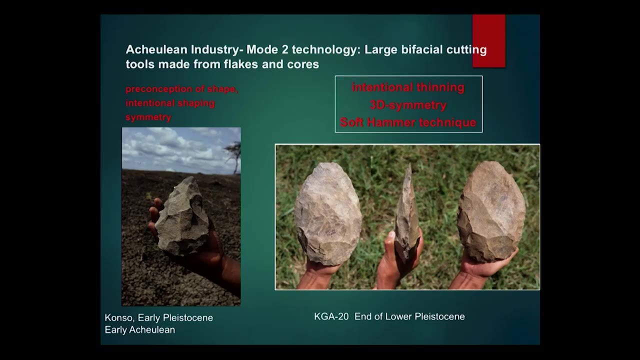 then, by the end of the lower Pleistocene, by around 800,000 years, hominids were able to shape better refined handaxes using soft hammer. invasive flex cars were there and you can see the platform, symmetry and the section which together makes 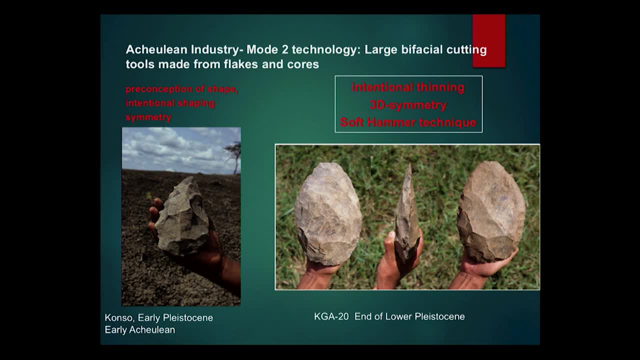 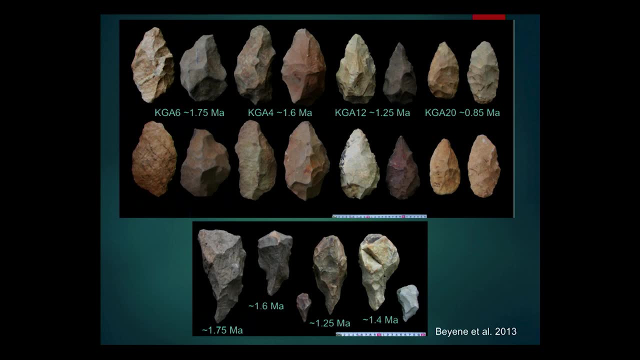 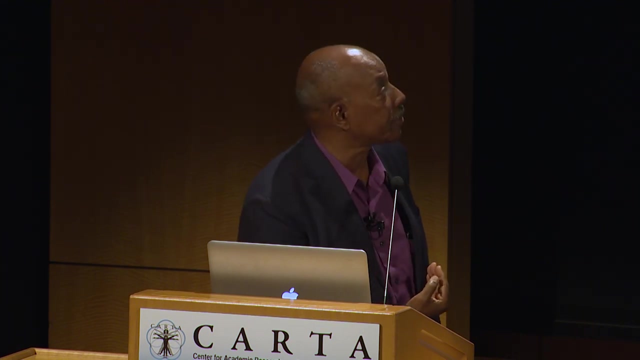 the 3D symmetric handaxes. So, in summary, what we have in Kosovo, from 1.75 million years ago all the way to 850,000 years ago, is a continuous progressive change of the technology. The handaxes it does not mean. 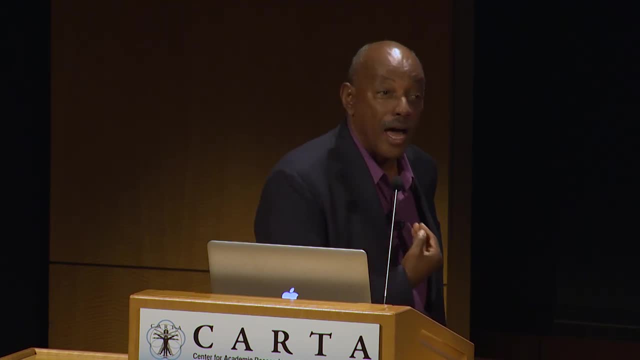 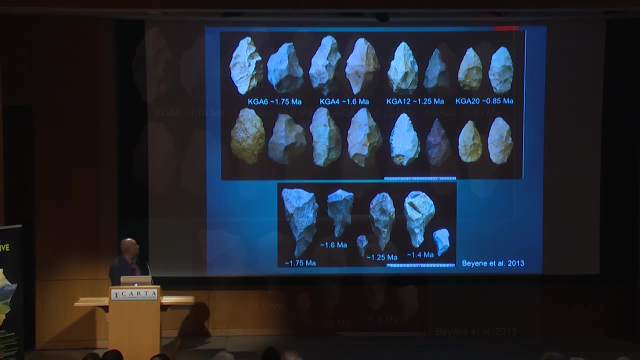 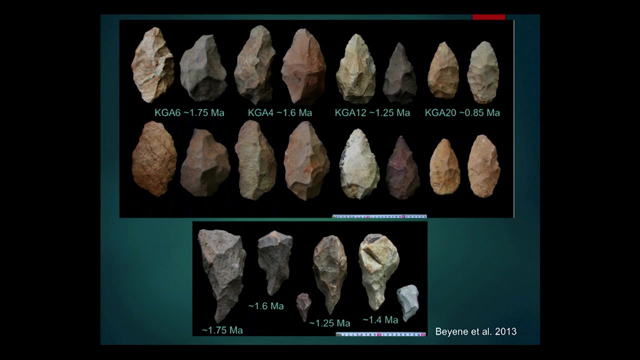 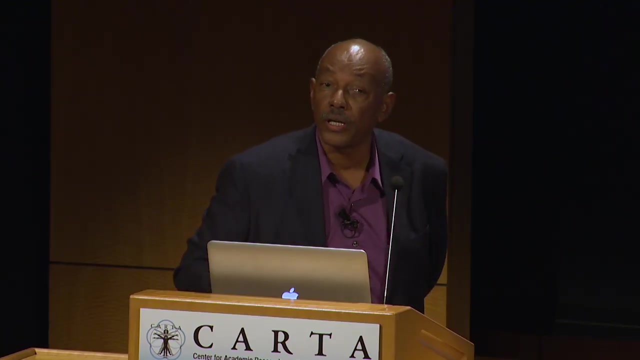 that there are less better made handaxes, but these are representatives indicative of the trend And, as you can see below, the peak forms continue the same, but the trend with the handaxes is well demonstrated. Kosovo is not only about lithic materials. 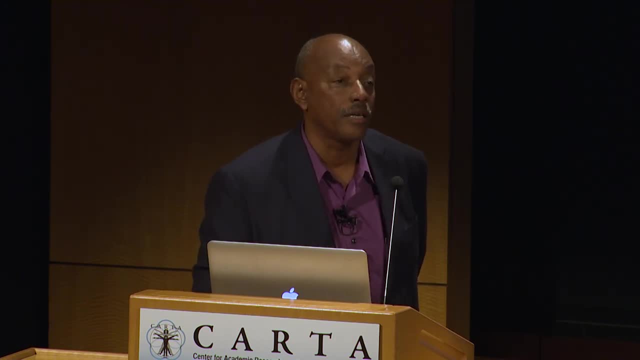 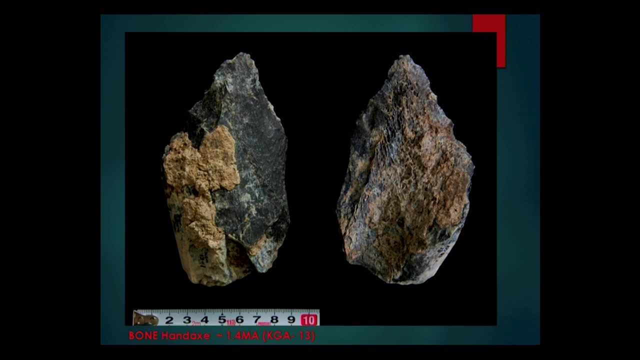 Kosovo is not only about lithic materials. Kosovo is not only about lithic materials. it's not about making only stone tools, not only making handaxes from rocks. They were also knapping bones from large mammoths At one point, four million years ago. 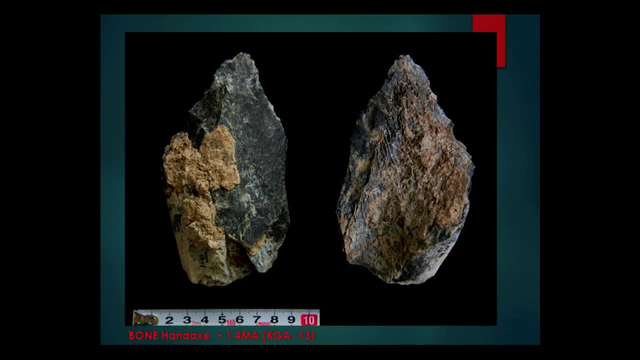 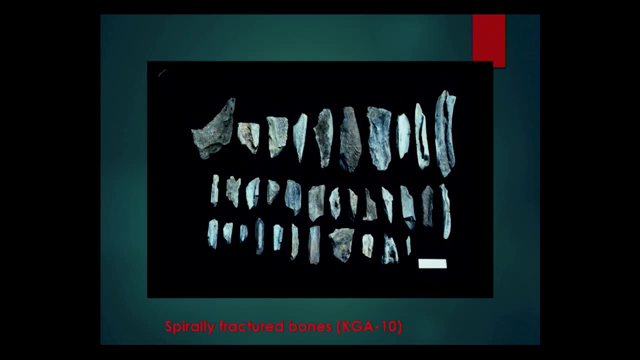 we have a handaxe made on bones, bones which were modified, maybe for digging spirally fractured bones to extract marrow, possibly from the bones, marrow possibly from the bones, And we also have hominids discovered in this site. 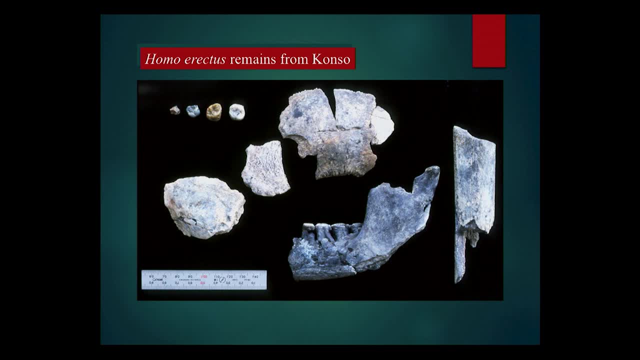 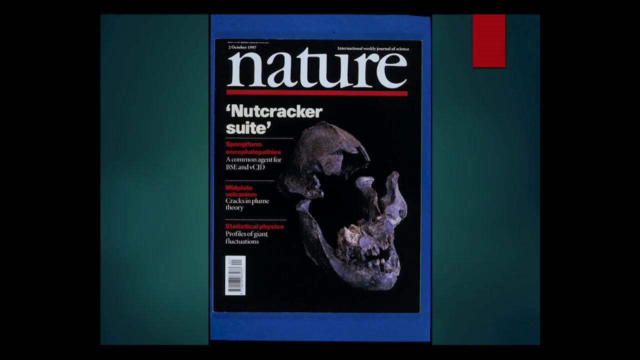 And we also have hominids discovered in this site, Here represented by this mandible. this cranial frags is a homo erectus, and there is also one post-cranial out there And the best-known Kosovo specimen, Australopithecus boisei, which made it to Nature's cover page. 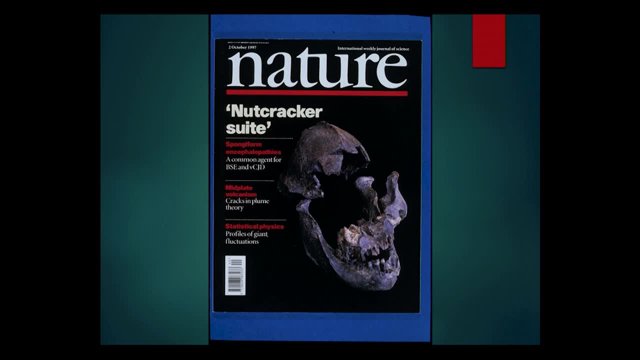 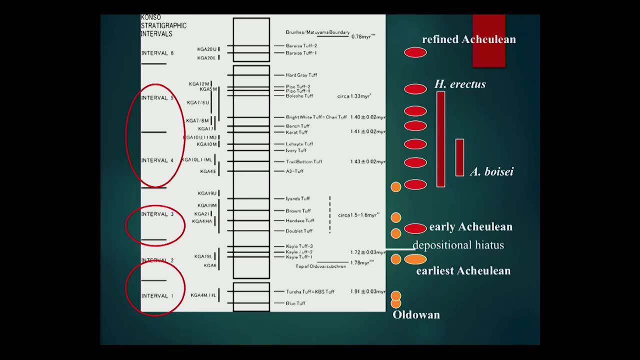 Australopithecus boisei, which made it to Nature's cover page, is represented here. So in general we can see an evolution from the older one to the earliest Acheulean, early Acheulean, then after 1.45,. 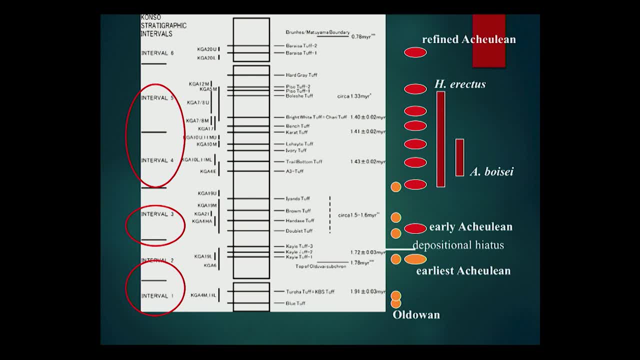 we have the boisei and the homo erectus going together and with more Acheulean sites after the 1.4 million years and with more Acheulean sites after the 1.4 million years and with more Acheulean sites after the 1.4 million years. 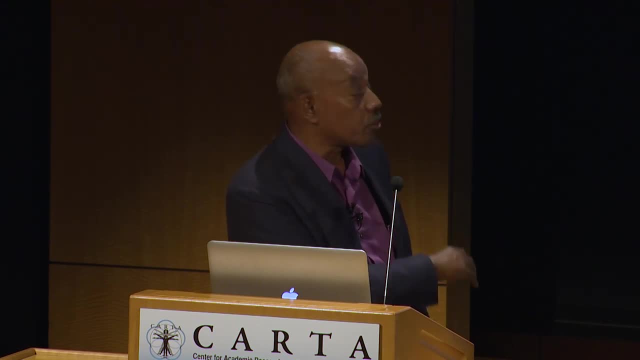 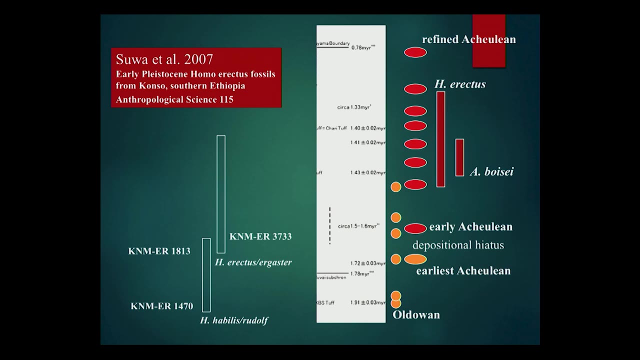 And when we compare Kosovo with what we have in India, And when we compare Kosovo with what we have in India- East Turkana, we can say that the earliest Acheulean in Kosovo began together with the appearance of perhaps the oldest homo erectus. 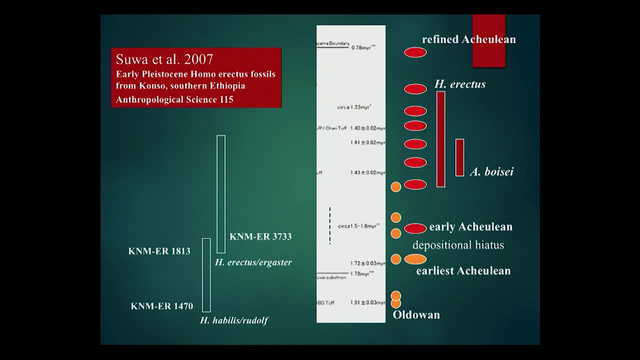 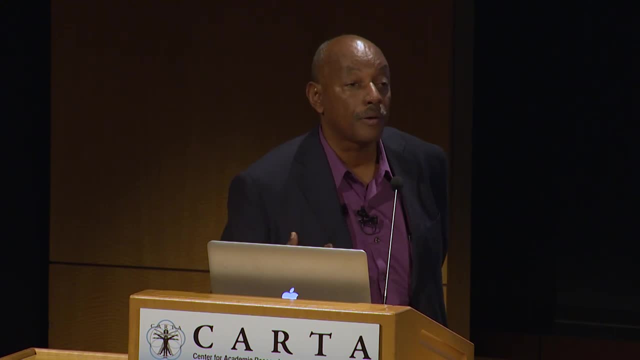 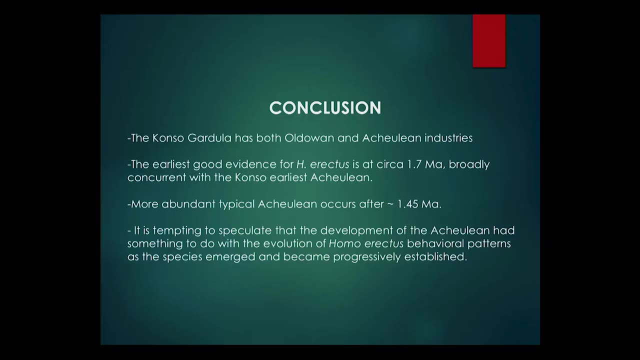 And as homo erectus was established, the Acheulean was more developed and took over and you can even start finding it everywhere in many cities. And you can even start finding it everywhere in many cities In the Middle East, Beria, in several sites in East Africa. 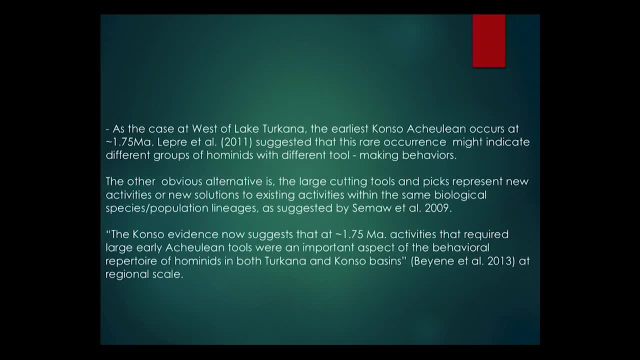 In the Middle East, Beria, in several sites in East Africa and elsewhere, So as in the case of west of Lake Turkana. So as in the case of west of Lake Turkana, the earliest Kosovo Acheulean occurs at 1.75,. 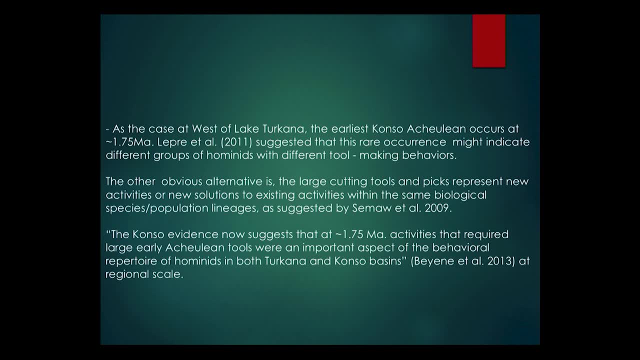 and several people have hypothesized why the Acheulean industry happened in the first place, why the Acheulean industry happened in the first place, whether it was a phenomenon, that was, that appeared in with the earlier, with older hominids. 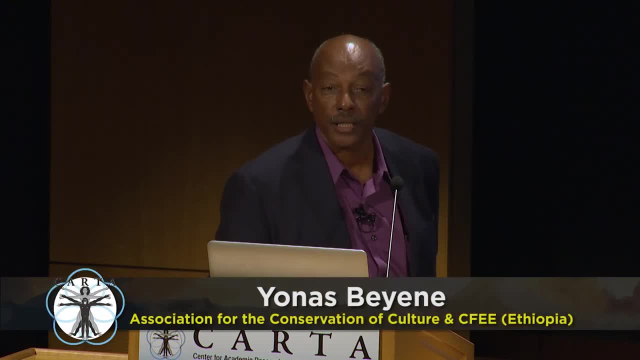 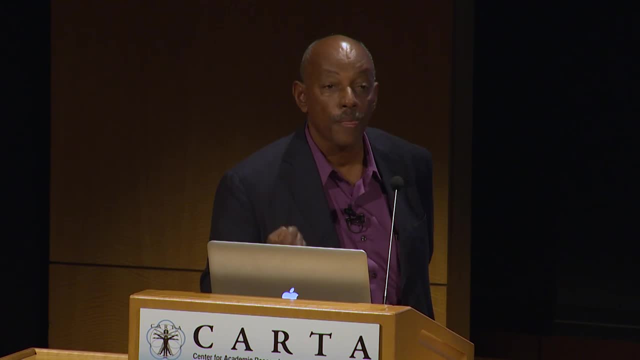 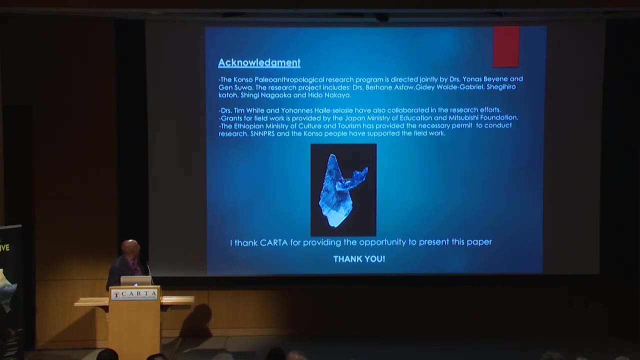 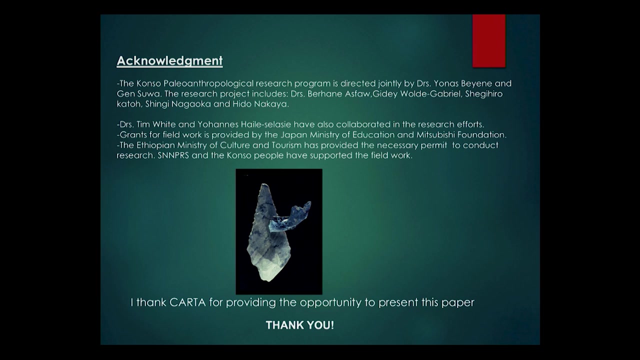 or with homo erectus, as homo erectus started to include more activities to exploit its landscapes. I would like to thank the Kosovo Paleoanthropological Research Projects, which I call lead with my colleague Professor Gen Suwa, and Brani Asfaw, was instrumental. 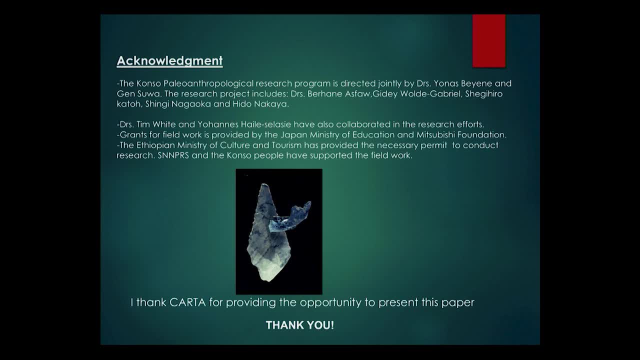 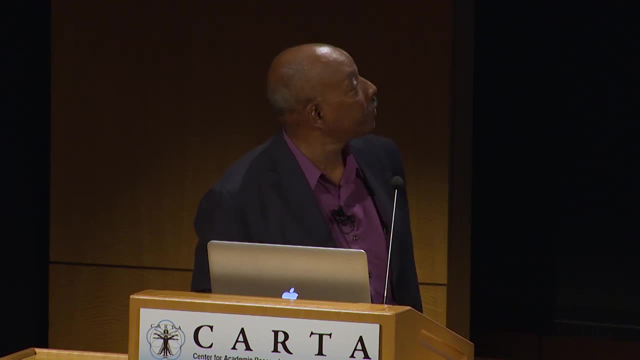 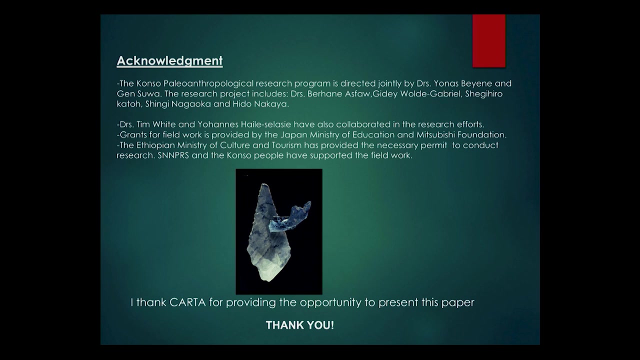 and it was his project which first discovered the site and he handed it over to me and Gen to work on it and he continued participating. And Tim White, Gidei, Waldo-Gabriel, Shigeru Kato, Shinji Nagaoka Hido Nakaya, our Japanese. 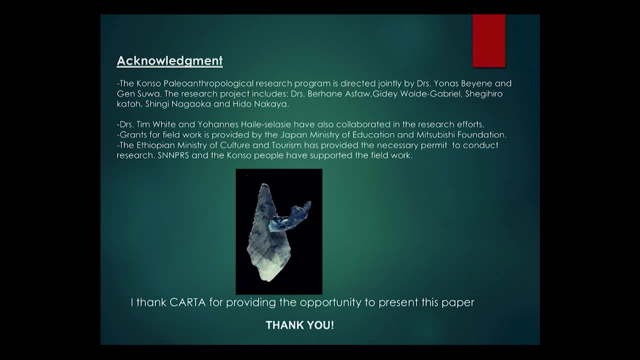 Shigeru Kato Shinji Nagaoka Hido Nakaya. our Japanese and other Japanese colleagues collaborate in this research And other Ethiopian colleagues also collaborated in this research and grant was provided by the Japan Ministry of Education in Mitsubishi Foundations. 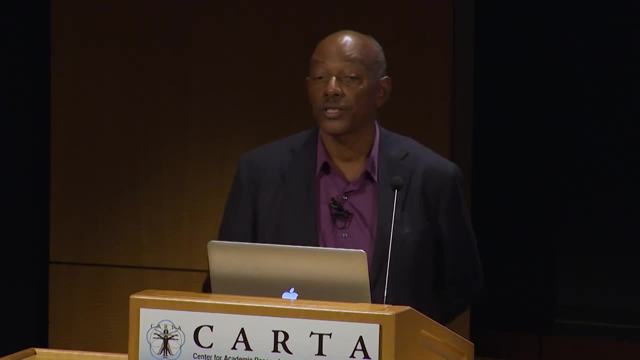 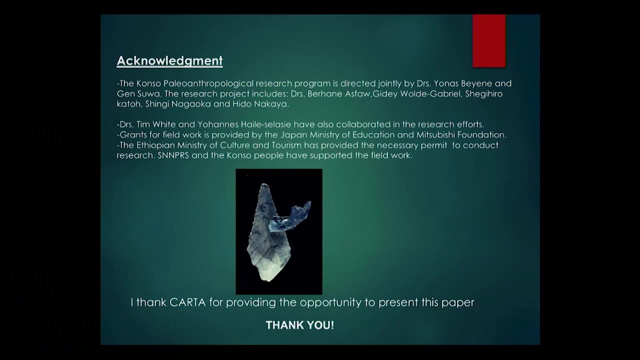 and the Ethiopian Ministry of Culture and Tourism and ARCCH and the Konso community and the Southern Ethiopian region's government have helped us in all our endeavor to do the field and laboratory research through research. I thank again CARTA for providing me this opportunity.